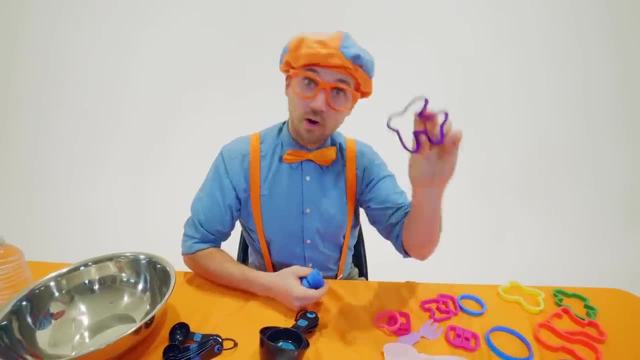 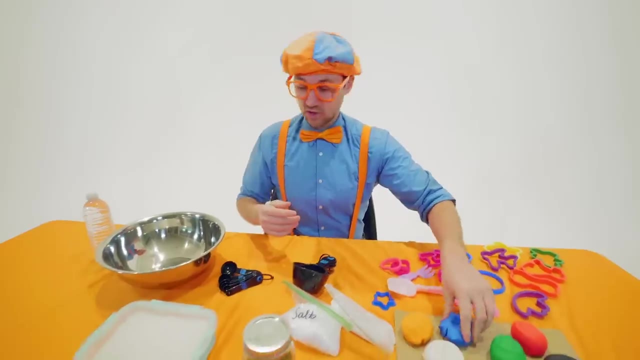 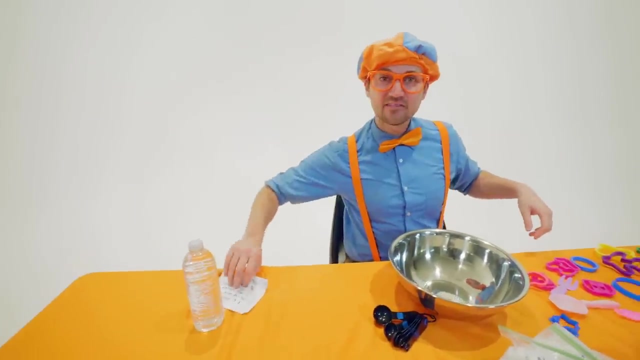 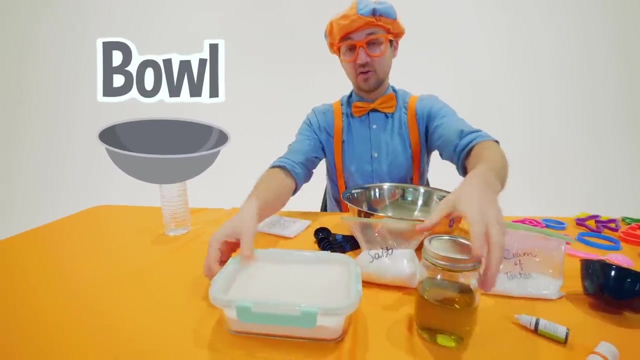 we can spell some words together. Maybe we can make an airplane together. This is gonna be so much fun, Okay. so the first thing we have to do is have all the ingredients for this clay. Yeah, here we go, And I have my recipe right here. First, we need a bowl. And what I would do if I was you. 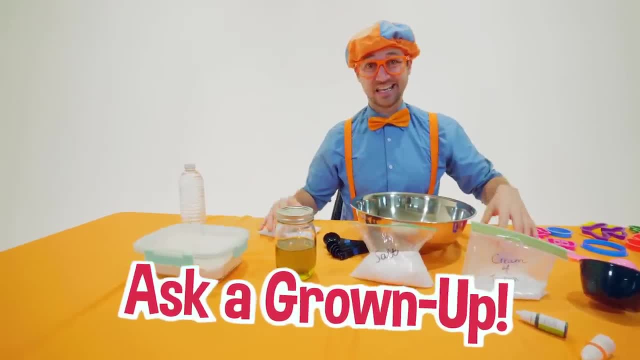 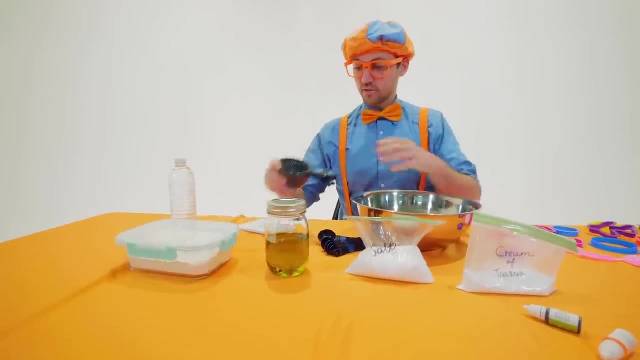 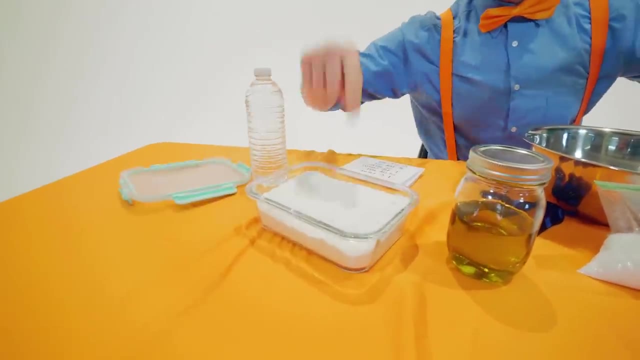 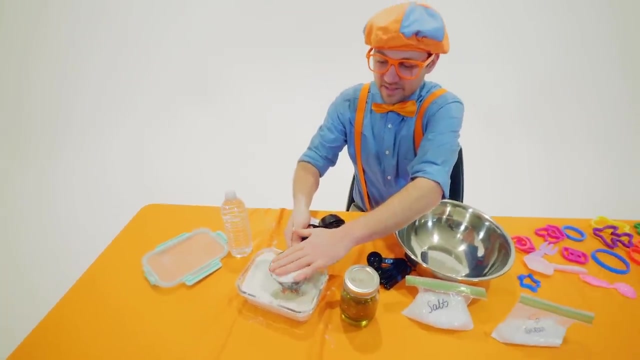 I would probably have a grown-up help you, because this can get really messy And there's a lot of ingredients. Yeah, all right. So first we need to start with one cup of flour. Okay, let's open this up. There we go, And it doesn't need to be exact. Yeah, that is one cup of flour. 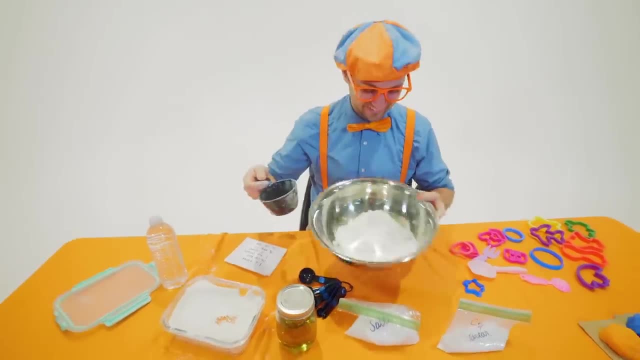 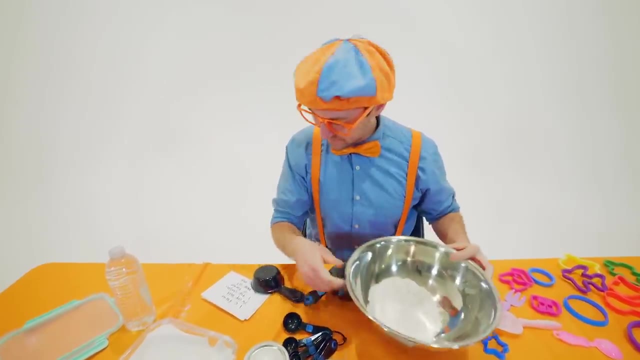 Here we go, And I have my recipe right here, And I have my recipe right here, And I have my. Here we go. Wow, That is a great base for the clay we're making. Okay, all right, Let's see One. 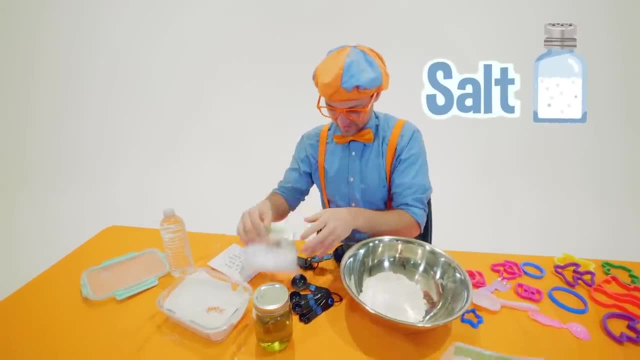 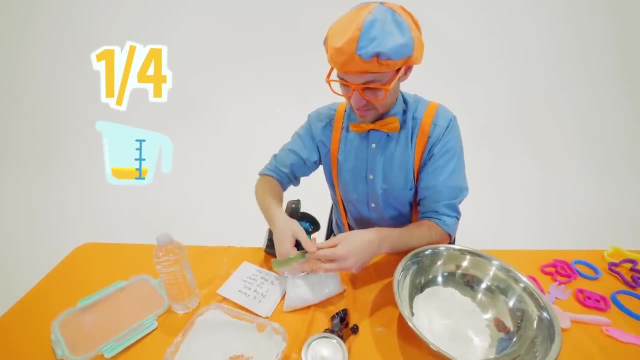 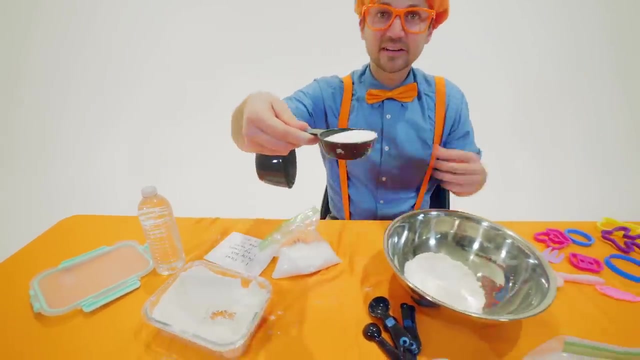 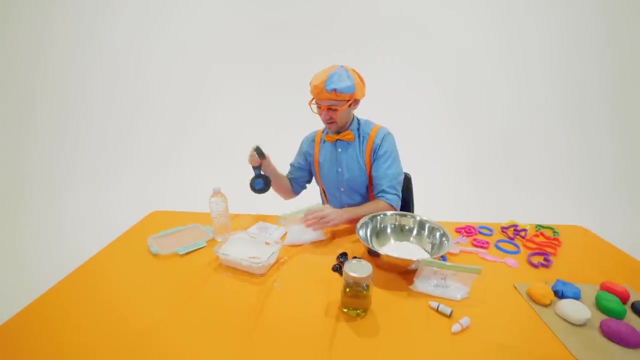 quarter cup of salt. All right, It is definitely already getting really messy. Okay, one quarter cup, And then we need to grab some salt. Here we go, Here we go, Perfect, Ready Three, two, one, Whoa, Perfect, All right. Okay, let me zip this. 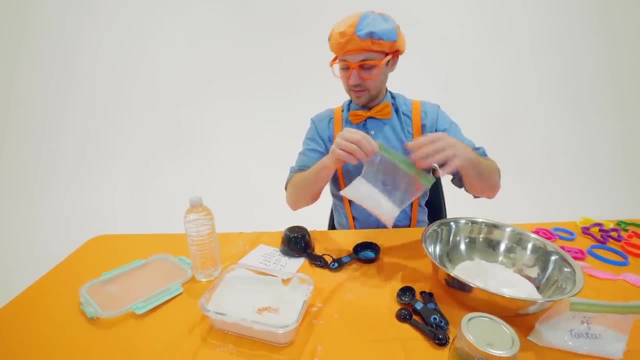 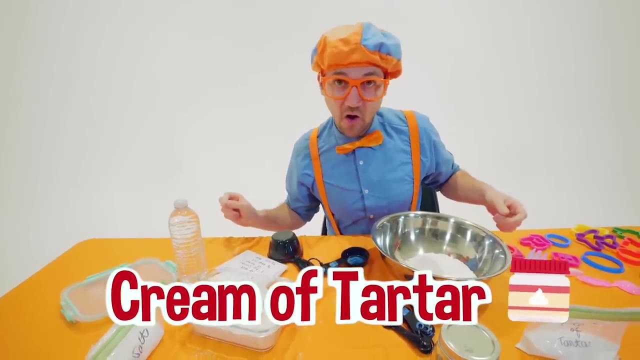 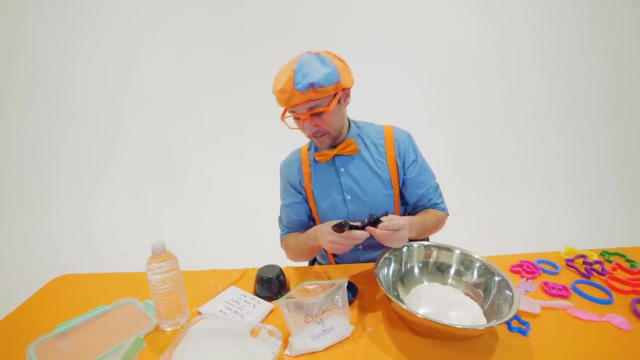 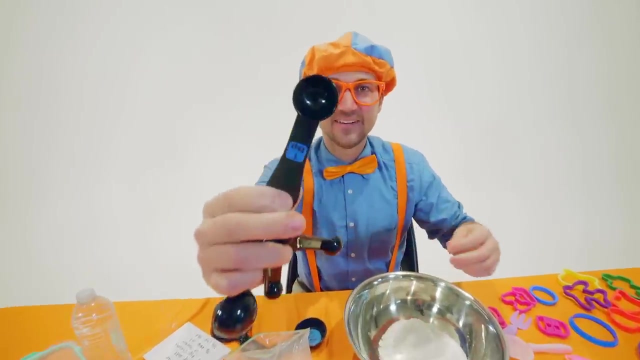 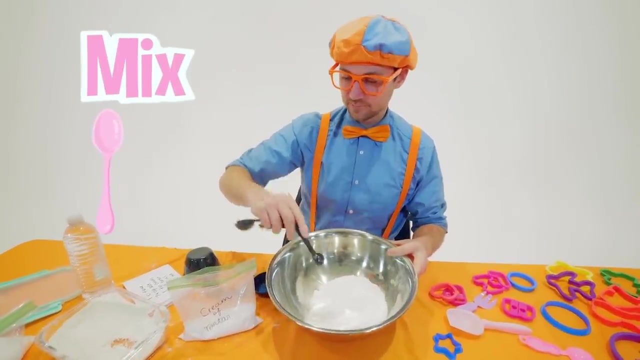 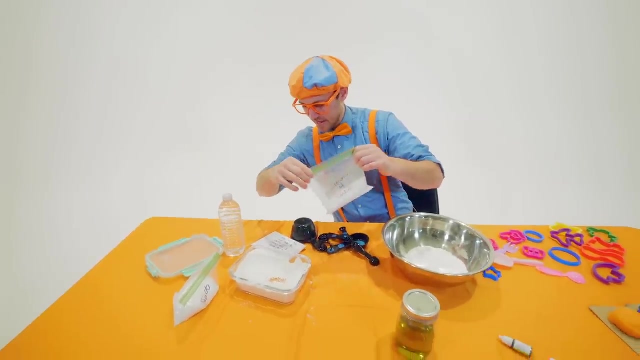 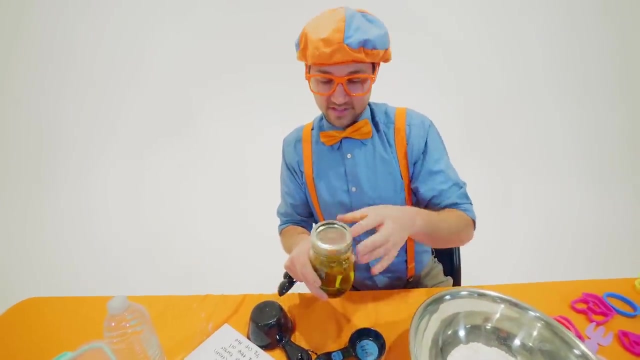 back up. Yeah, Then we need one teaspoon of cream of tartar. What a silly name. That's so fun: Cream of tartar. Cream of tartar. One teaspoon- Oh, there's so many? Okay, here we go. Here's one, Here we go, And we're going to mix all this up in a little bit, But for now, let's pour all the ingredients in here. Then we have a half a tablespoon of oil. Okay, Whoa, This is where. 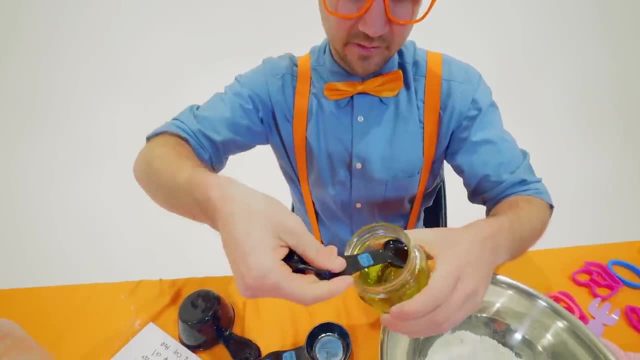 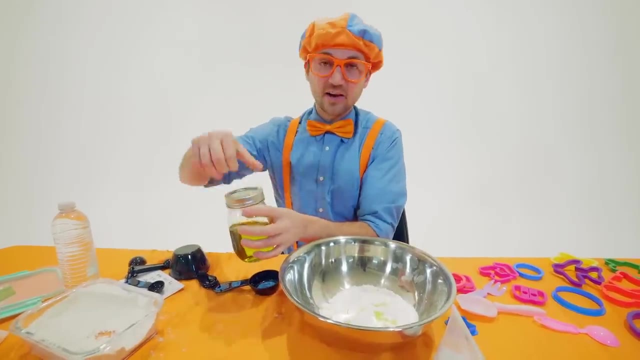 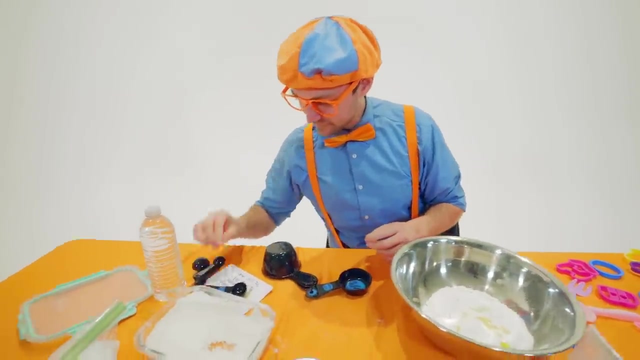 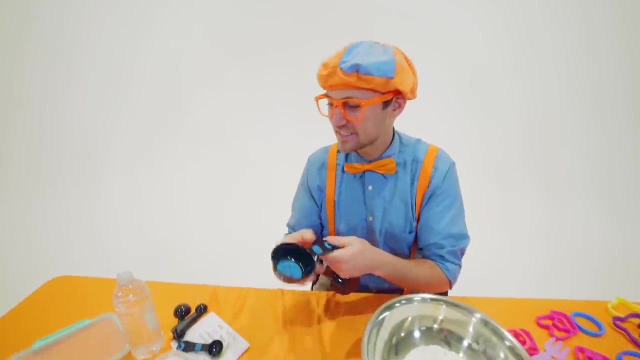 Might get a little messy, Okay, Perfect, All right, Put the lid back on, Just so it does not spill. That would be bad news. berry, Okay. And then we have half a cup of H2O. You know what H2O stands for, Yeah. 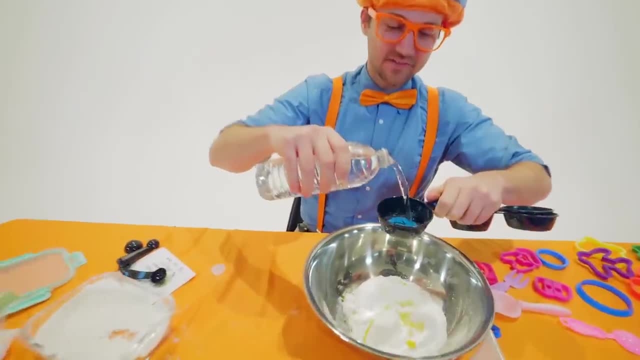 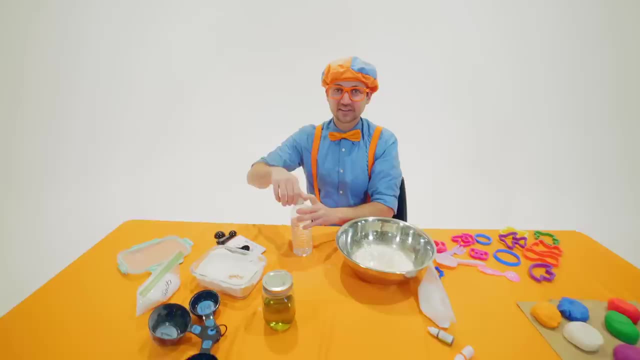 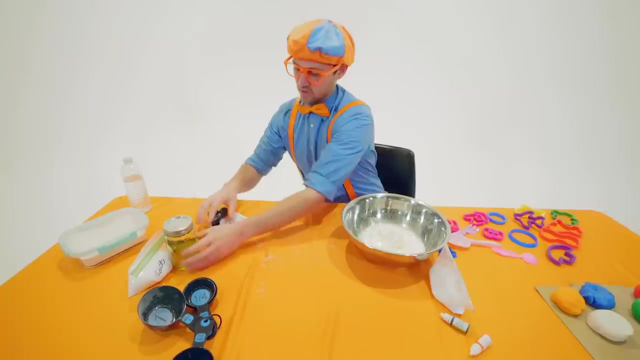 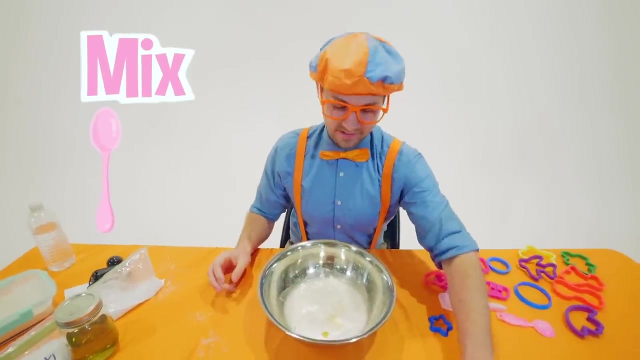 Water. I love water. All right, Half of a cup, Perfect. All right. Oh, hey look, I forgot to close up the flour. You should probably do that. All right, Push all that stuff to the side, because now we're ready to mix it up, But what we need to do is put in some color. You can make any color you want. 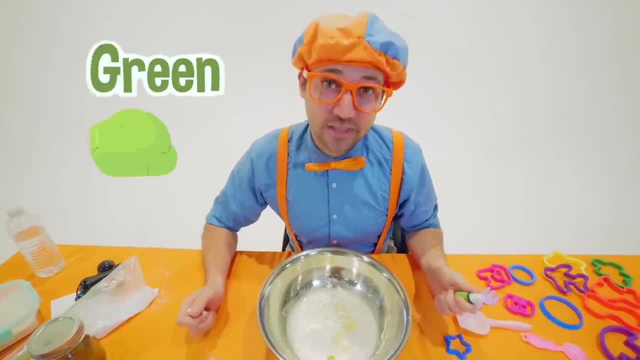 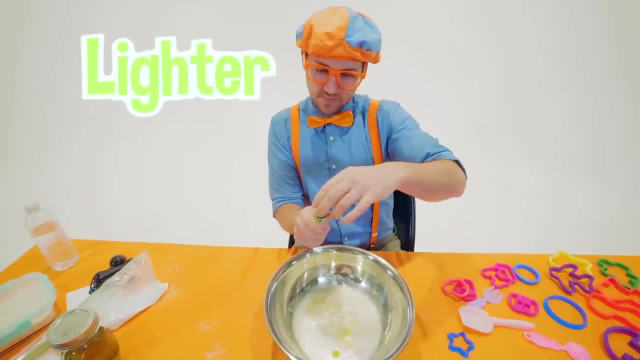 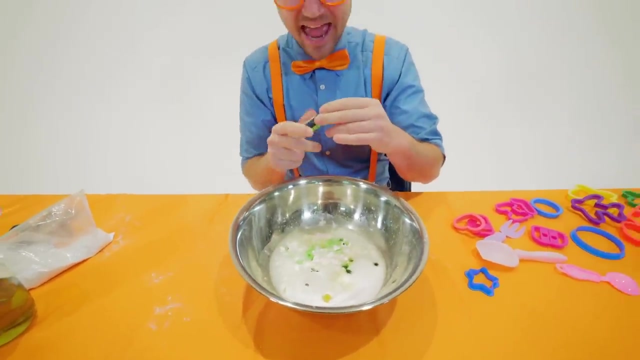 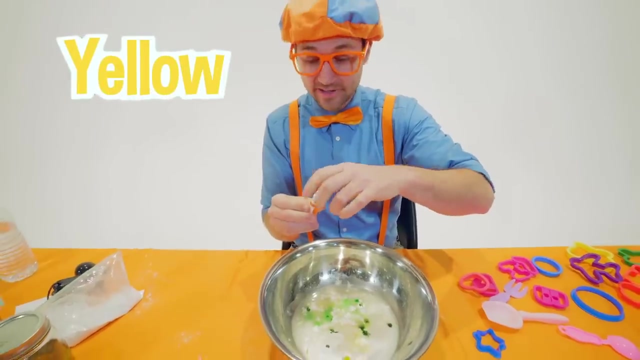 But what we're going to do. although we already have a green color, I think we should make another green, But this one will be a little bit lighter. So let's open this up, Add some green. I don't know how much to add, but that seems like quite a bit. And then also, I'm going to add a little bit of yellow. Yeah, it's going to make it more of a bright green. 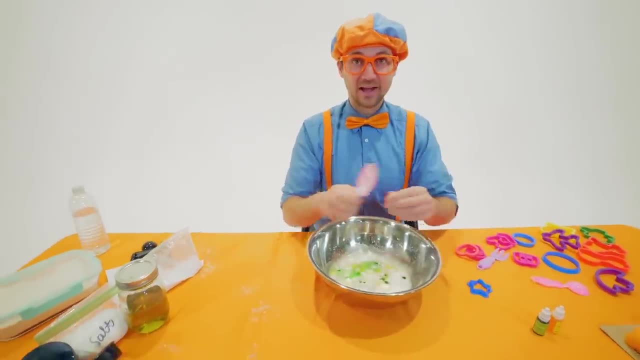 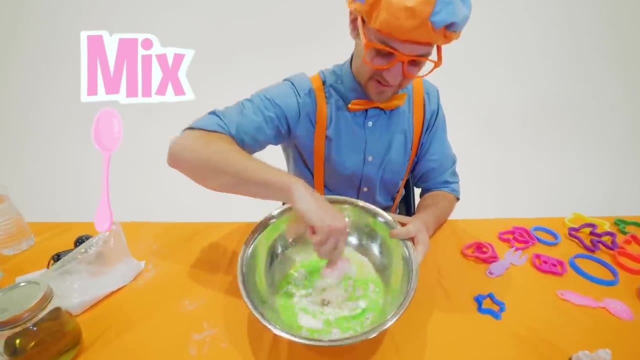 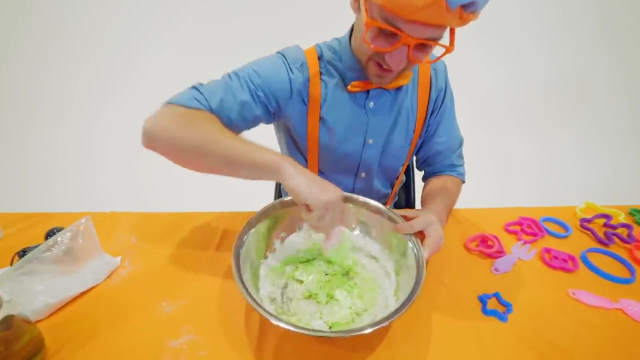 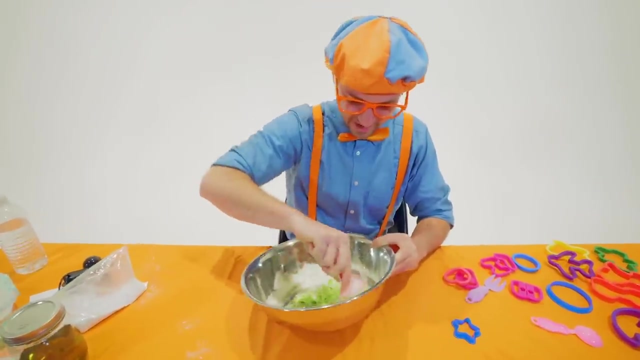 Okay, Let's close that up. Whoa. That was a fun recipe to make, But now I got to mix it up. Whoa- It's looking so good. Wow, You see it. Whoa. All right, Let me keep mixing it up. 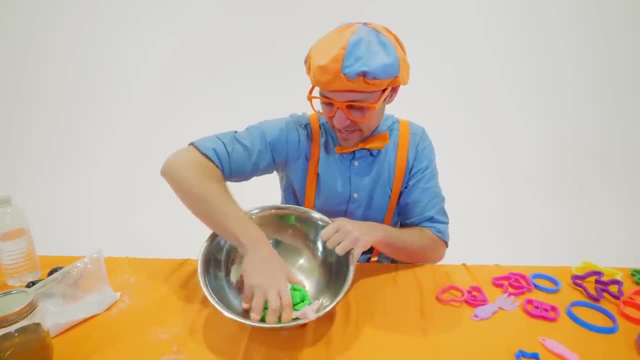 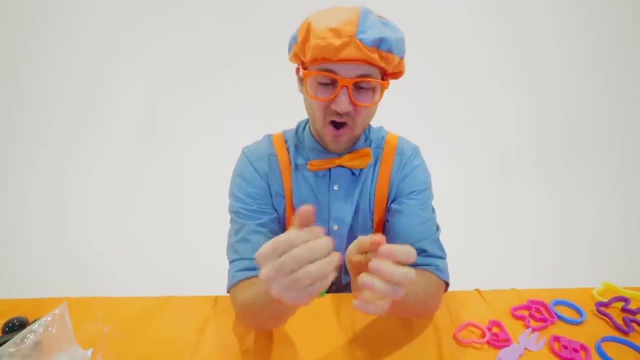 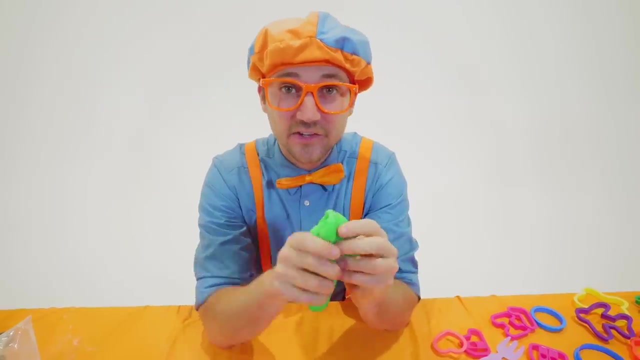 Whoa, Yeah, We did it. Whoa, Check it out. Wow, Whoa, Homemade clay. Wow, What a pretty green color. we made Good job. I wonder what color you're going to make at home for your first color. 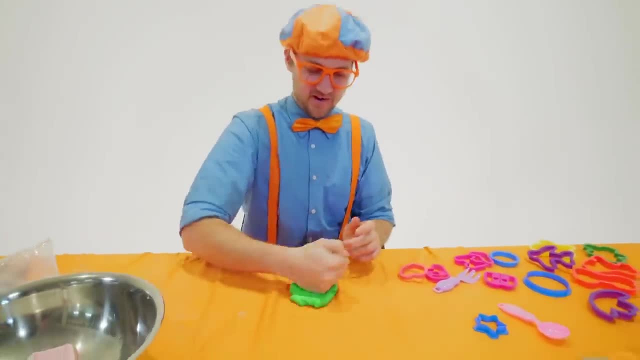 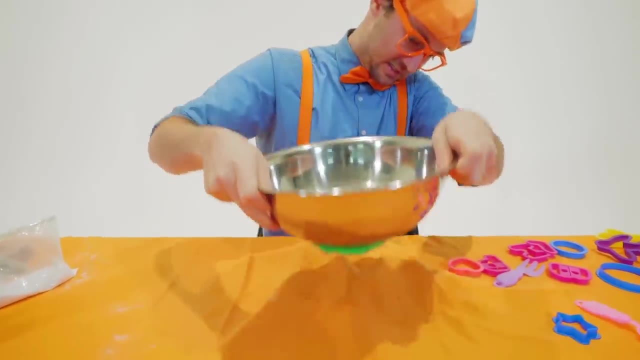 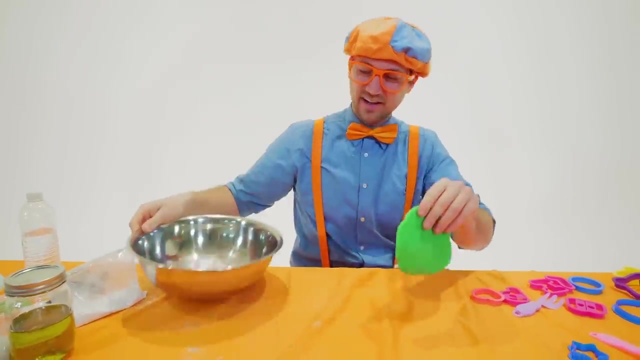 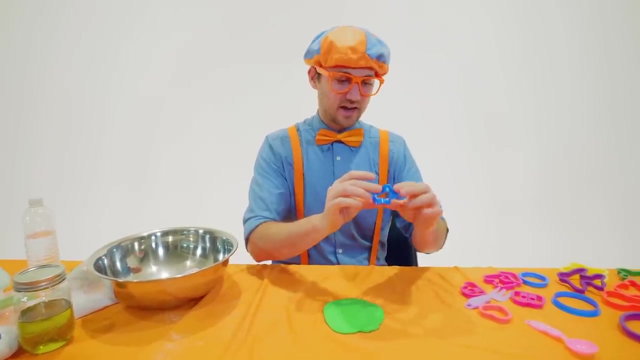 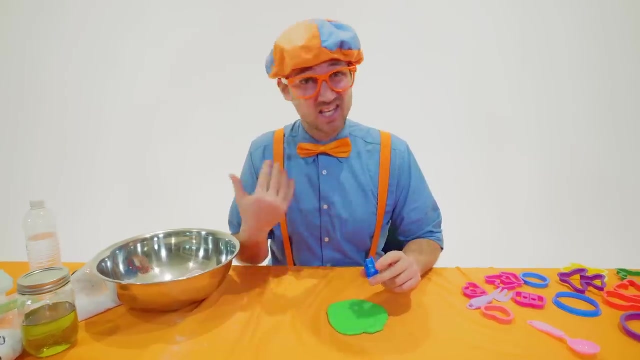 So now what you can do with this. it's so much fun. You can actually smash it flat. Watch this trick. Hmm, Where'd it go? Oh, that's silly. Okay, Let's peel it off. Wow, Perfect. And then now you can use these. Yeah, They're like cookie cutters, but these are definitely not cookies that we're making. I would not eat this. Okay, All right. Okay, Yeah, Remember that airplane. 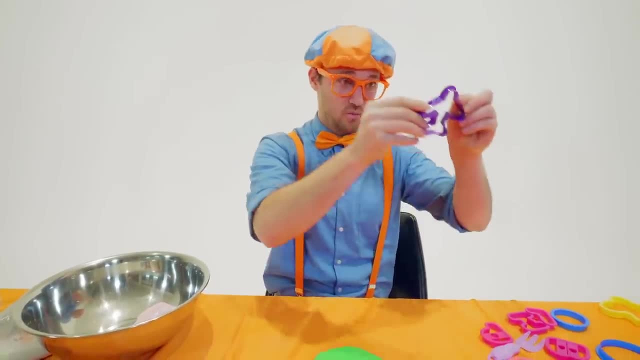 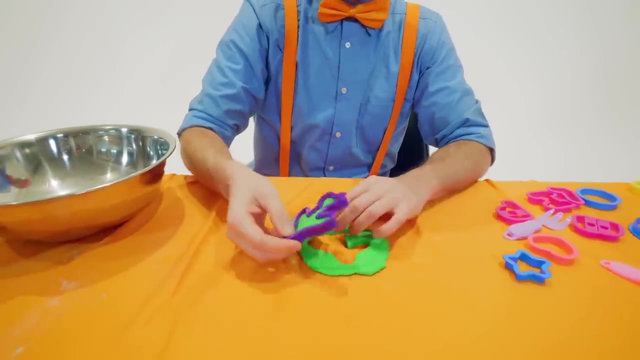 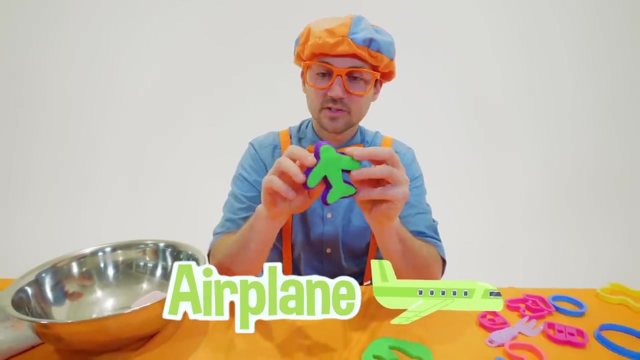 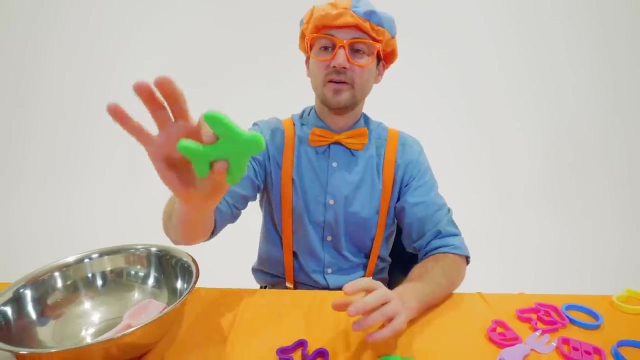 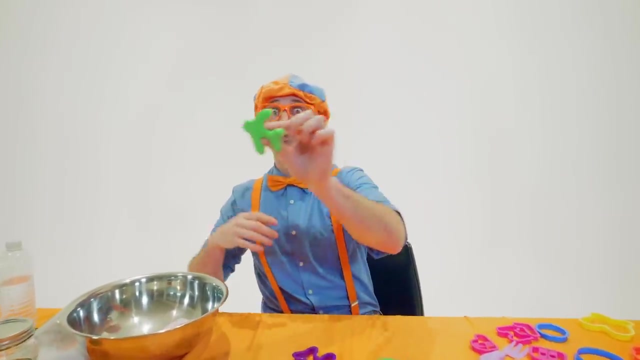 Whoa, Yeah, Check it out. Okay, Now you push it down. Whoa, Look, Cut an airplane out, But first let's push it out of here. Wow, Yeah, We did such a good job. Whoa, whew, wow, okay, I'll put that airplane, right there. 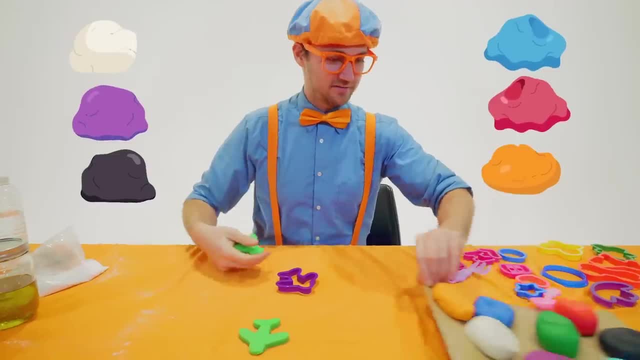 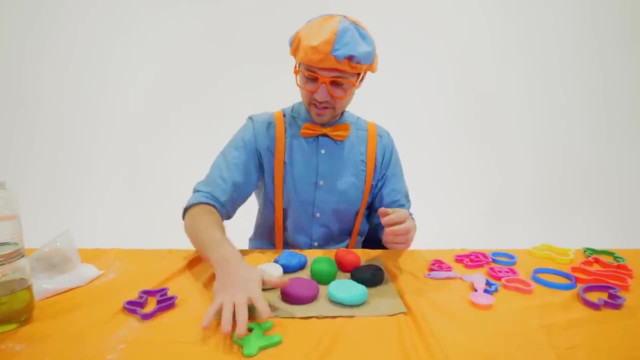 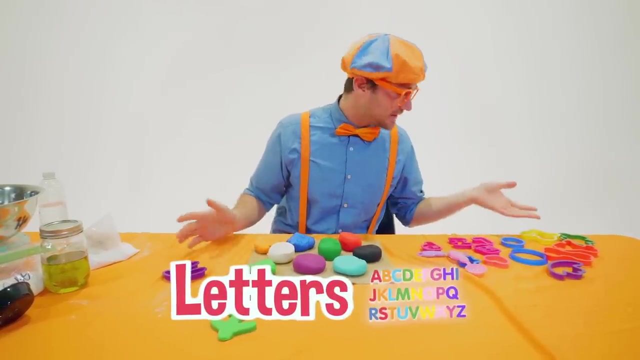 Now, let's bring all the colors that we have out and then let's see what we can make together. Okay, so let's put that green back and we have the airplane right there. what else? Oh, we have some letters. we have, ooh, a dog. 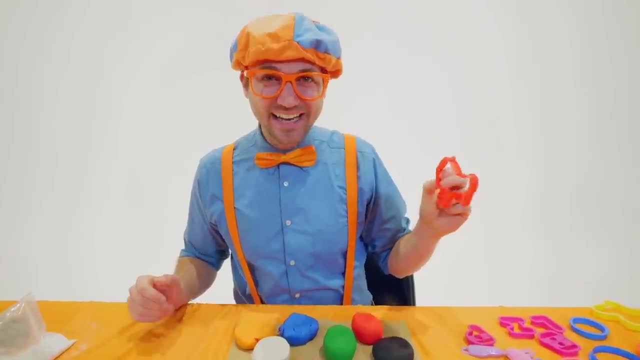 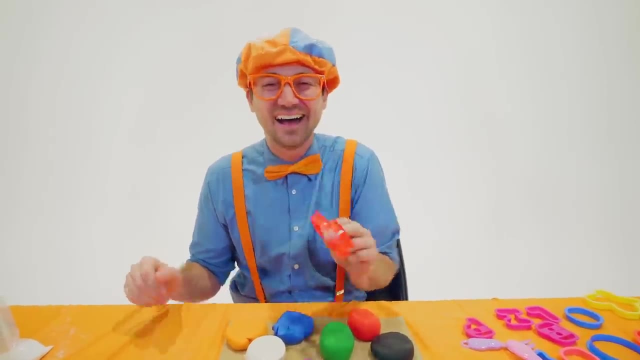 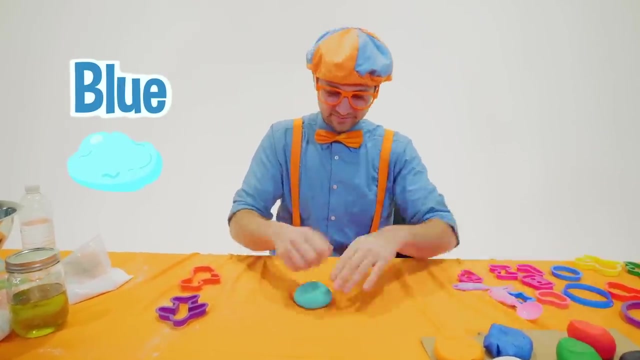 Woof, woof. will you act like a dog with me? Ready Woof, woof, woof, woof. haha, wow, dogs are so cute. Okay, let's make a blue dog. That sounds pretty silly, doesn't it? 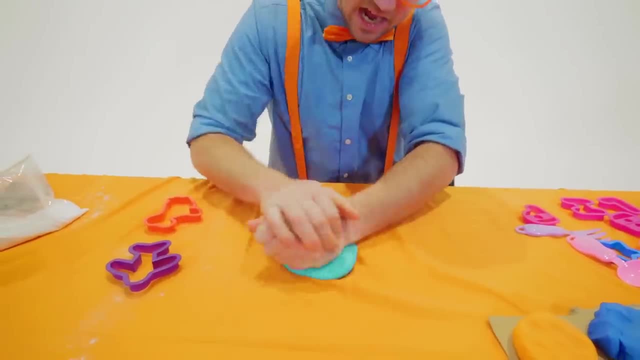 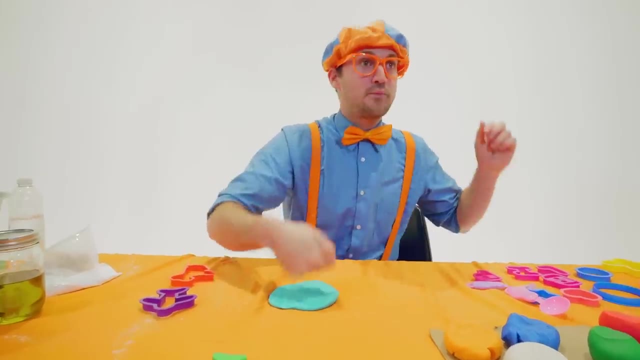 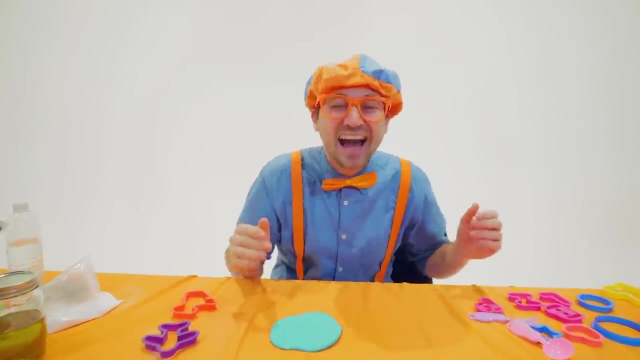 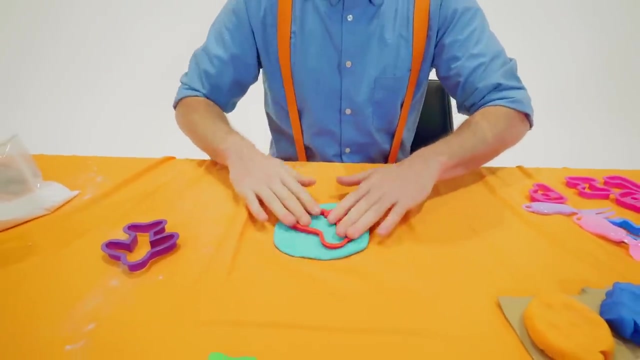 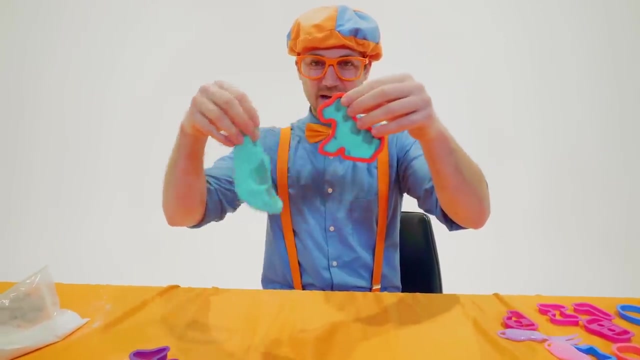 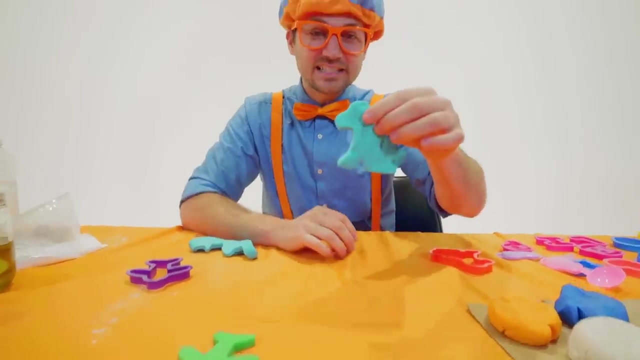 Okay, you know what to do. Smash out your clay nice and flat. Oh, okay, there we go. all right, push it down. All right, whoa, look at that. whoa pull the sides away, Wow, and now, oh, that's silly. look what is that. 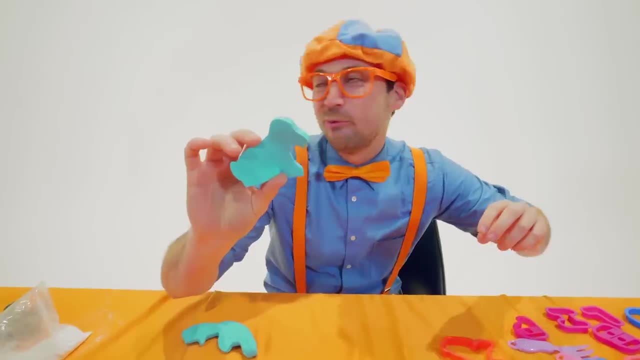 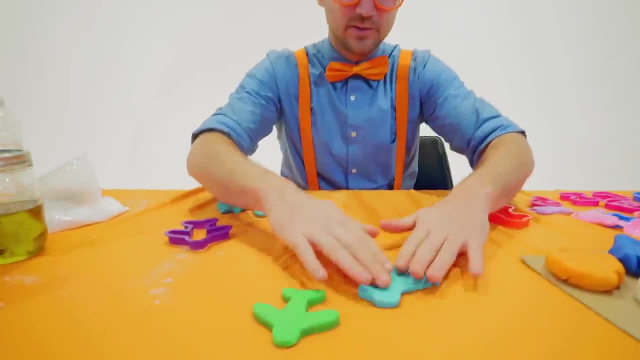 Yeah, It's a little poochie. Woof, woof, woof, woof, woof, woof, woof. Oh, whoa. Okay, we'll save you, we'll put you right there, perfect. 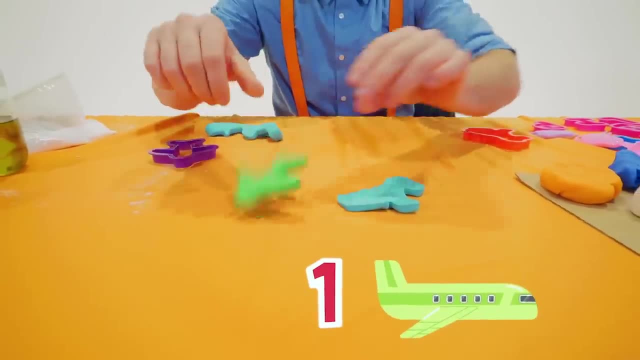 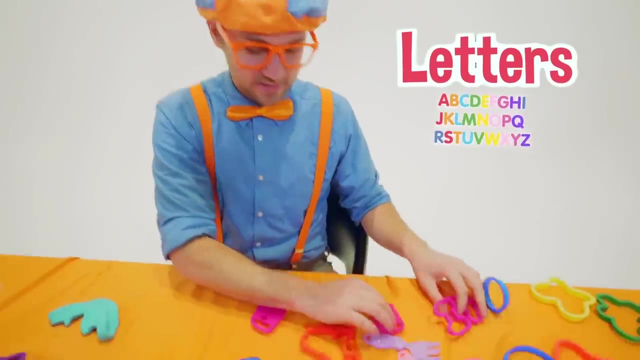 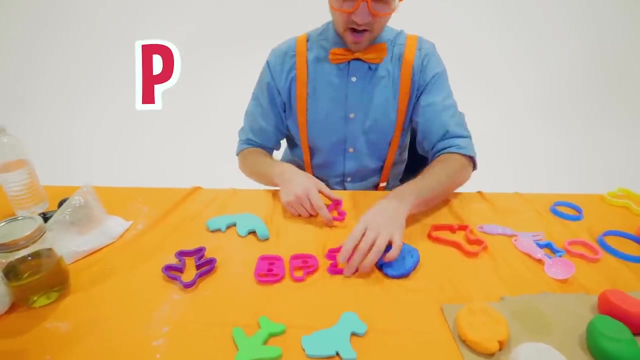 All right, one pooch and one airplane, Perfect, ooh hey, I think we have some letters over here. We can spell something out. okay, Looks like we have a B a P, an I, an L. huh, a B, a, P, an I and an L. 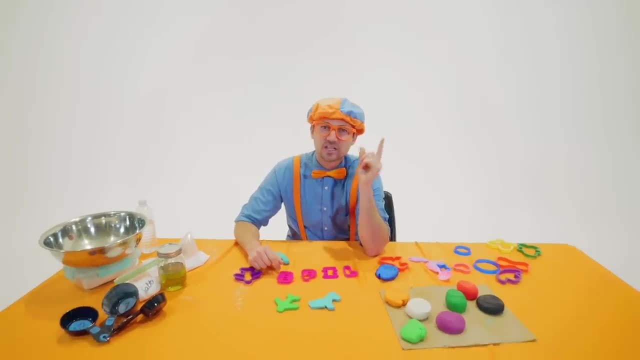 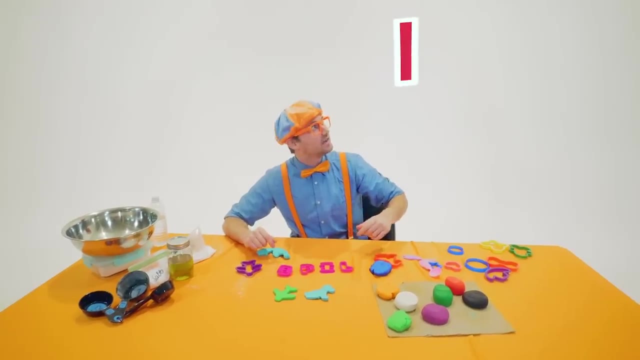 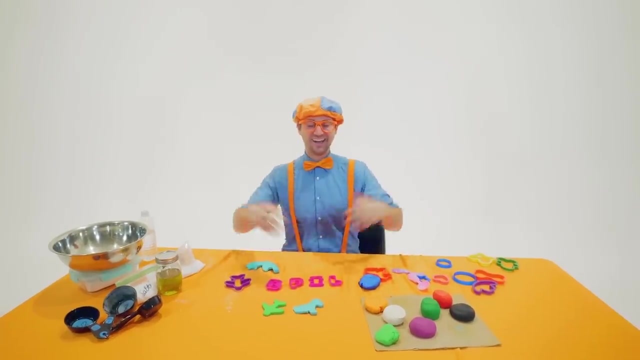 What word can you think that uses those letters A, B, a, P, an, I and an L? hmm, I know, yeah, my name. I know, yeah, my name, Blippi. yeah, we can actually spell my whole name out. 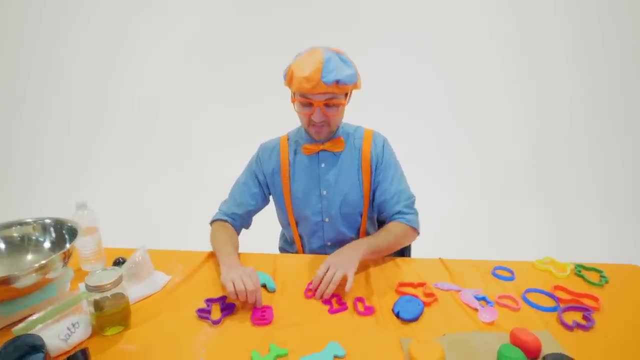 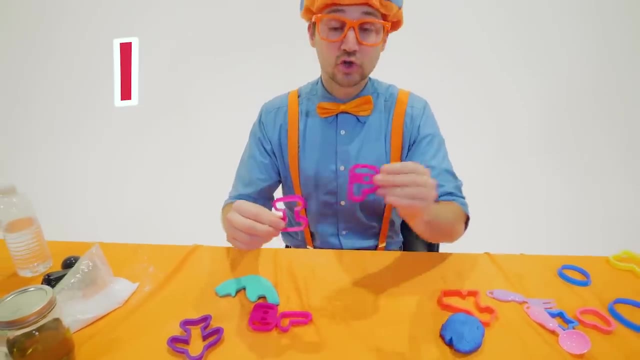 just with these four letters. See, we would go like this: We would use a, B, an, L, an, I, we would do two P's and then we would use another, I Perfect. all right, let's do that. 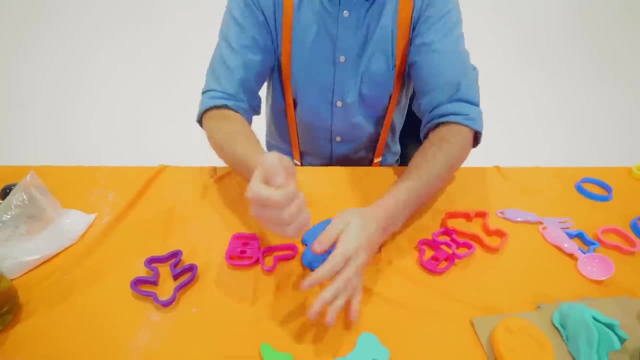 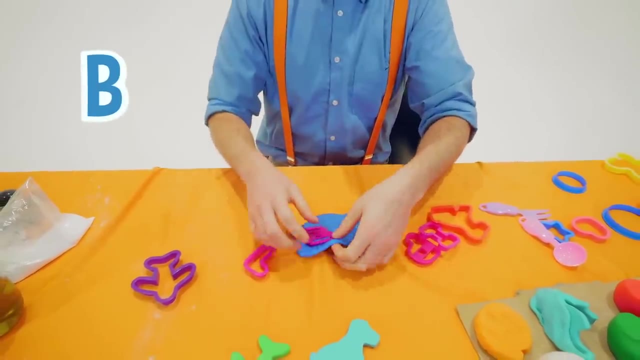 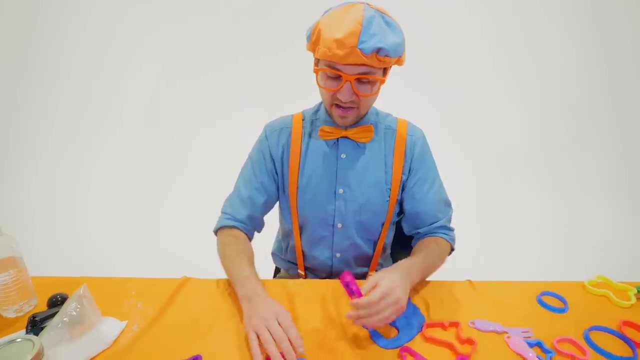 All right, first we need some colors, So let's use this blue color. yeah, There we go. Let's do a B right there. perfect, Whoa, this is gonna be so cool. Yeah, and if you use some of this at home, 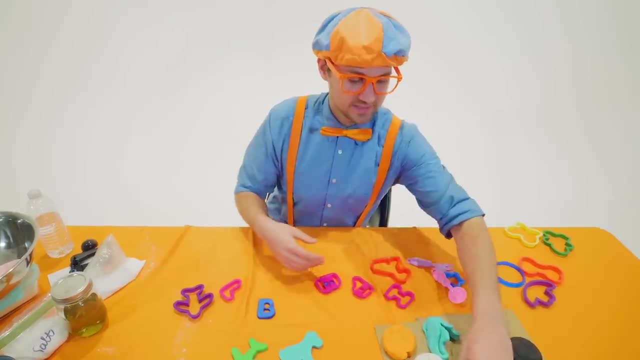 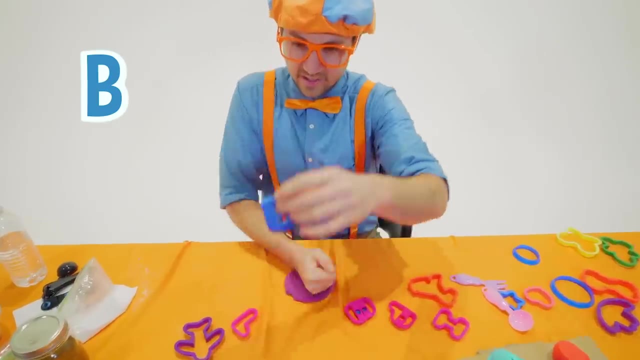 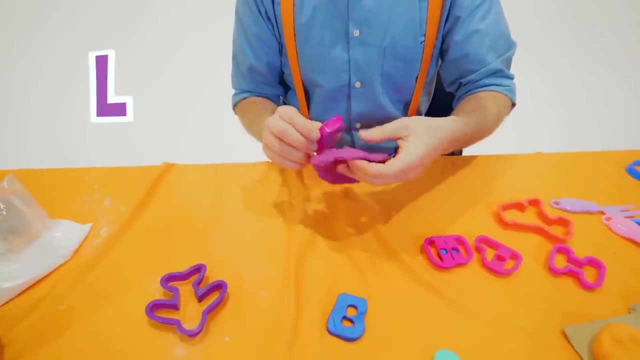 maybe you could spell your name. Okay, let's use some purple. All right, so we got a blue B right here. Yeah, whoa, okay. and then we have an L. All right, nice little L right there, yeah. 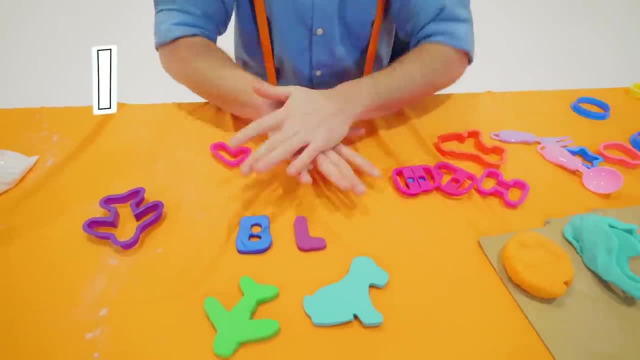 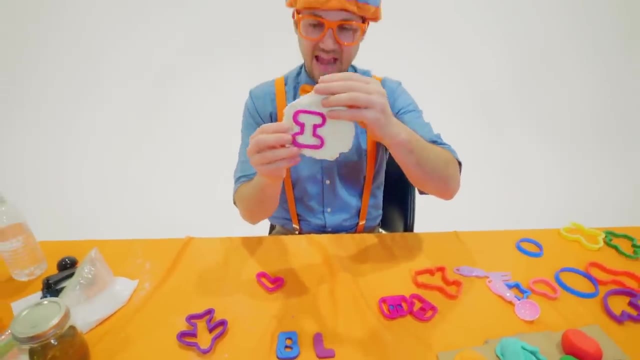 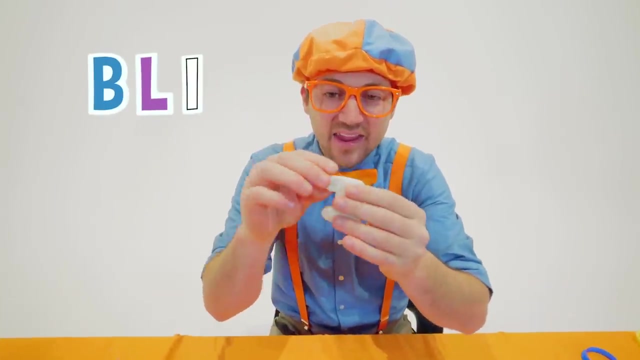 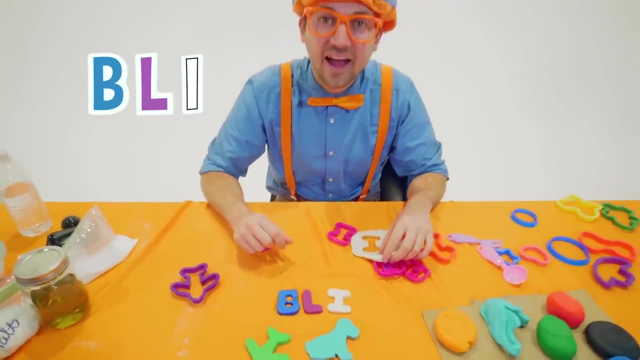 So a B L and then we need an I. How does that look? Yeah, whoa, okay B-L-I, yeah, B-L-I. what's the next letter? Yeah, P, and there's two of them. 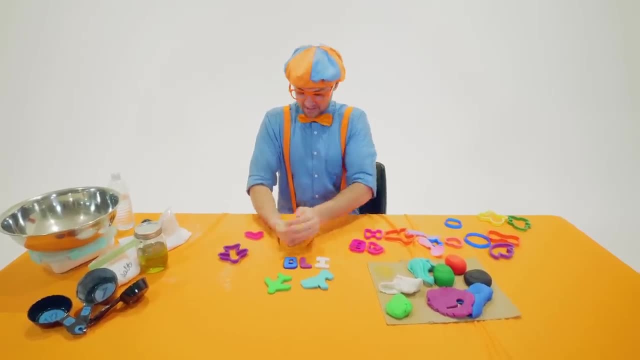 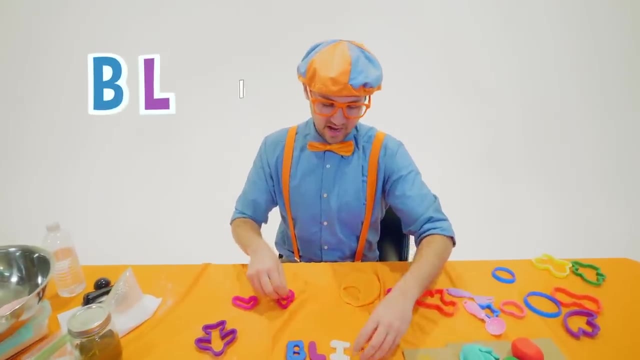 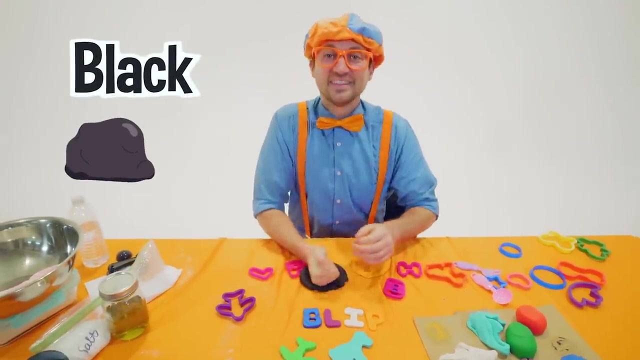 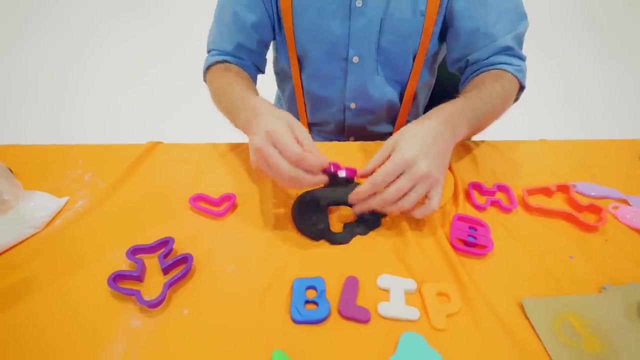 Let's use one of my favorite two colors. Yeah, the color orange. B-L-I P. we need another P. we'll use the color black. This is so much fun and it feels so cool on my hands. Ooh, another P. yeah, so we got here, we go. 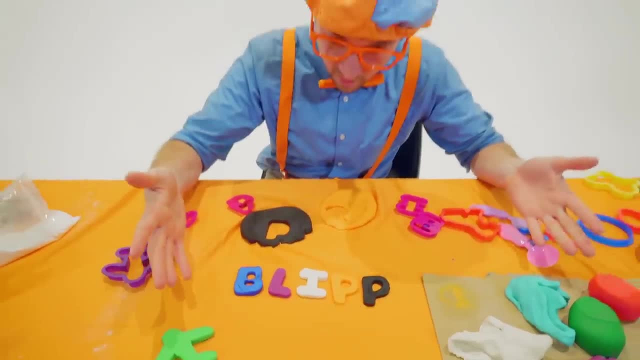 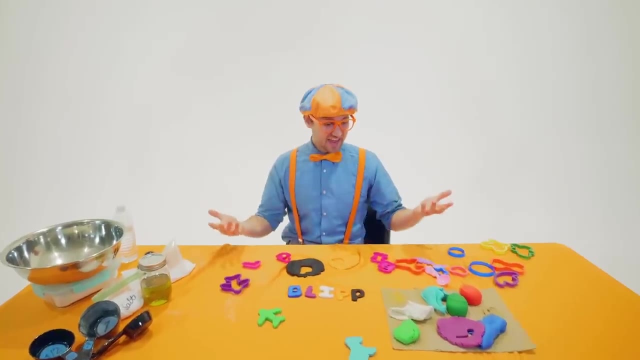 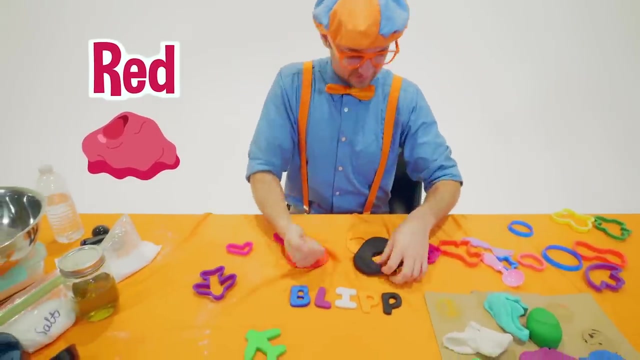 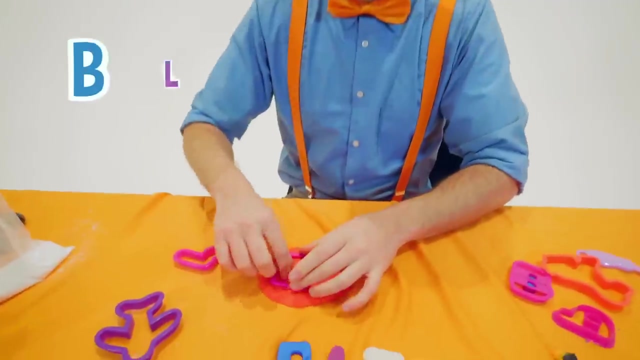 We got B-L-I- P-P. what's the next letter? B-L-I- P-P. yeah, I, and let's use this bright red color. All right, here we go. B-L-I P-P. I- here we go. 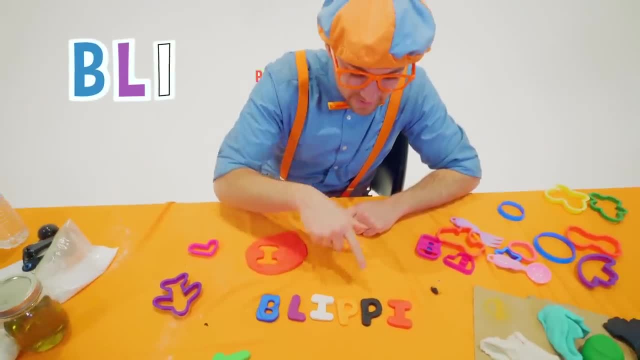 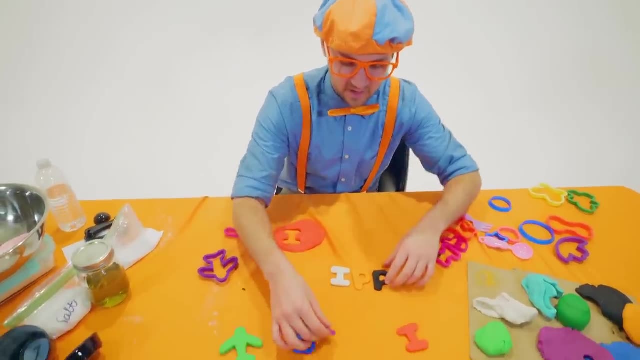 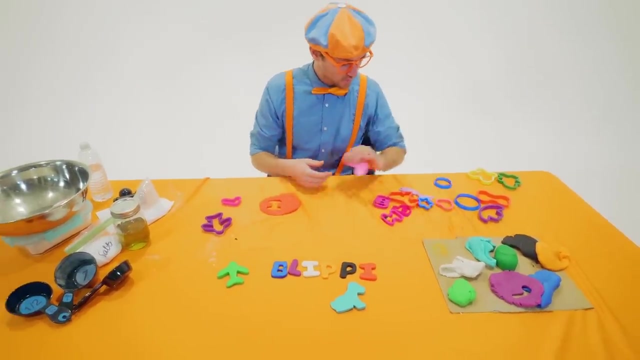 Oh, how does that look? B-L-I, P-P. I yeah, good job, All right. okay, let's put these down here with the dog and the airplane. there we go. All right. now let's make one more thing, huh. 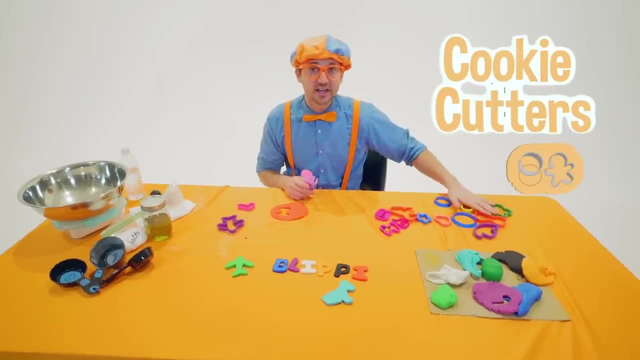 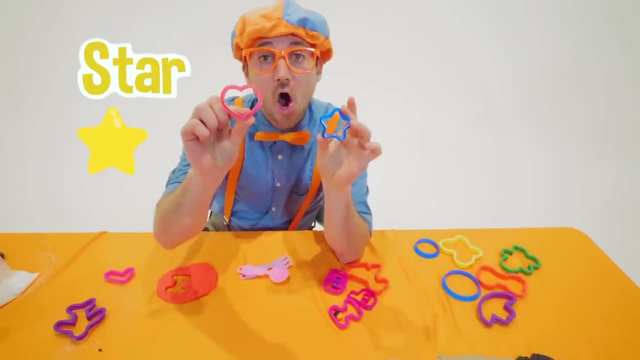 Hey, Since we had all these stencils and these cookie cutters, yeah, you could actually use a lot of them. You can make a star, you can make a heart, you could make, ooh, a butterfly, yeah, 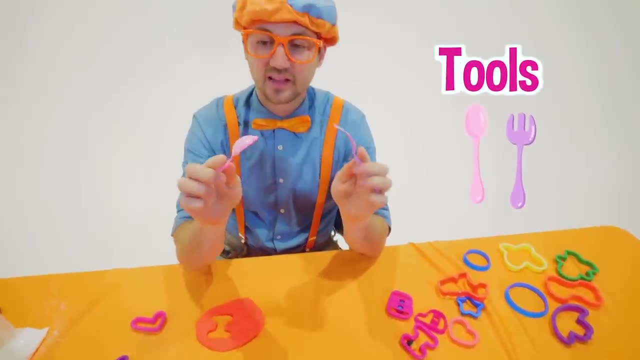 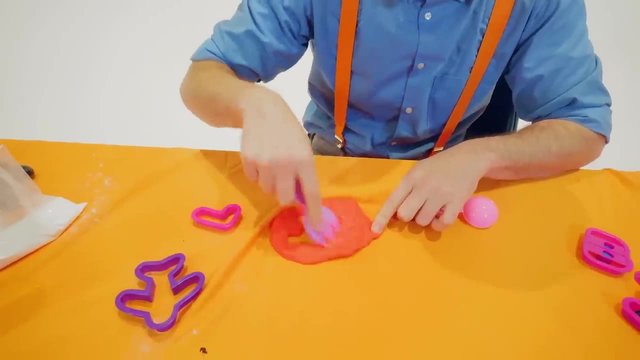 Or you could use some other tools, Yeah, like this spoon or this fork, and see, look at this. See, you can use the fork and, yeah, act like you're in the garden. doo doo, doo, doo doo. 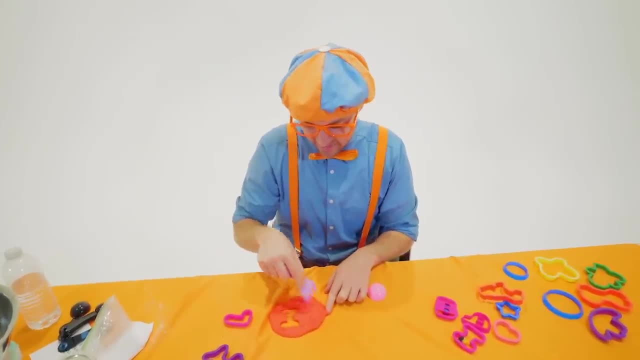 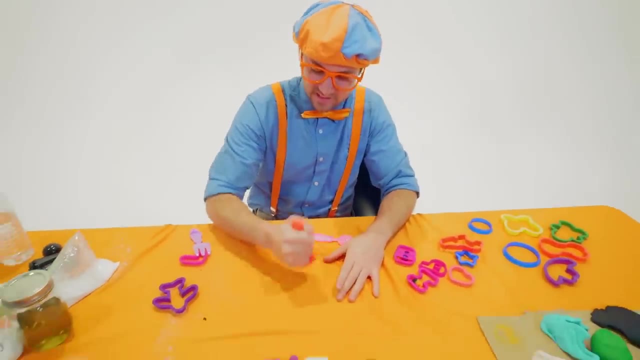 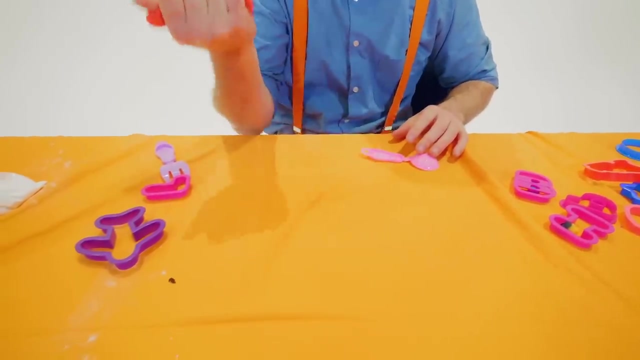 Yep, gotta make the soil nice and soft, so then you can plant some plants. Wow, but I am definitely making a mess with all these small pieces. so look at this. This is a cool trick that I learned. See, you can actually pick up a lot of the pieces. 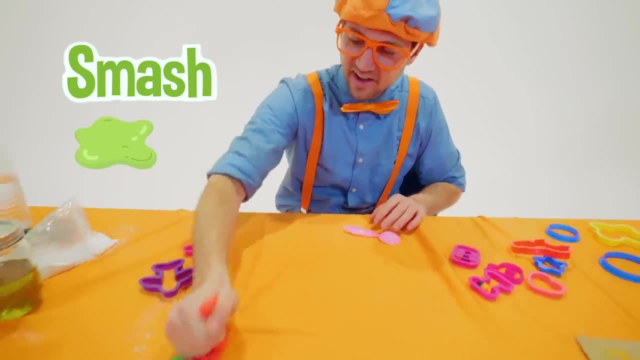 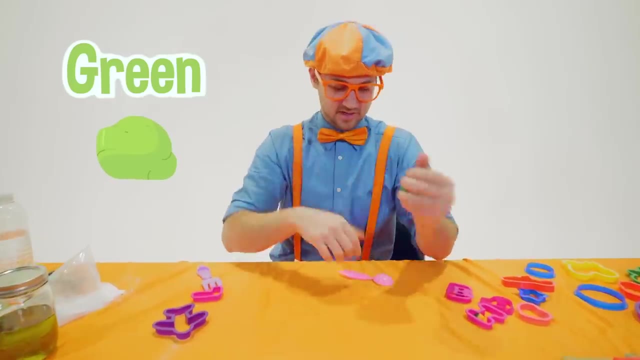 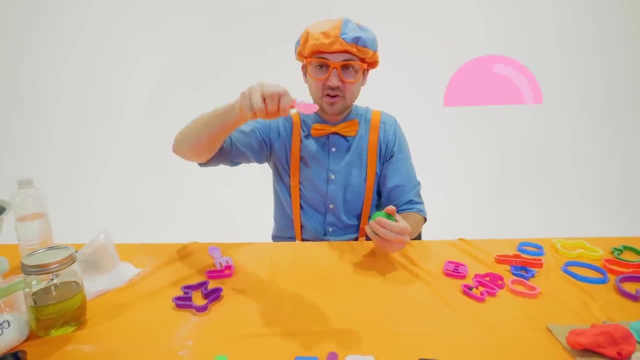 by smashing it. yeah, it's kind of fun, huh, Okay, but watch this. hey, we haven't used this color or green yet, so if you take the spoon and you scoop it, although it's a half of a circle, 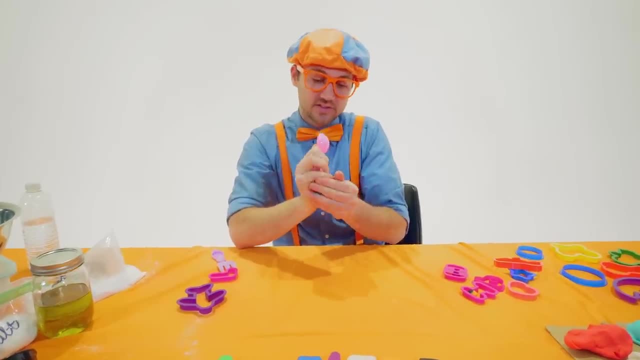 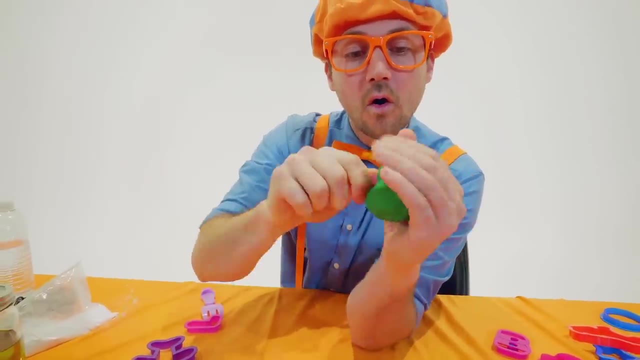 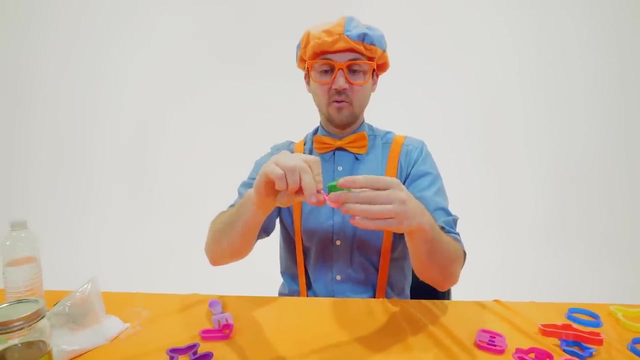 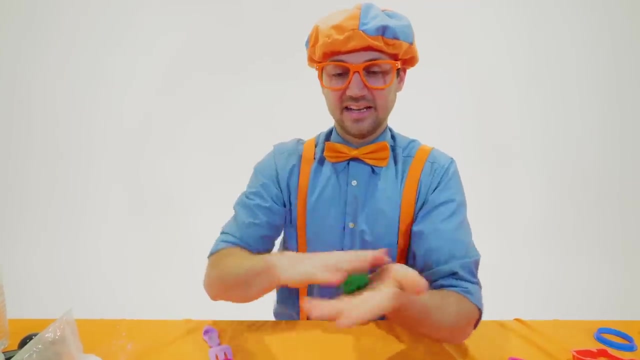 we go all the way around, you actually might be able to scoop a full circle. Okay, let's try it ready. Yeah, look, there we go. whoa, look, it's like a circle. Cool, wow, and then you can put it in your hands. 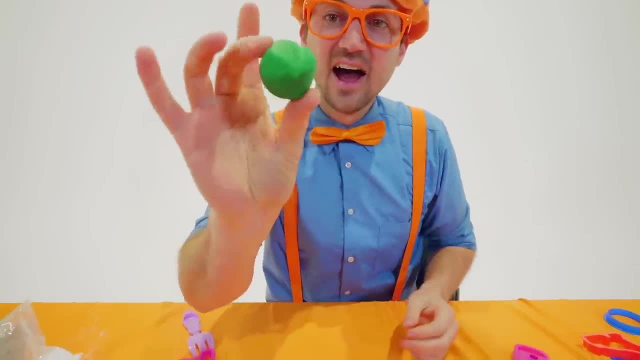 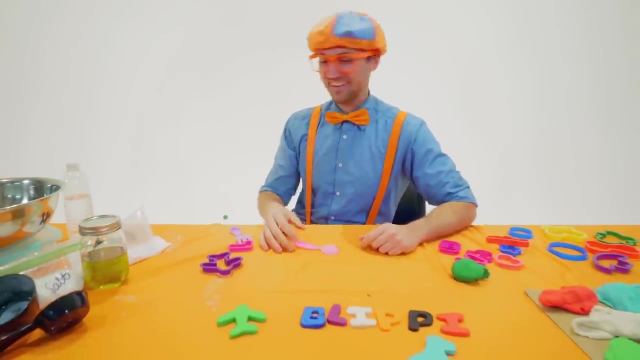 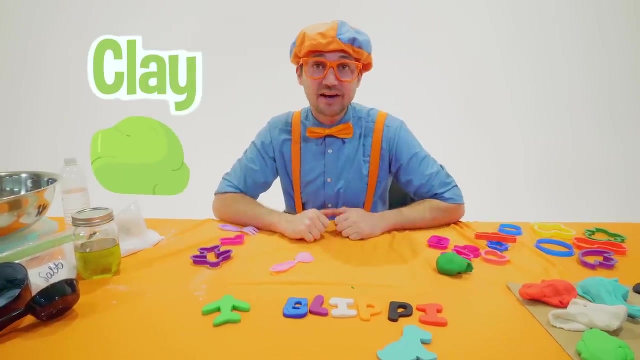 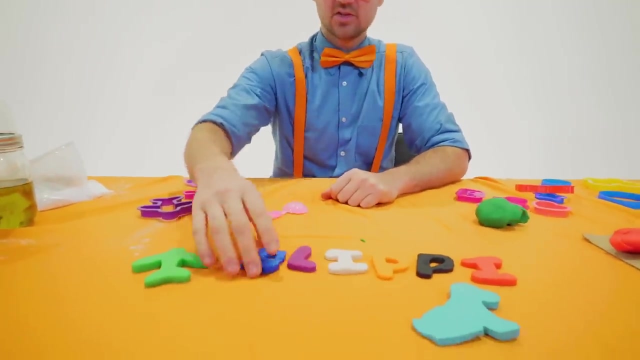 roll it around. yeah, look, it's like a basketball. Oh, that was silly. Well, this has been so much fun making this clay with you. Did you have fun making clay with me? Yeah, and it was really fun, yeah, using those cookie cutters. 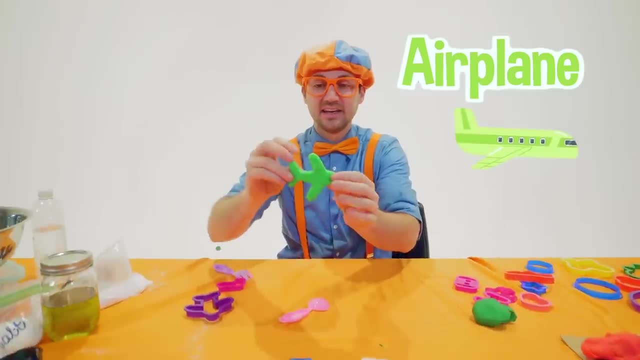 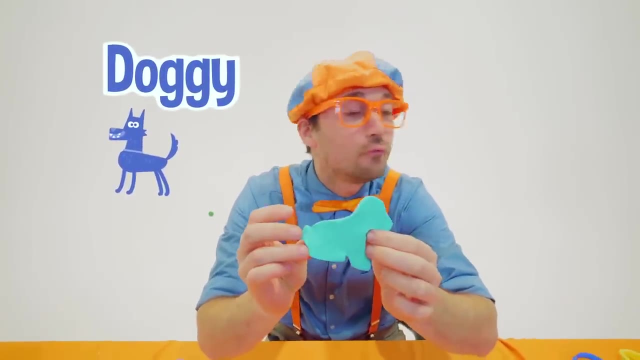 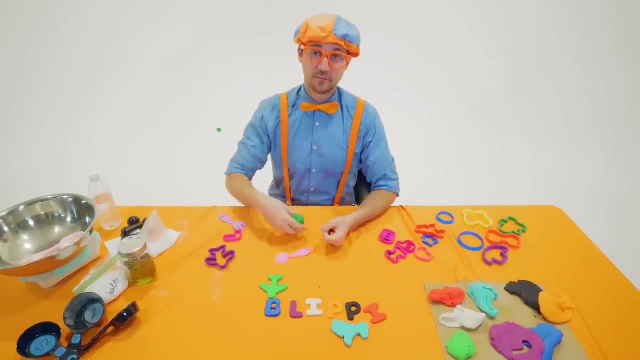 to cut out some of the clay into an airplane. yeah, a doggy. woof, woof, woof, woof and my name Blippi. Well, this is the end of this video, but if you wanna watch more of my videos, 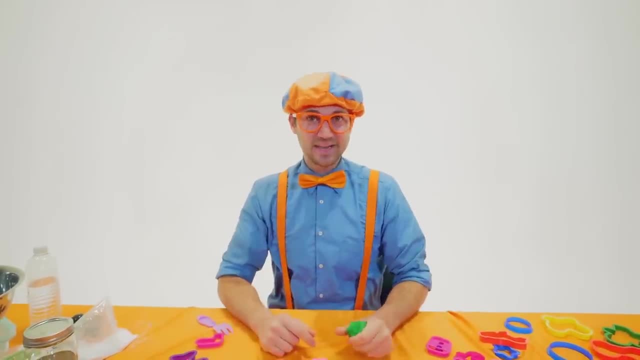 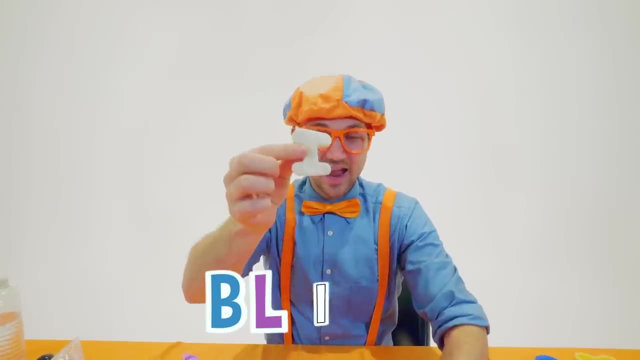 all you have to do is search for my name. Will you spell my name with me? Ready B-L-I-P-P-I-P. Blippi, Blippi, Blippi, Blippi, Blippi. A I P, PI. 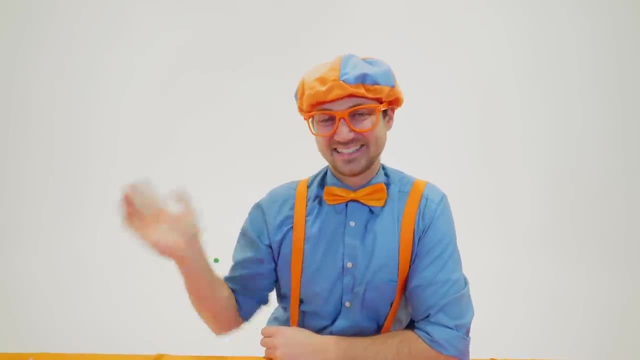 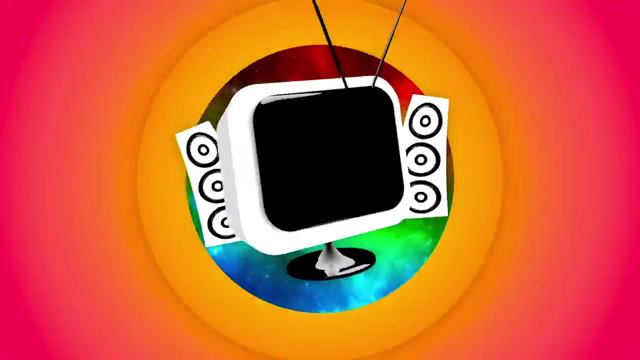 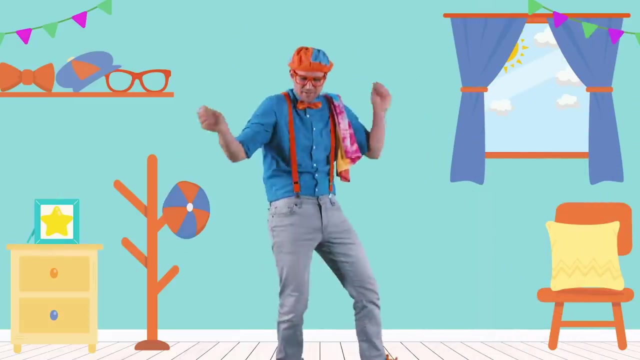 Blippi. All right, thank you so much for being my friend. See you soon, bye-bye. So much to learn about. It'll make you want to shout: Blippi. Yeah, nice music, woo-hoo-hoo. 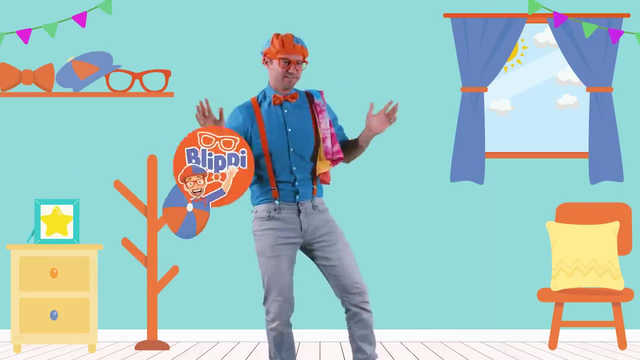 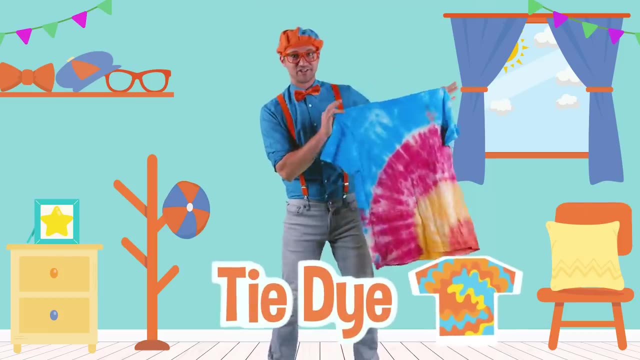 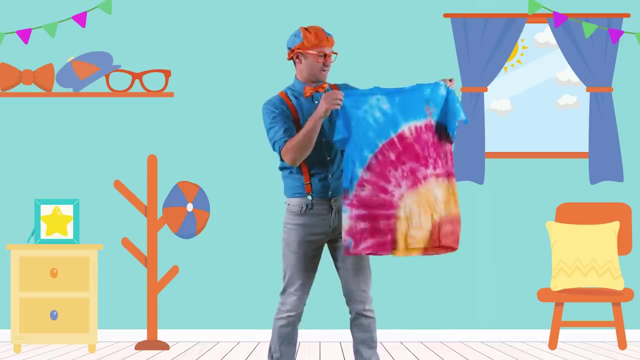 Hey, it's me, Blippi, and I was just grooves into some tunes. check this out, though. do you see this? this is a tie-dye shirt, and today, you and i are gonna make a tie-dye shirt. wow, it's so colorful. let's list all these colors. 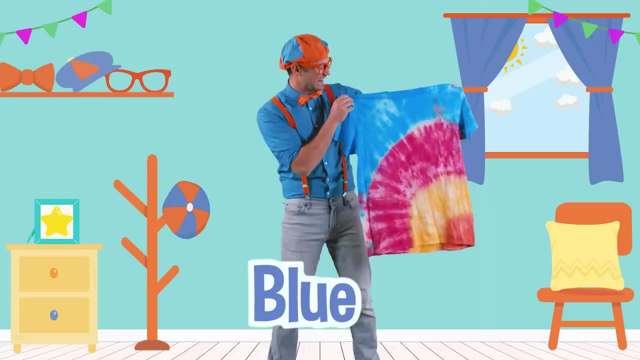 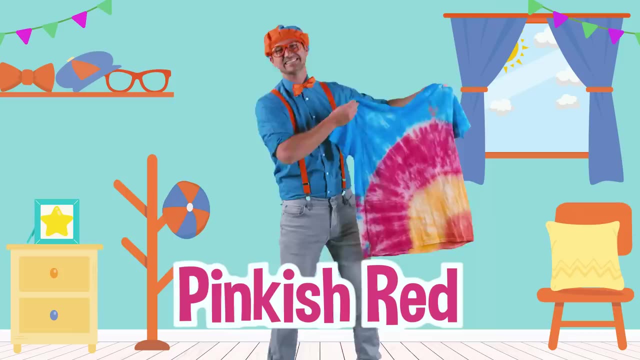 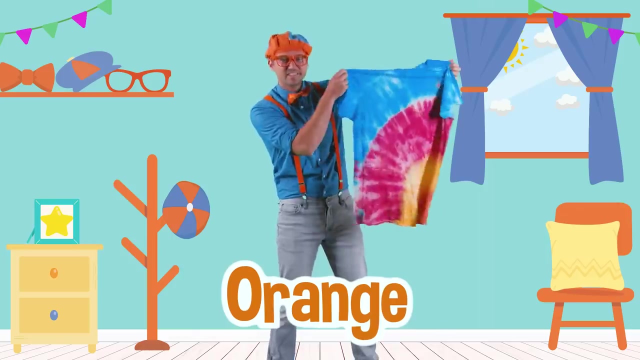 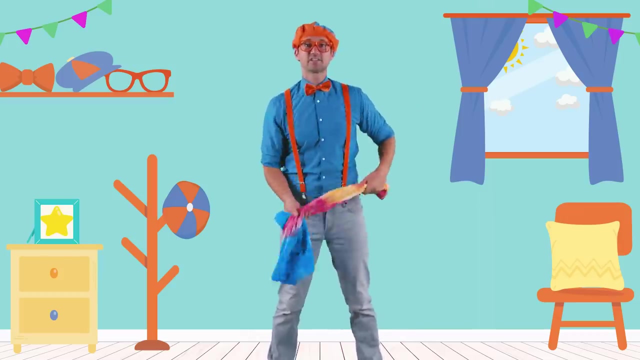 top there is the color blue. yeah, then below that looks like it's the color pink or red, pinkish red, and then we have yellow, like the color of the sun, and then we have orange at the bottom. do you see it? whoa, this shirt is so groovy. all right, let's go get some supplies and make our very own tie-dye shirt. 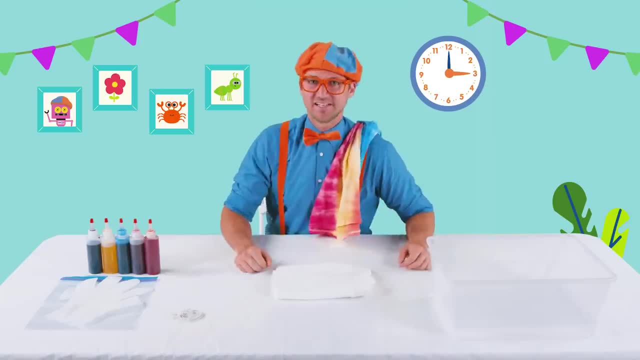 check it out. we have all the materials and supplies we need to make our tie-dye shirt. all right, we don't need this because we're gonna make one. so first you start with a white t-shirt- yeah, like this, see- and then you take a die. 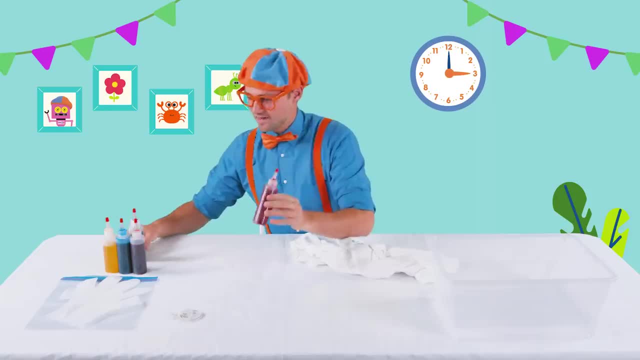 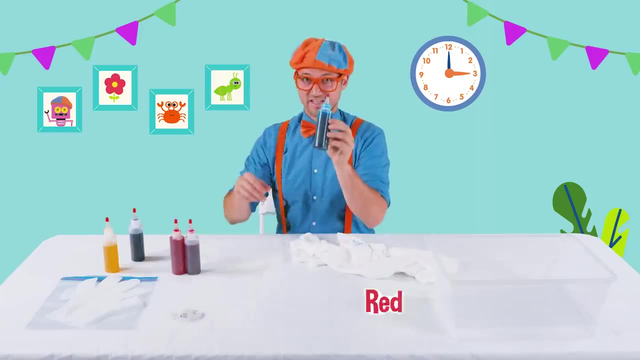 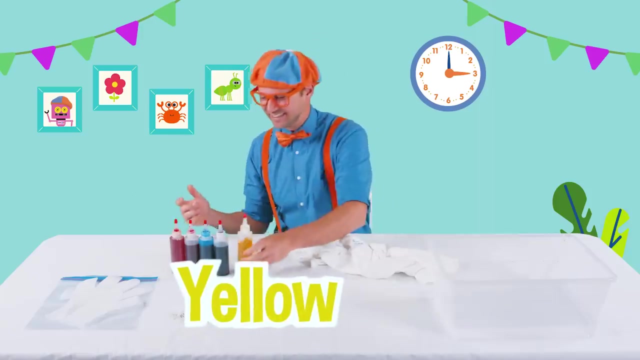 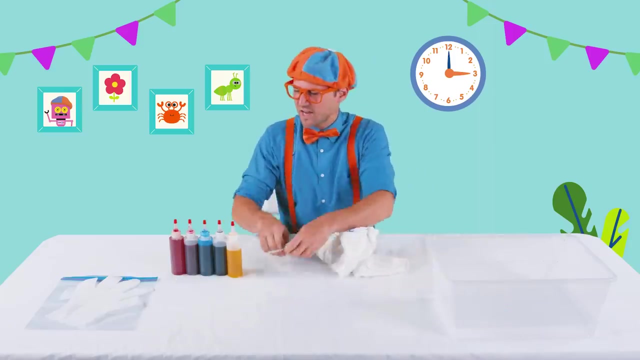 yeah, let's see a fabric die. this is the orange fabric die, this one is red, this one is blue, this one is purple and this one is yellow. and then we have some rubber bands and you tie the shirt really tight. then you spray the dye on it, but you have to wear your gloves or else your hands are gonna get. 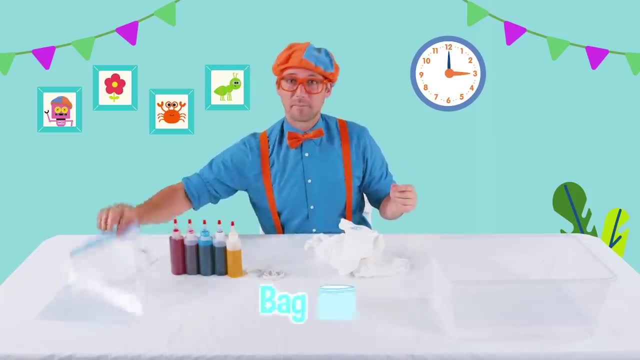 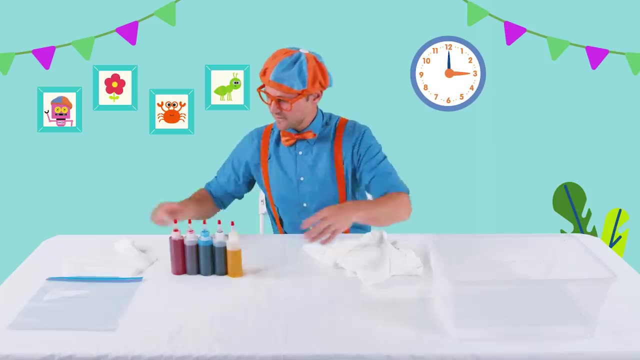 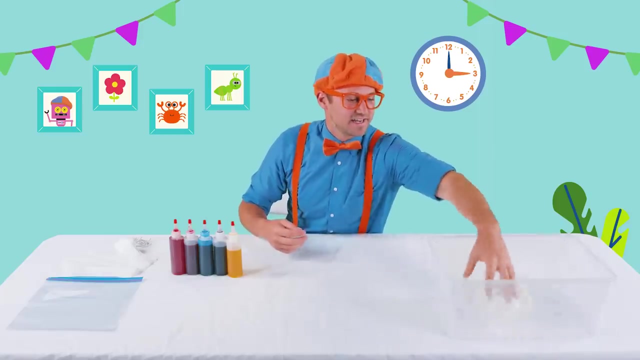 stained. i don't want that. and then we have a bag for later. i'll show you what that's all about. and the water, okay. so first step: we need to get the shirt wet, just like that. let's get it nice and wet. wow, that water's really cold. okay, squeeze out all the 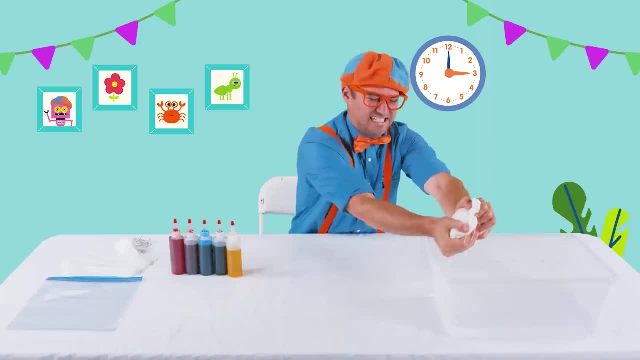 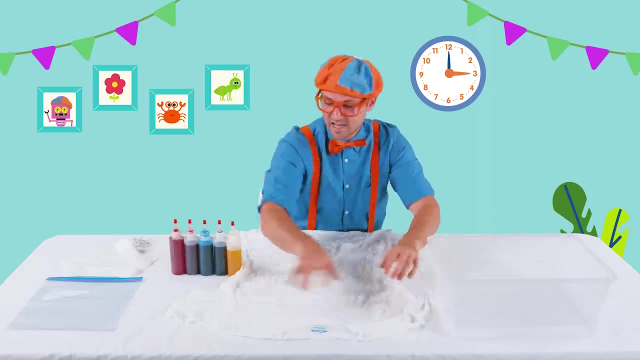 water, we're so strong, all right, and then let's lay the t-shirt out on the table. yeah, and the cool thing about tie-dye is that you don't have to do the whole thing on the table, because if you're doing it is, you can do so many different designs. 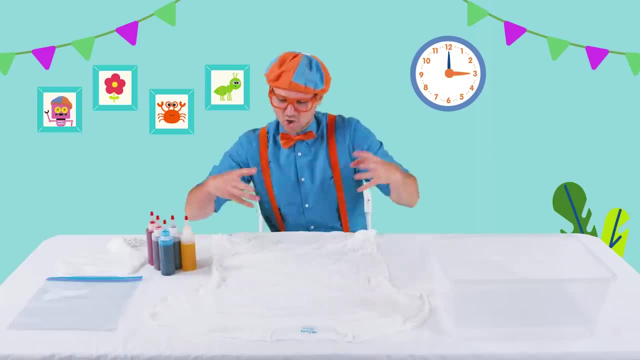 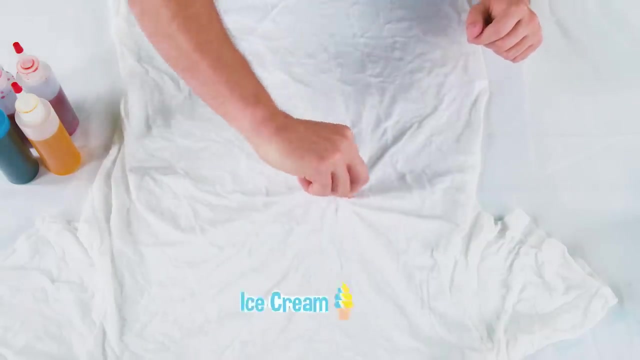 And it's all about how you twist and crunch the shirt and wrap the rubber bands around it. So let's do a swirl. I love swirls. Yeah, kind of like ice cream swirls. I love ice cream. Okay, here we go. 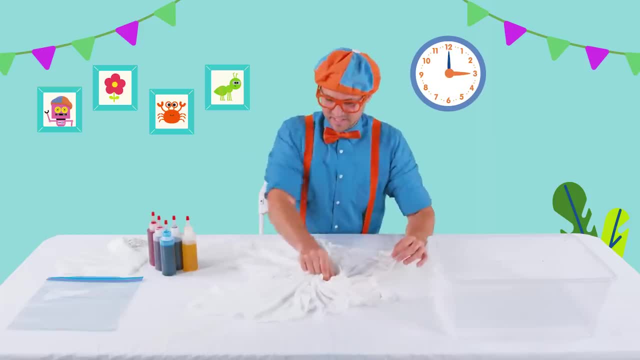 So you just twist it, swirl it and perfect. Wow, I am so excited to pick the colors. Okay, there we go. And then you have a nice bunched up shirt. You could even bunch it, but I chose to swirl it. 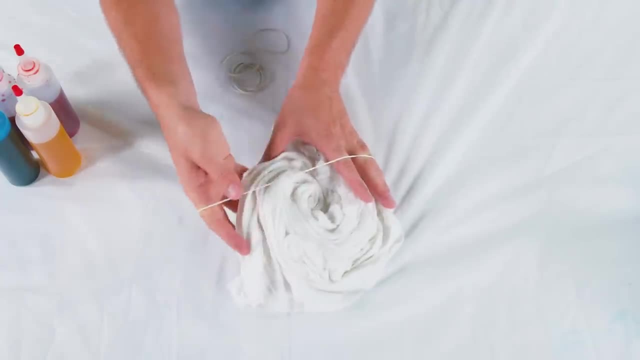 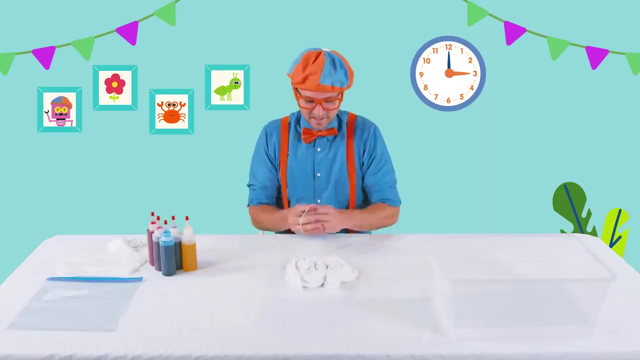 And then you take these rubber bands and wrap them around the top and the bottom of the shirt, Just like this. Yeah, This white shirt is going to be so colorful. All right, There's two rubber bands. Here is three rubber bands. 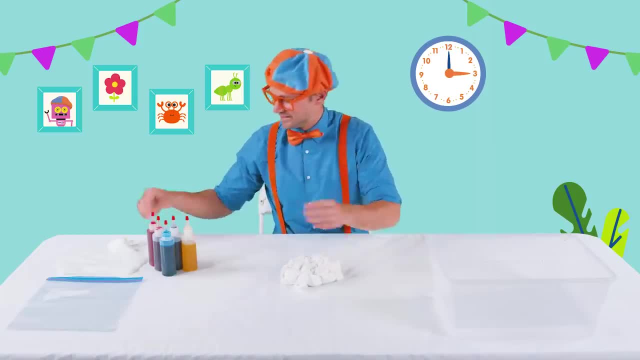 Perfect, This is looking so good. And then there's the fourth rubber band. Wow, Will you count to four with me, Ready Ready. One, two, three, four, Good job, All right, Now we get to pick our colors. 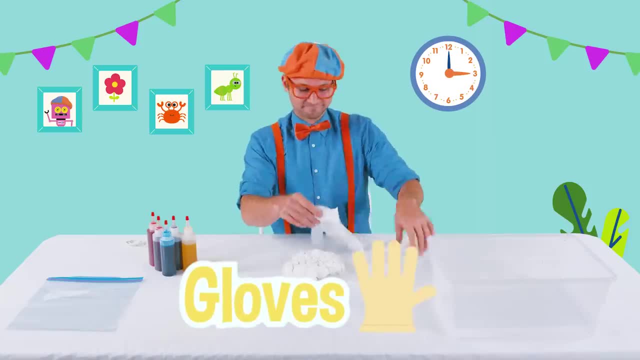 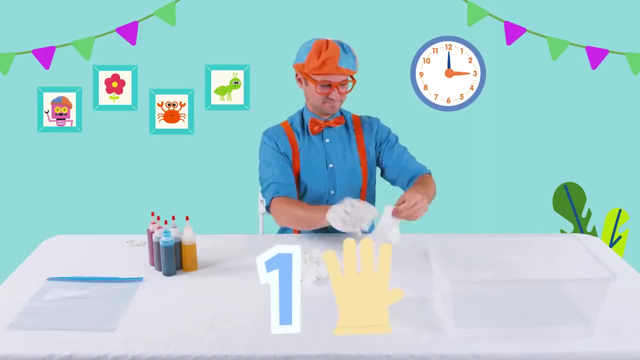 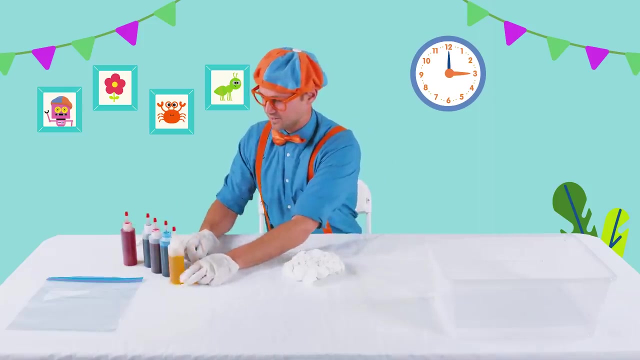 But remember, let's put on our gloves. Here we go: One glove, Two gloves, One, two. All right, Let's see We have a lot of colors. I know I think I'm going to choose two colors. 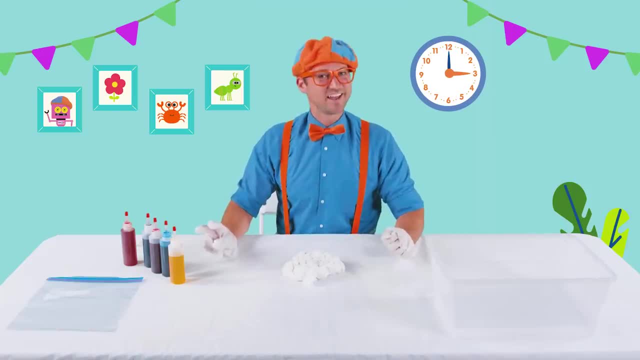 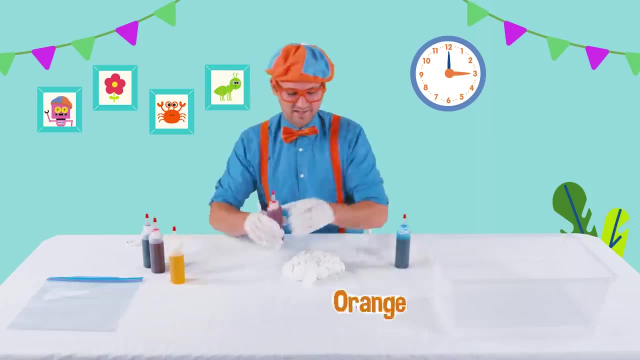 My two favorite colors. Do you know what colors they are? Yeah, I bet you do. Yeah, Blue and orange. All right, Here's the two colors, And then take the caps off, And then you get to squirt the shirt in whatever way you want. 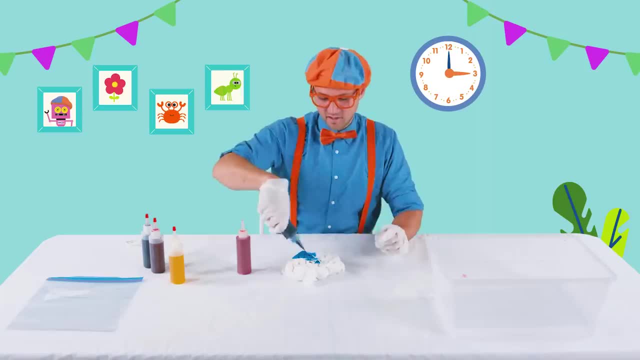 I'm going to squirt some blue right there. All right, I'll skip some and squirt some blue right there. How about some blue right there And some blue right there? Wow, The shirt was all white, But now what color is it? 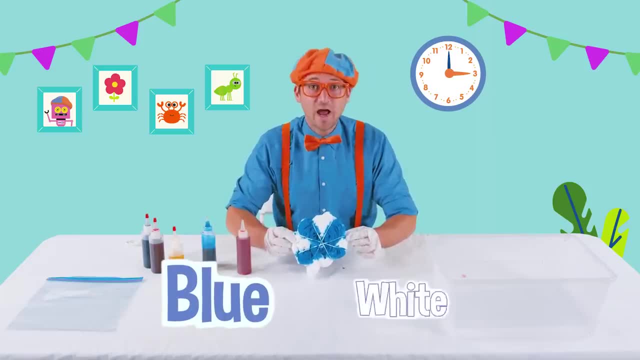 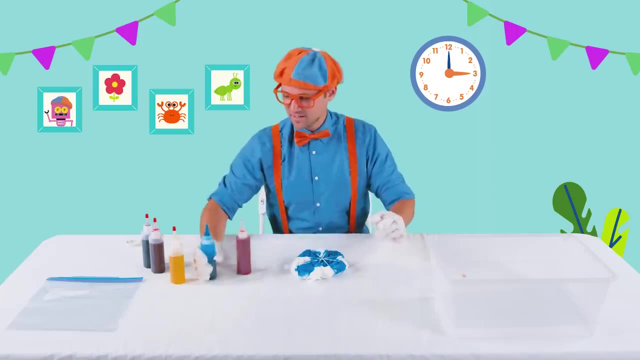 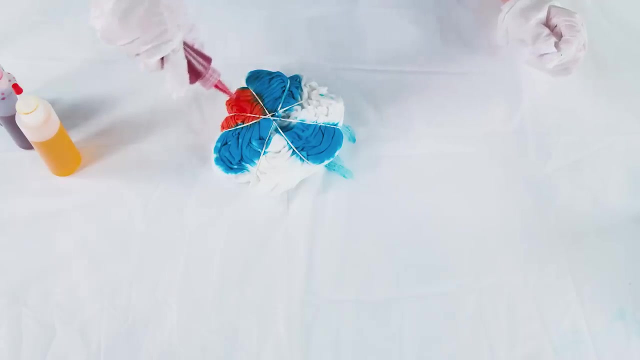 Yeah, there's two colors: Blue and white. Yeah, All right, Let's give it a little more Wee, wee, wee, All right. So then the other color, like I said, is orange. So Let's squirt that white and get it nice and orange. 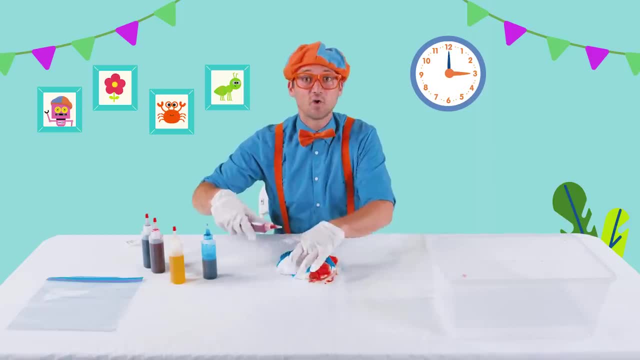 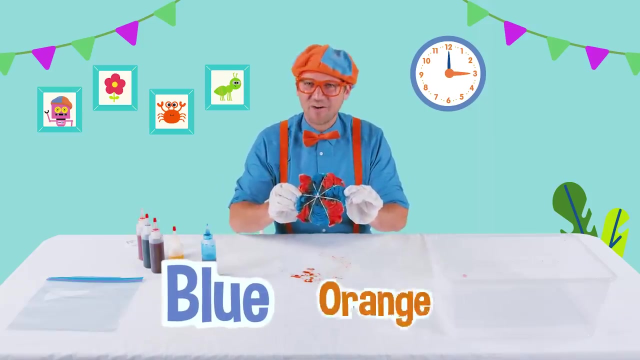 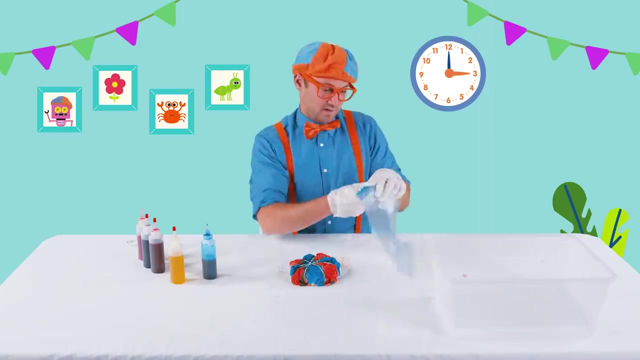 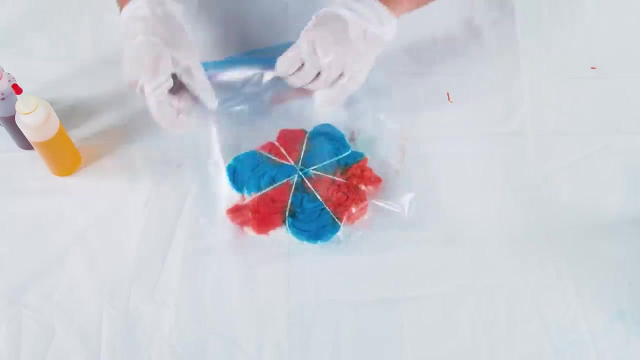 There we go. Wow, We are doing so good. Go Perfect, Wow, Amazing, Wow, This looks so good. Do you see it? We have blue and orange. All right, Set that down. And now you take The big plastic bag and put the shirt in there and close it up. 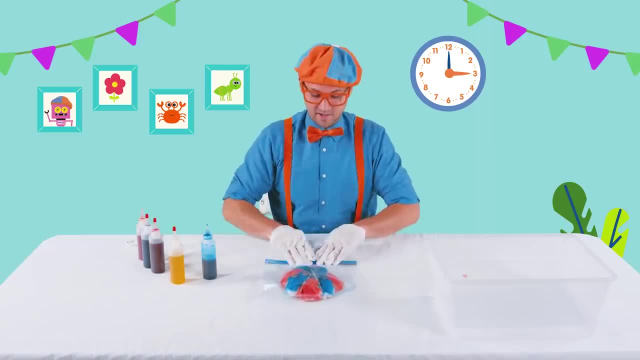 And now we get a weight, but you have to keep it in here for at least six hours. You can even do it up to 24 hours if you wanted to. The longer you keep it in this bag, the darker and more vibrant the colors are going to be. 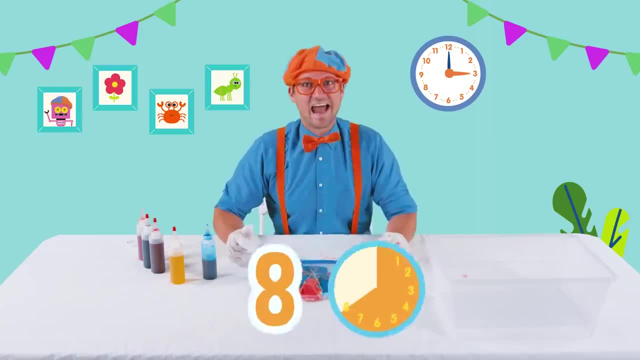 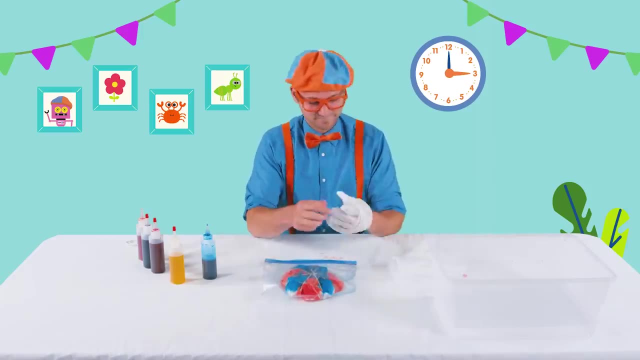 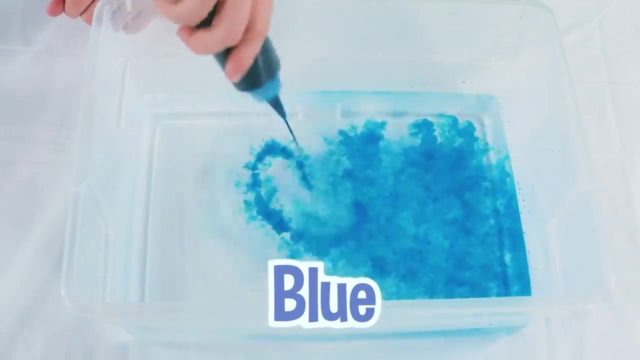 Hmm, I think we should probably wait eight hours. So let's wait. We're almost done waiting, But I think what we should do is mix two colors and see what color it makes. First let's take our blue Whoa. 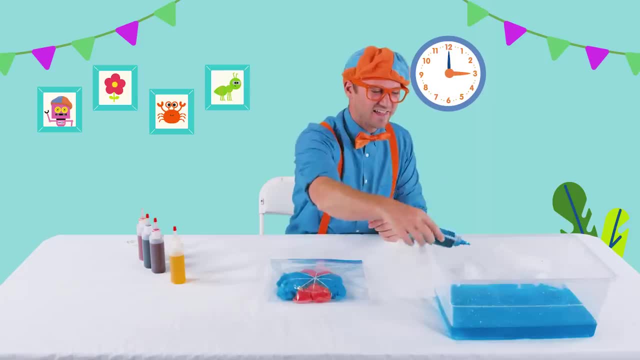 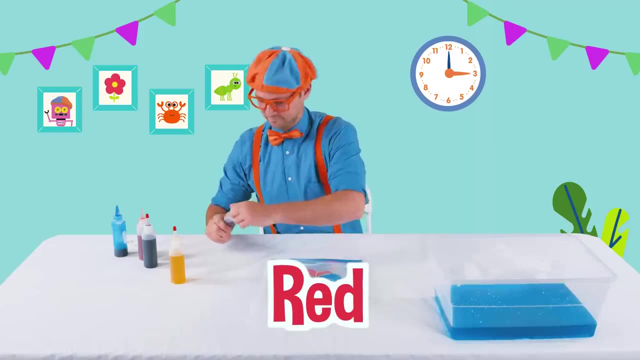 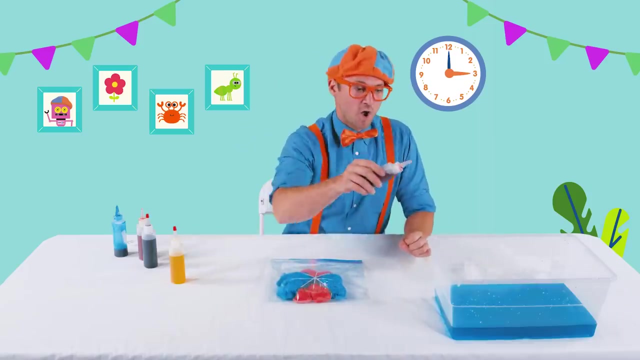 Oh, do you see that? Whoa, That's awesome. Wow, Blue water. Then let's take How about red? Hopefully it doesn't spill on me, because I don't have my gloves on anymore. All right, Here we go. 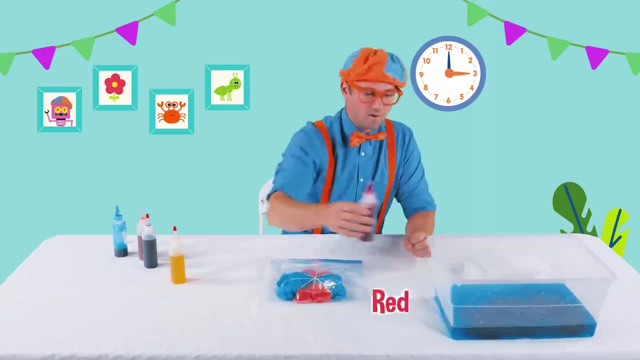 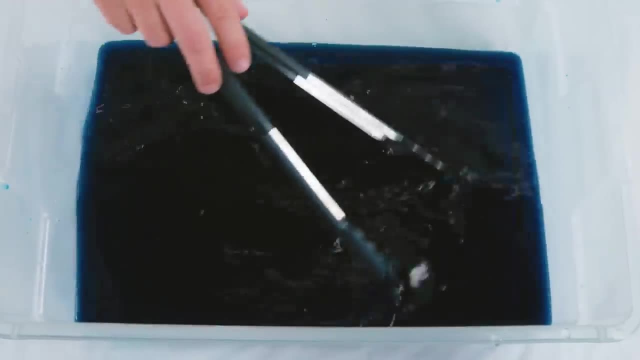 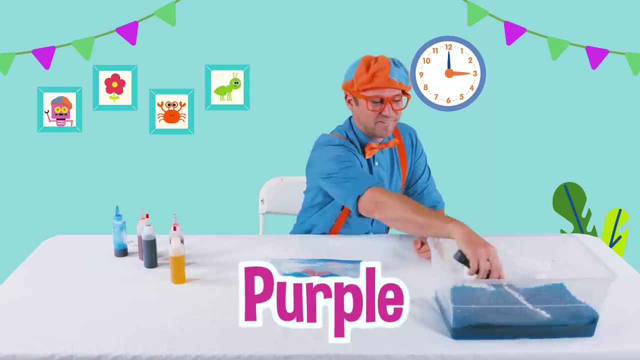 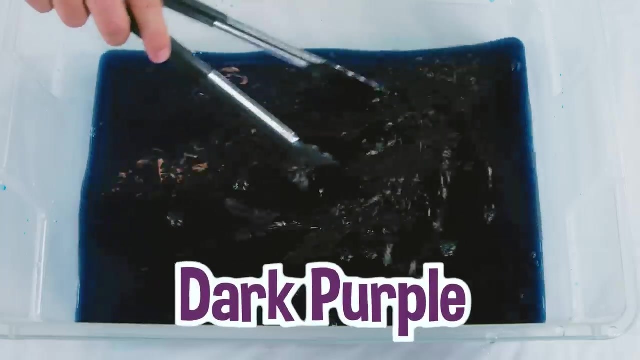 Blue and red- Whoa, What color is that? I have my mixing tongs, Wow, Yeah, Blue and red Make the color purple. Purple, Whoa, Let's put a little bit more red in there. Wow, Now it's a dark purple. 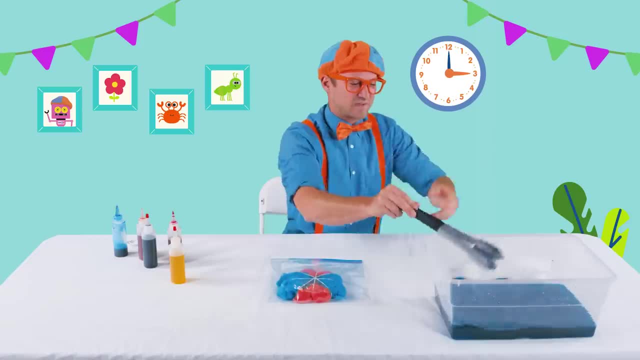 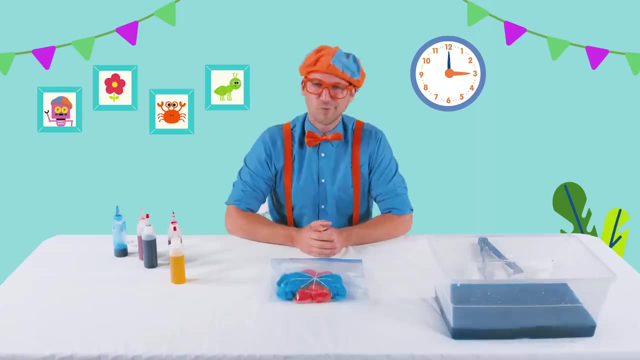 Whoa, That's fun, Okay. Well, I think our t-shirt has been in here for long enough. It's been about, yeah, multiple hours. So now I'm going to go take this to the sink, take the rubber bands off and rinse it off. 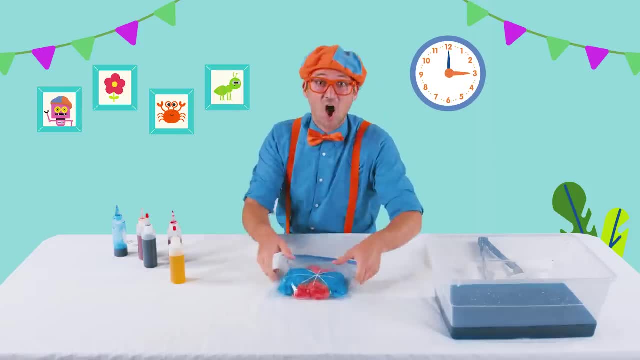 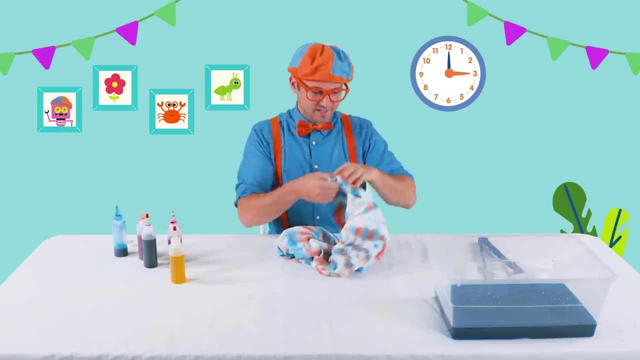 And then I'm going to go put it in the dryer. Hmm, I'll be right back, okay, Wow, This is awesome. Our shirt is complete. Wow, All right, Here it is, Do you see it? Wow, Yeah. 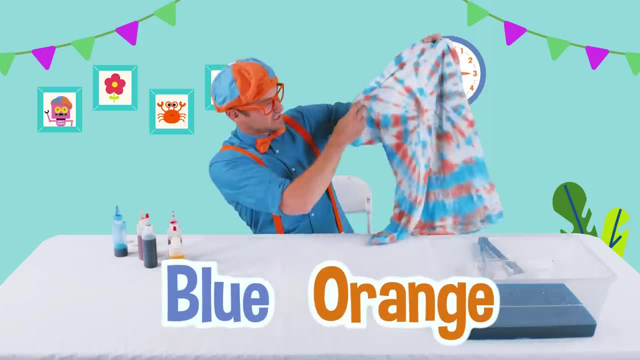 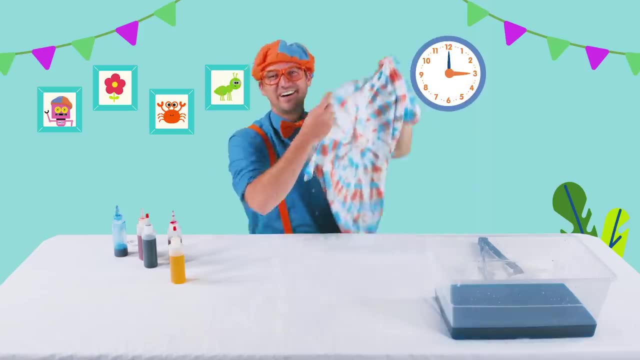 It's blue and orange. Can you see how it where? I swirled it Right about there. Whoa, It's so cool. Time to try it on. Here we go. First, we're going to take a look at the shirt. 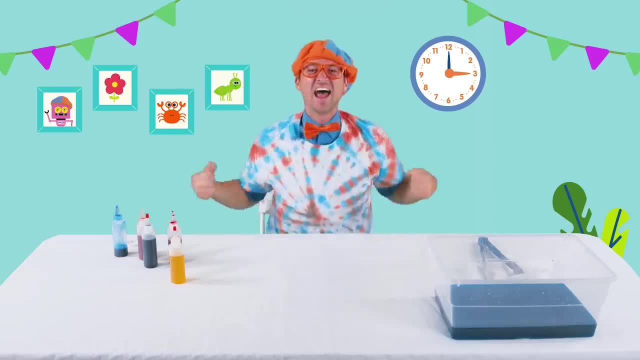 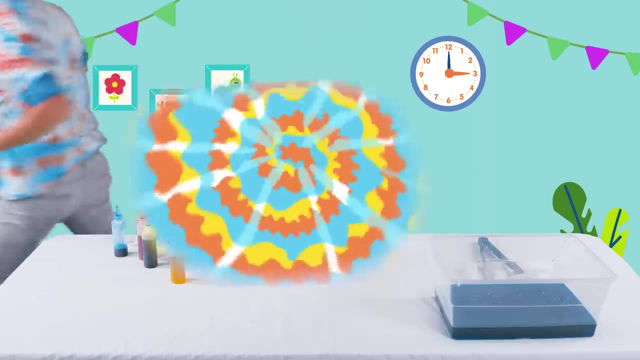 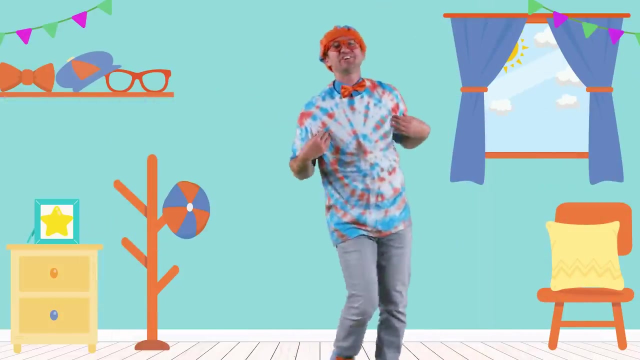 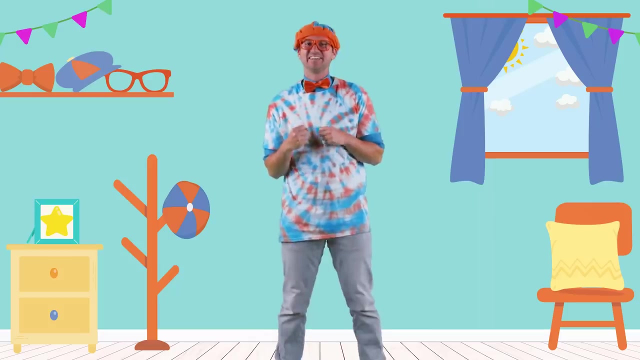 Whoa, How do I look? That was awesome. I love making tie-dye shirts. Woo Yeah, Woo hoo hoo. I sure do love tie-dye shirts. Whoa, Maybe now at home, you can make your very own tie-dye shirt. 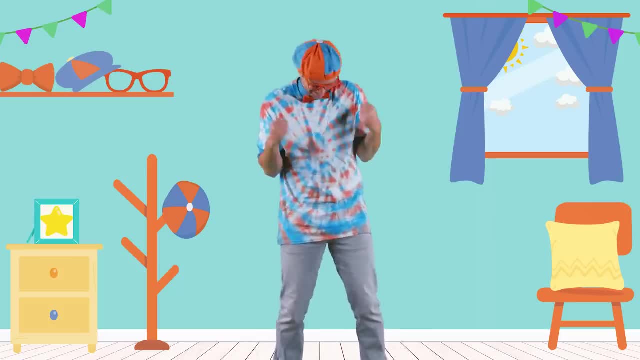 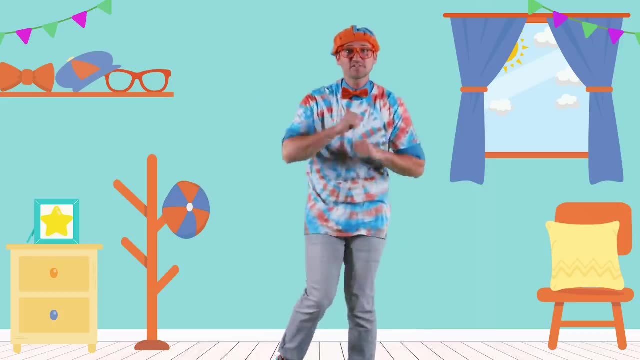 I am so excited to see that, excited to see the creation that you make. all right, well, this is the end of this video, but if you want to watch more of my videos, all you have to do is search for my name. will you spell my name with me? 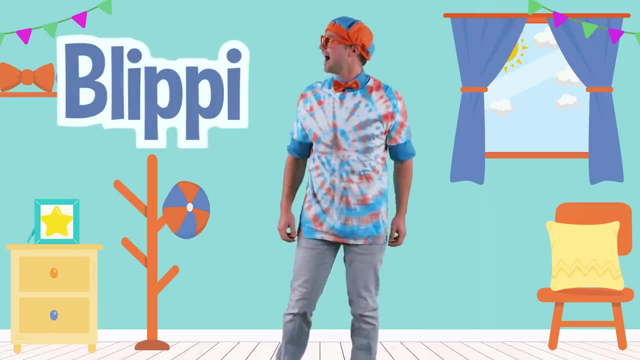 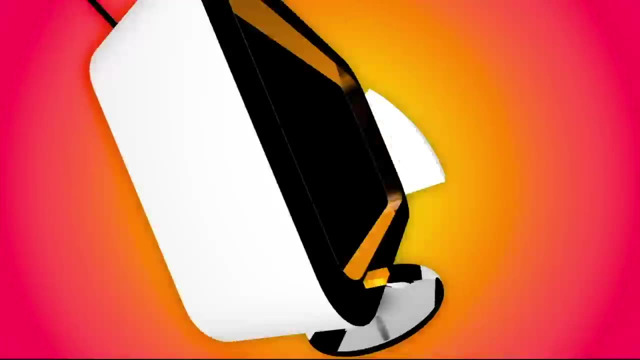 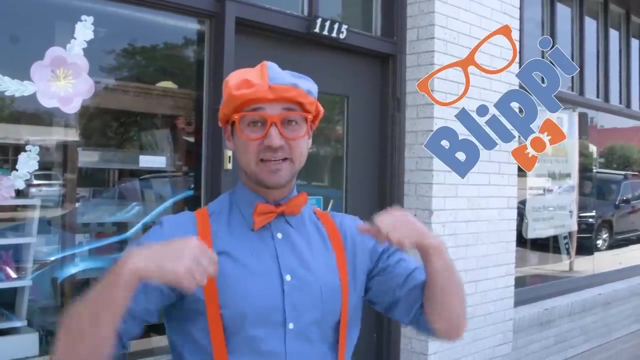 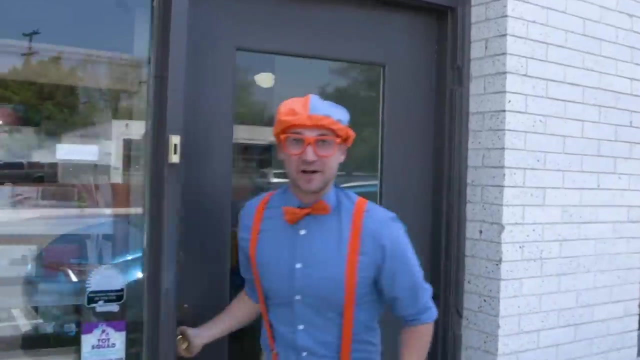 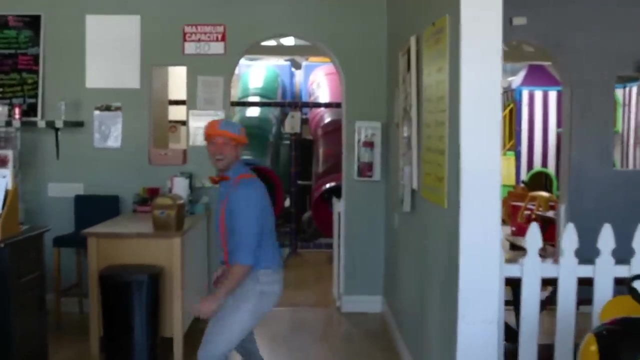 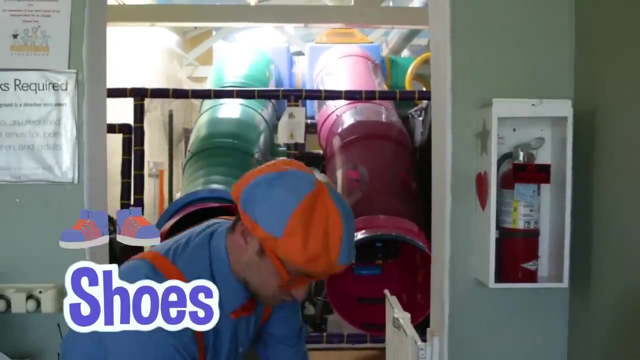 B L I P P I. Blippi, good job, all right, see you later. hello, it's me Blippi, and today we're on Amy's playground in South Pasadena, California. come on, we're going to learn our colors. this place is so cool. we can't go past here without taking off our shoes. 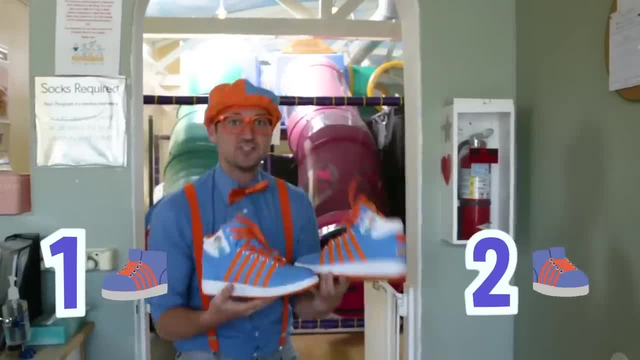 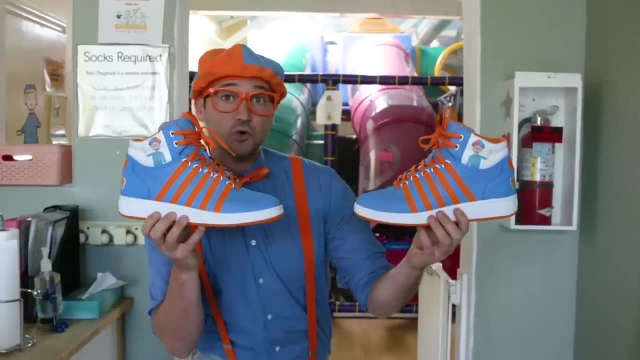 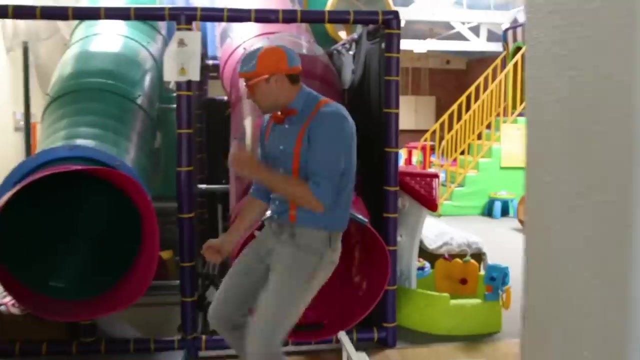 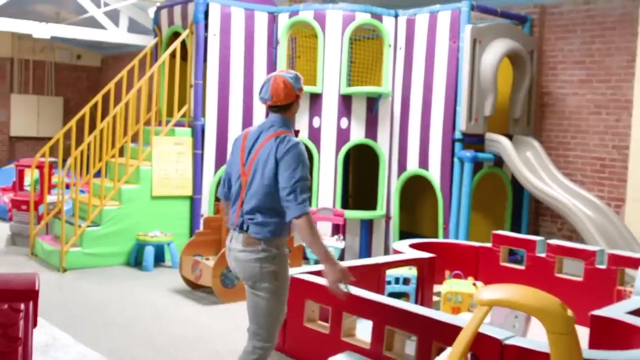 haha, Here's one shoe and here's two shoes. Hey, what color are my shoes? It looks like there is blue, orange and white. Woohoo, Let's go. Whoa, this place is so colorful. Whoa, I love playing around here. 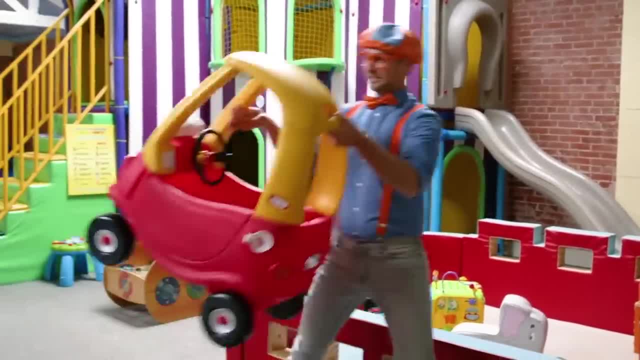 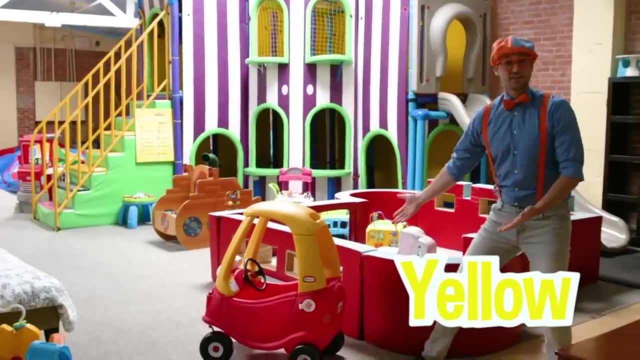 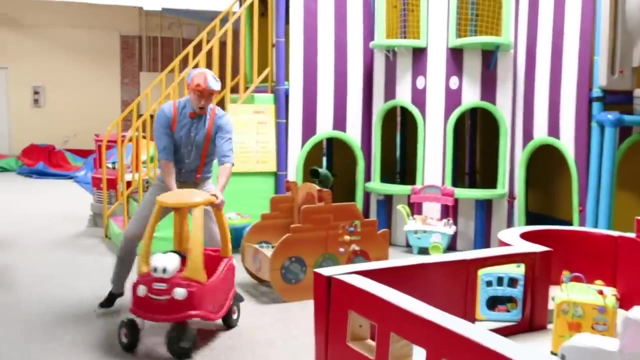 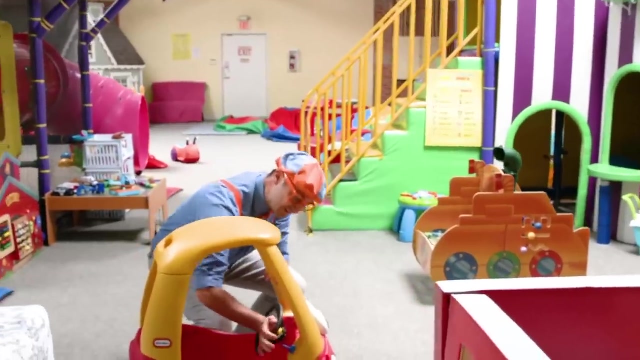 Oh, this is pretty colorful. Whee whee, look at this car. This car is the color yellow and the color red. Here we go. Whee whee, whoa, Whoa, whoa, So silly. 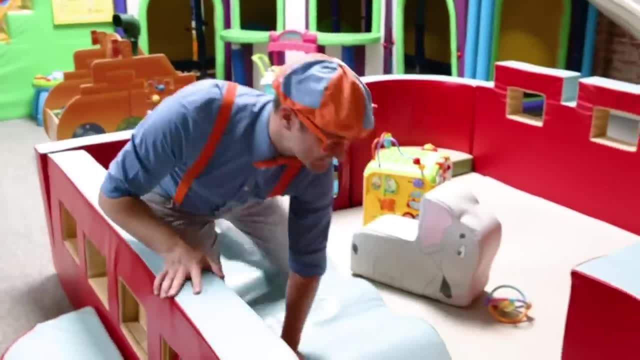 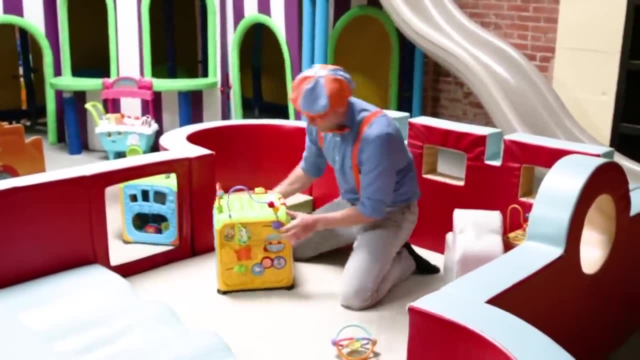 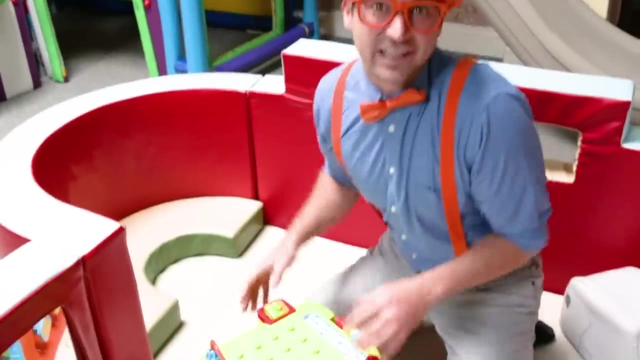 Oh, what's in here? Whoa, it's so soft in here. Whoa, whoa. hey, look at this. This box has so many colors on it. There's so many colors to name. Let's go continue to explore. 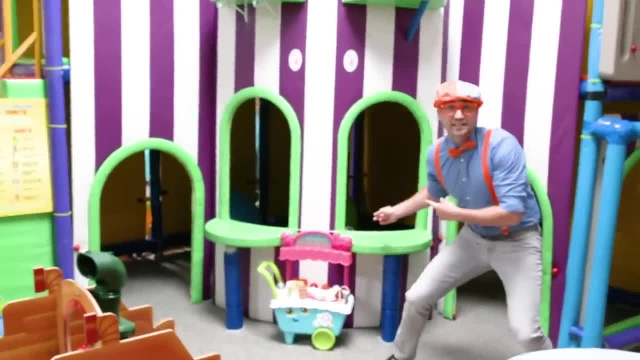 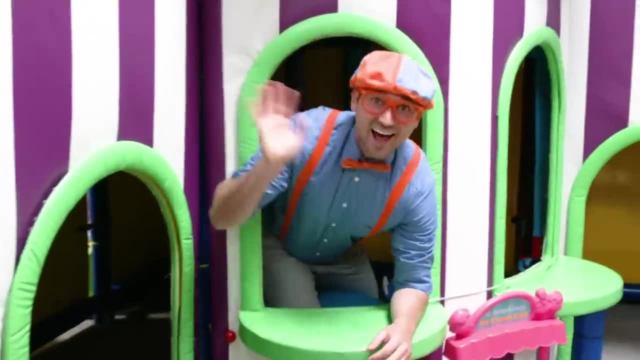 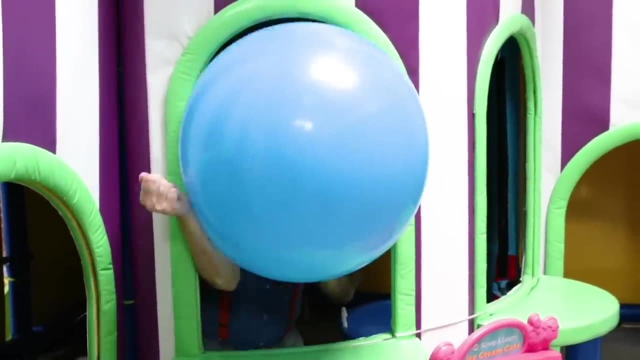 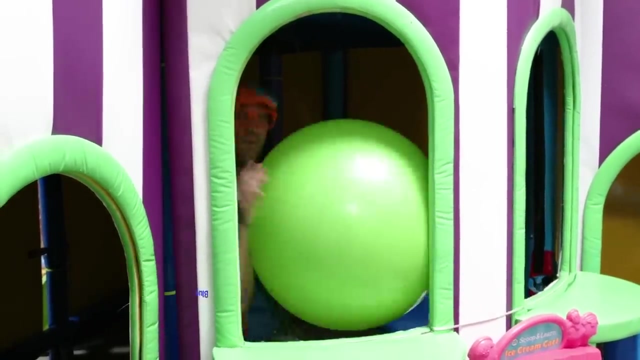 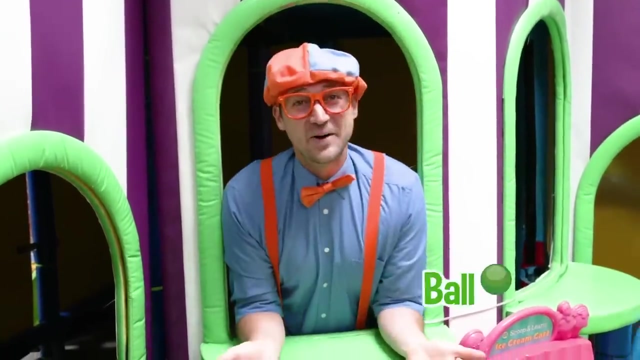 Whoa whoa, it's like a castle. Let me go inside. Hello, Whoa Whoa, check this out. Whoa, that ball was the color blue. Whoa, hey, here's another one. That ball was the color green. 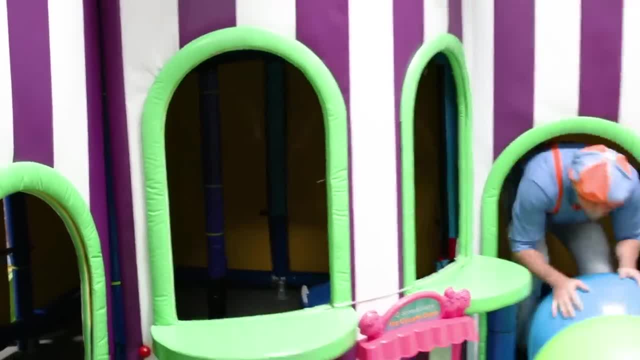 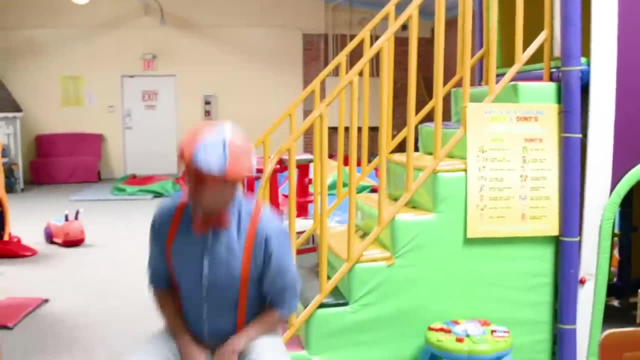 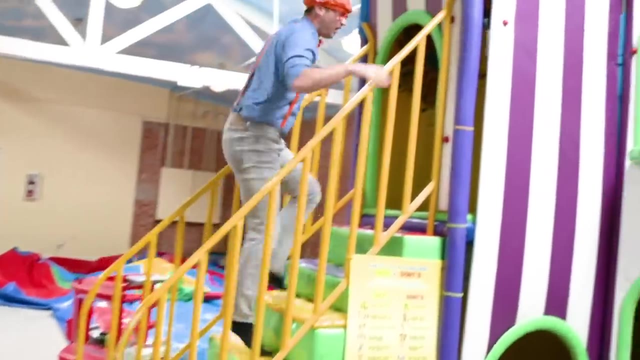 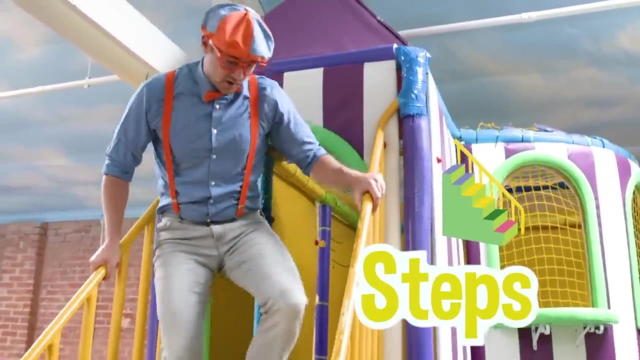 Good job, Whoa, hey, Okay, Boing, Whoa, Whee, Whoa, Whoa. Wow, the castle is so tall. Whoa, hello down there. Hey, Whoa, look at these steps. Wow, do you see the colors? 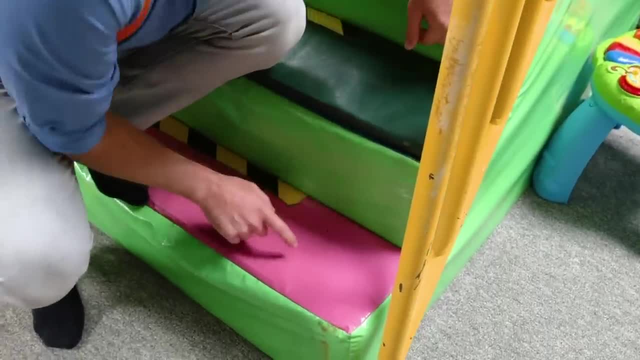 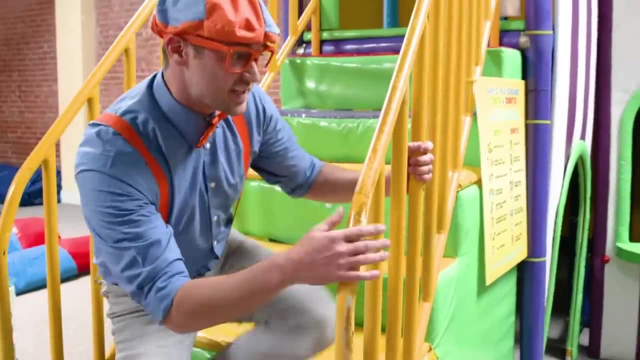 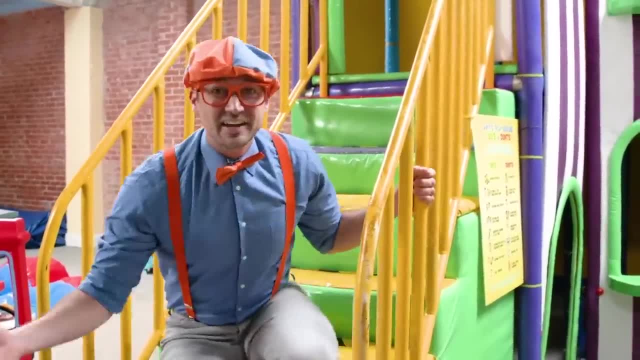 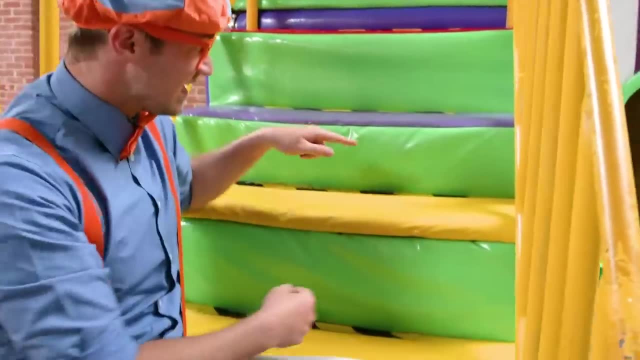 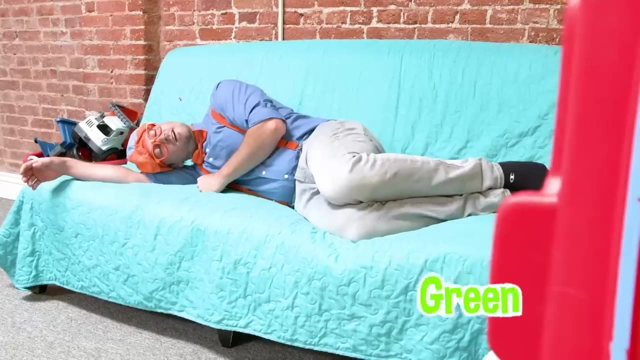 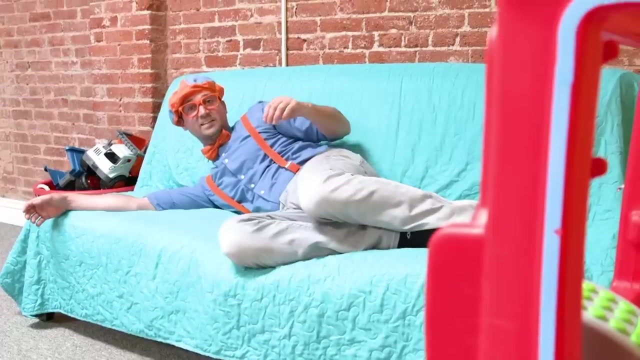 What color is this? Yeah, the color yellow. And right here, we learned this one already. This, this and this- Yeah, these are all. the color green. Wait a second. no time for napping, But this is a nice comfy couch. 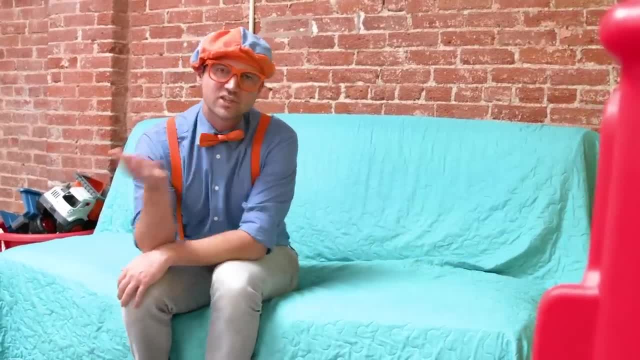 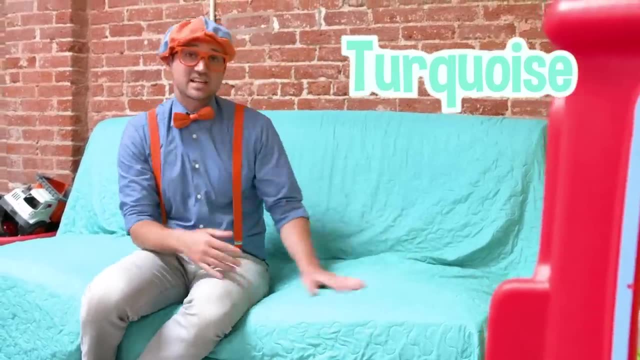 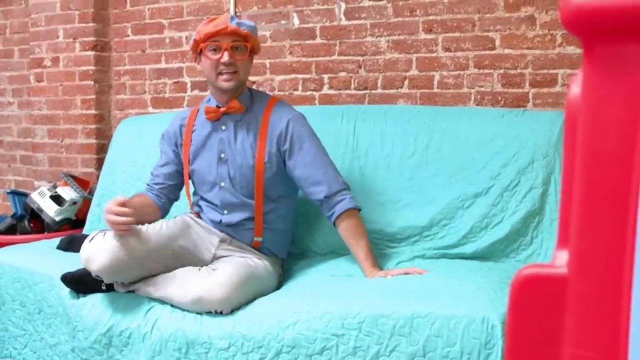 You see what color it is. Hmm, this is an interesting color. This color is the color turquoise. Wow, it's kind of like a blue and a green mixed together. Woo-hoo. But no time for napping, It's time to do some rolling. 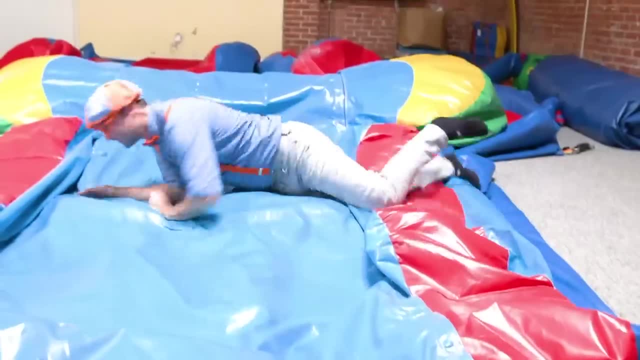 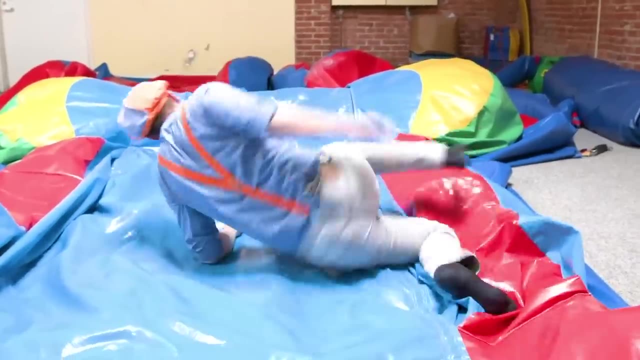 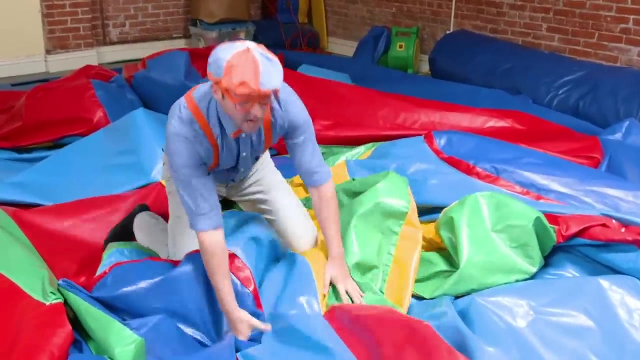 Woo-hoo, Whoa, Whoa, Whoa, Whoa, Whoa, Whoa. I love rolling around. This is so silly, It's so colorful And I think it's deflated. Hmm, How do we inflate this? 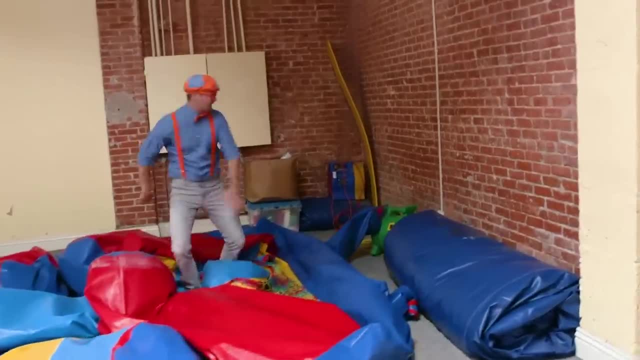 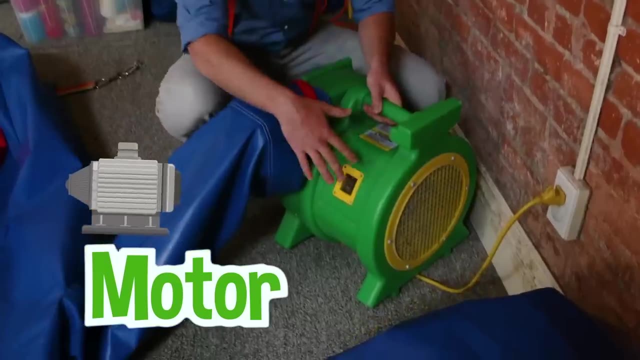 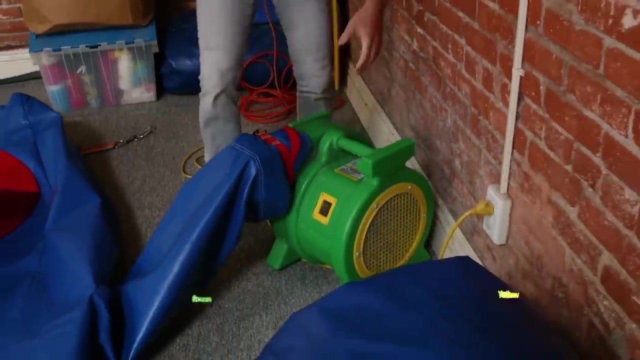 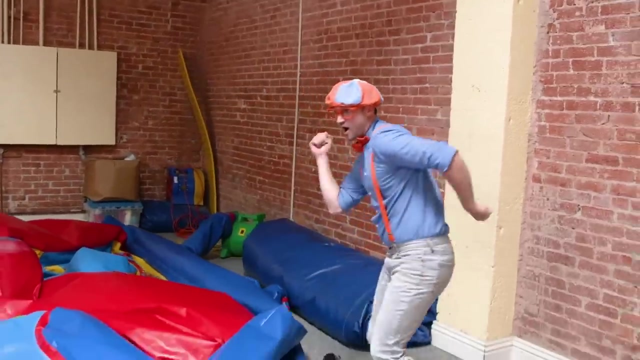 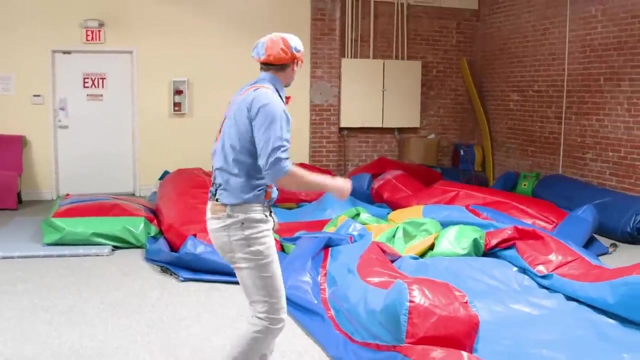 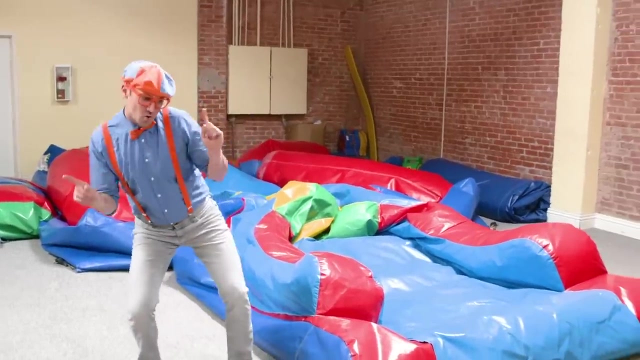 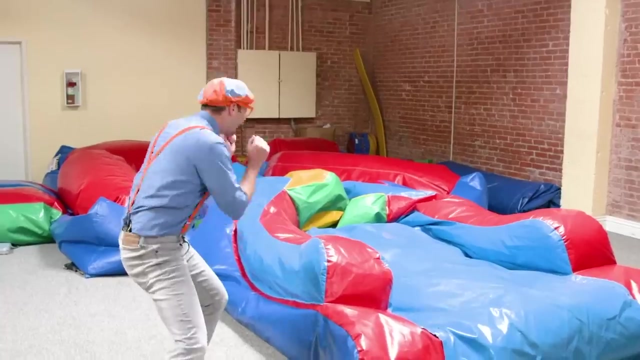 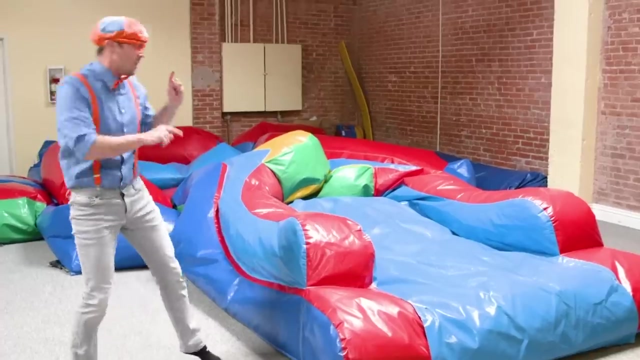 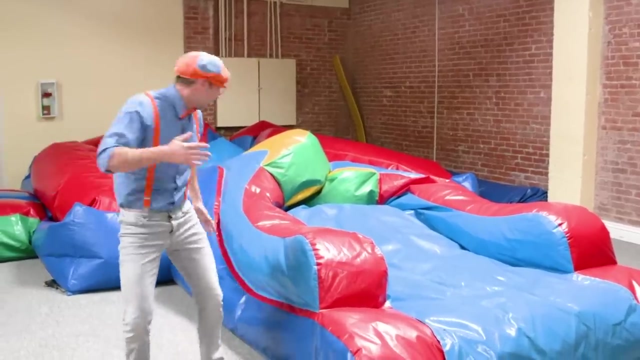 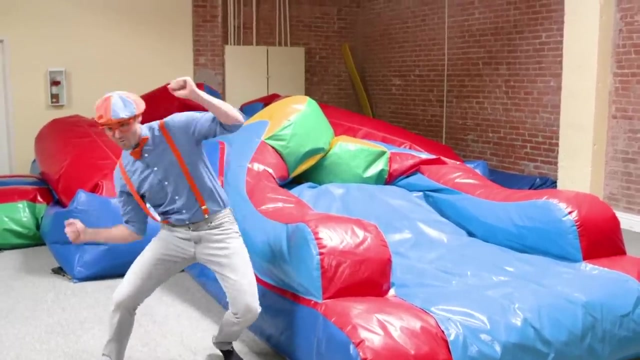 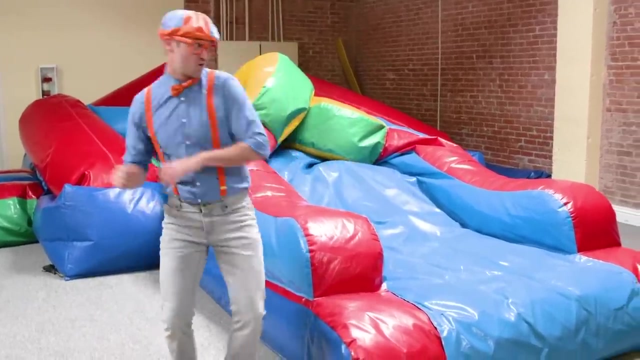 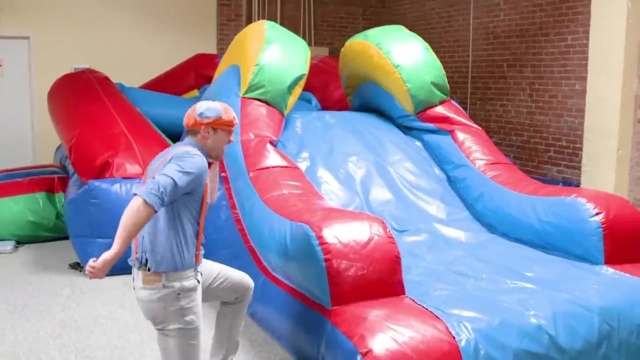 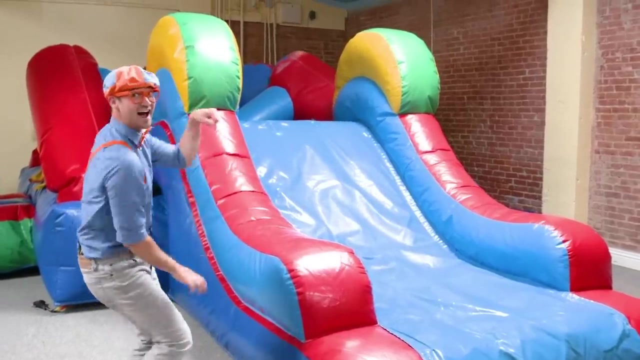 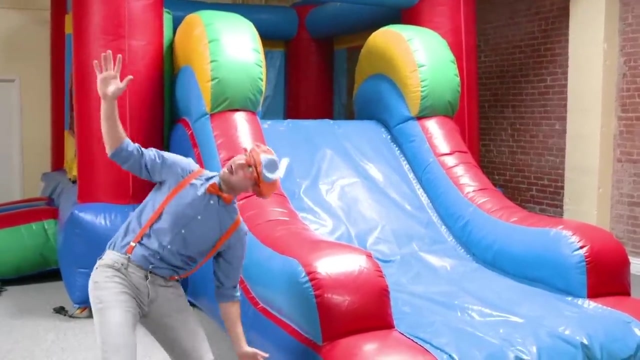 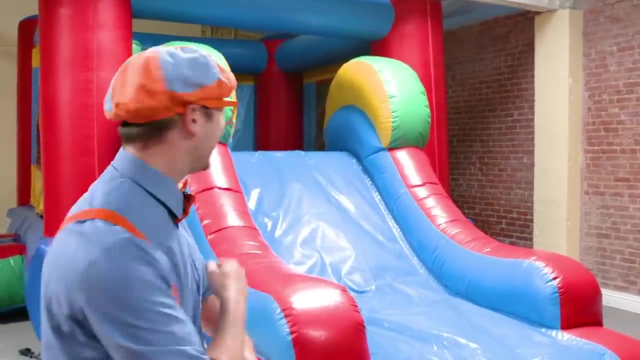 Wait over here. Whoa, This is the green motor. Yeah, this is green and yellow. Here we go. Thanks for watching. Thanks for watching, Whoa, Yeah, We did it. Good job, Woohoo. 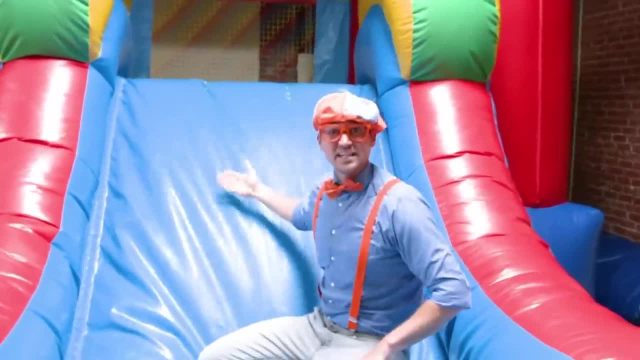 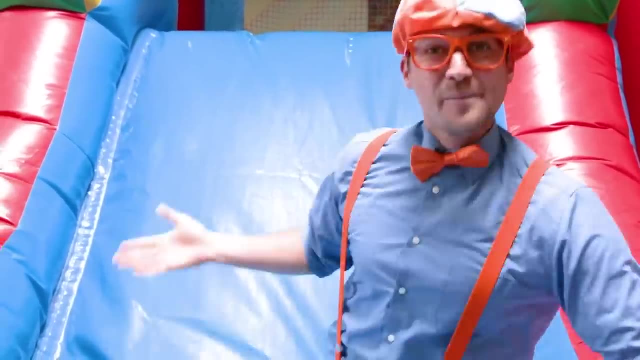 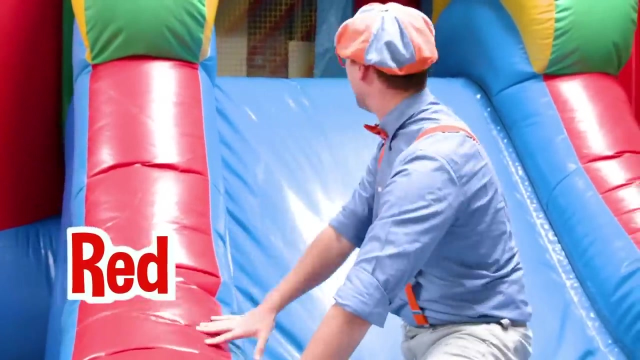 Woohoo, Whoa. What color is this? Yeah, It's one of my two favorite colors. Yeah, And it rhymes with two Blue. And look at this, This is the color red. Alright, Time for me to go down the slide. 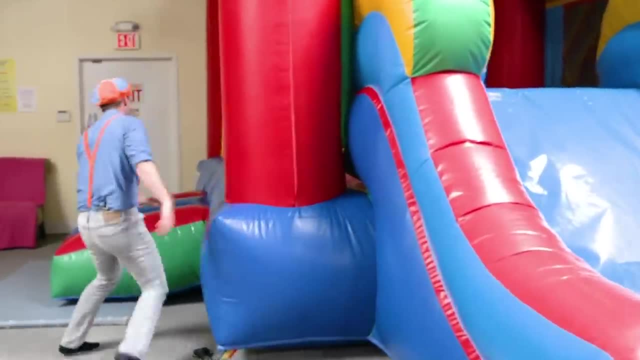 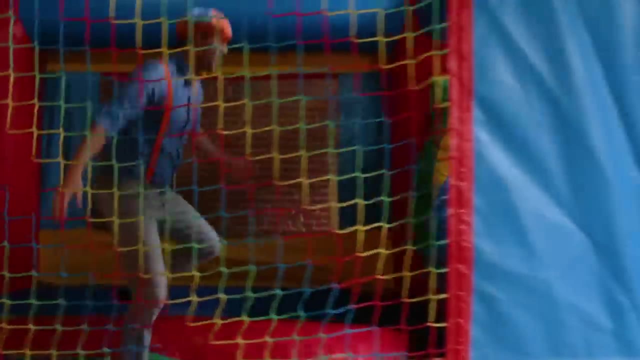 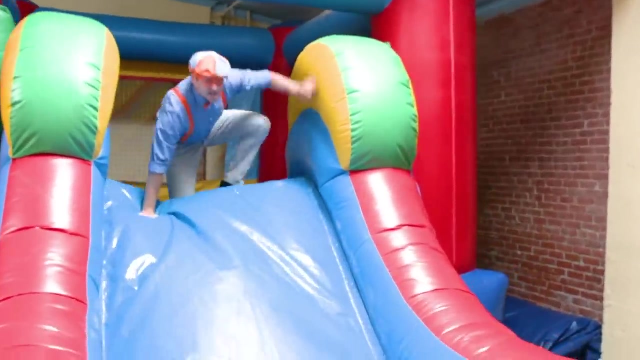 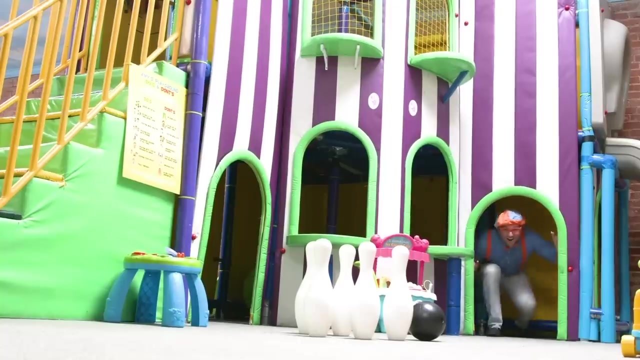 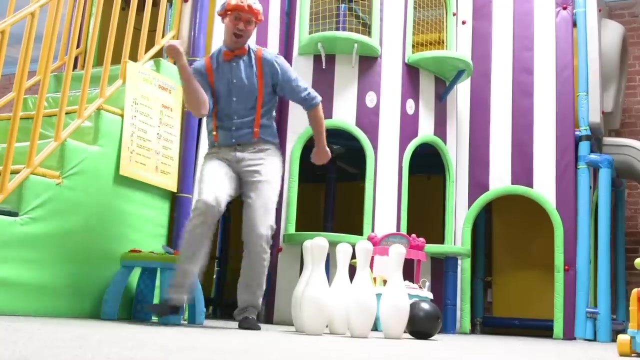 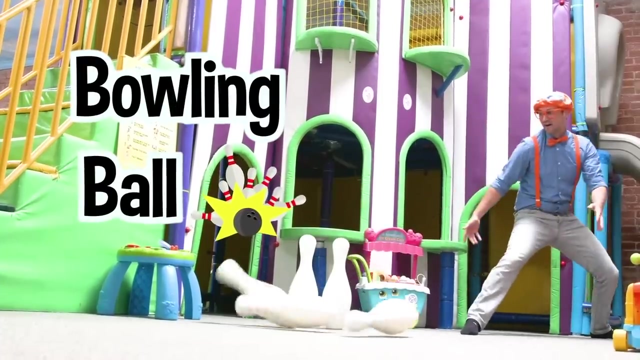 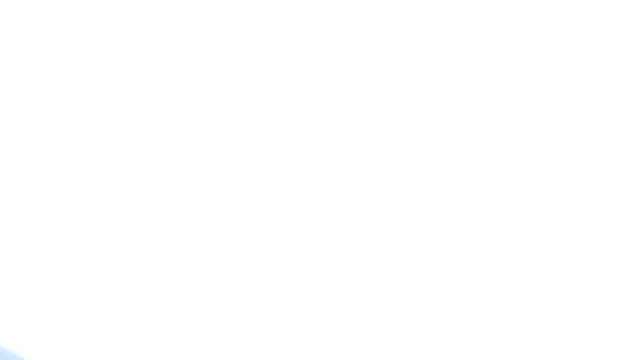 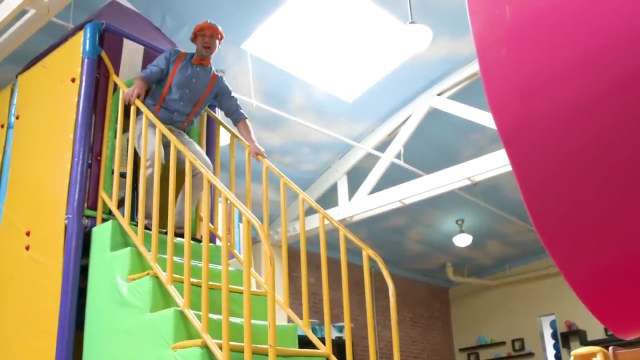 Woohoo, Here we go. Woohoo, Woohoo, Yeah, Hello, Hey, Woohoo. Black bowling ball, White pins- Woohoo, Hey, Hello, down there. Look, I'm at the top of the stairs. 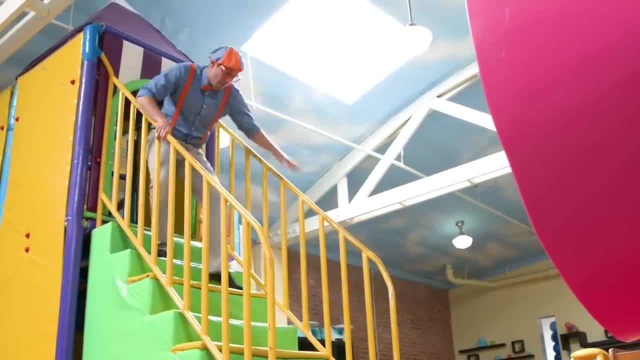 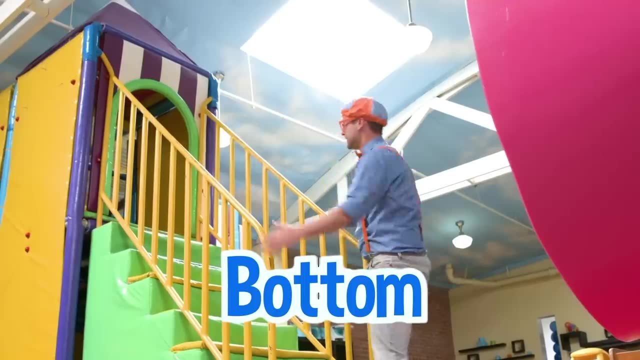 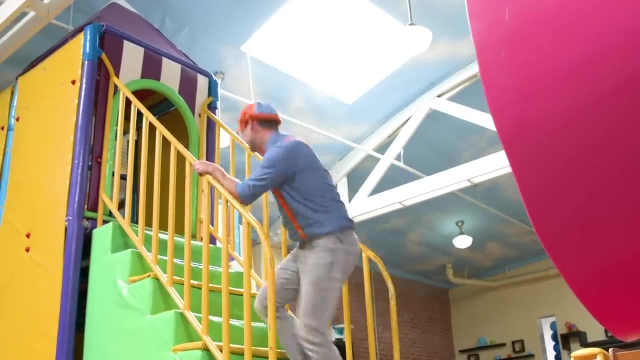 Now I'm going to climb down. Whoa, Whoa. Now I'm at the top of the stairs. I'm at the bottom of the stairs. I should probably climb up to the top of the stairs. Woohoo, Bye-bye. 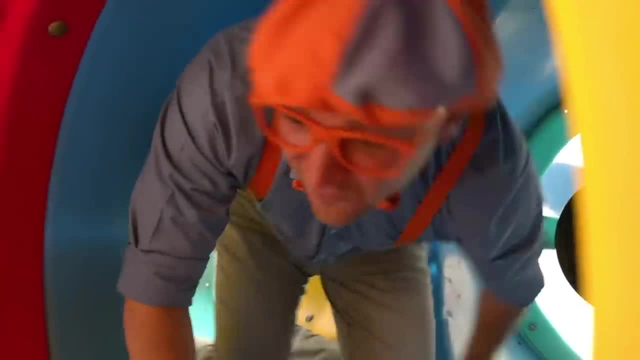 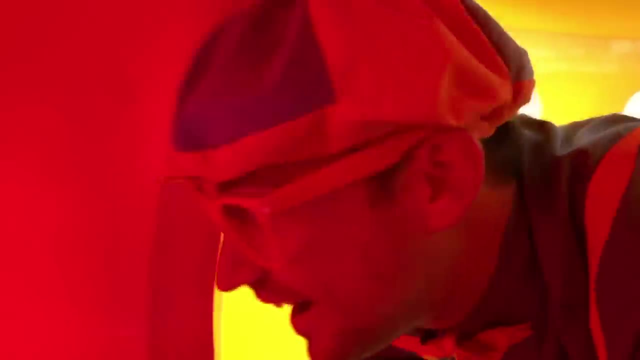 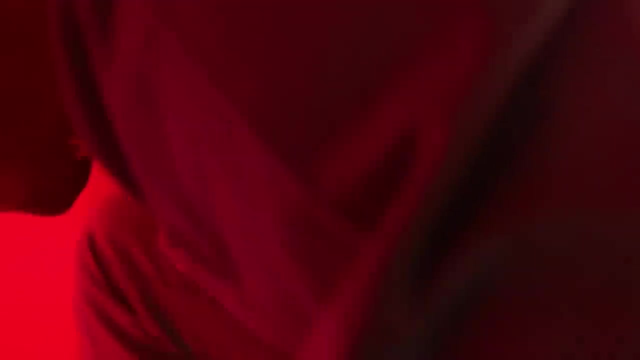 Whoa, It's so colorful in here. Wow, I love crawling through these tunnels. Wow, Okay, A slide. Haha, I love it. I'm excited. Whoo Okay, One, Okay, Are you ready? Three, Two, One. 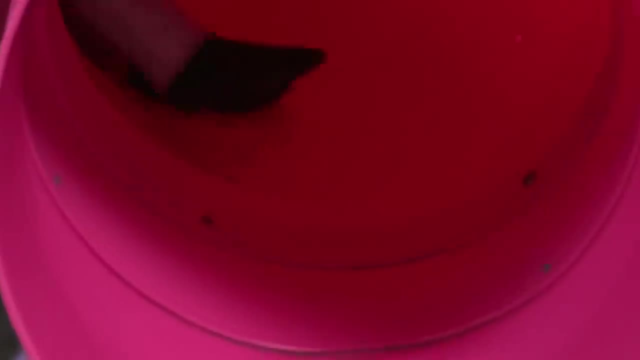 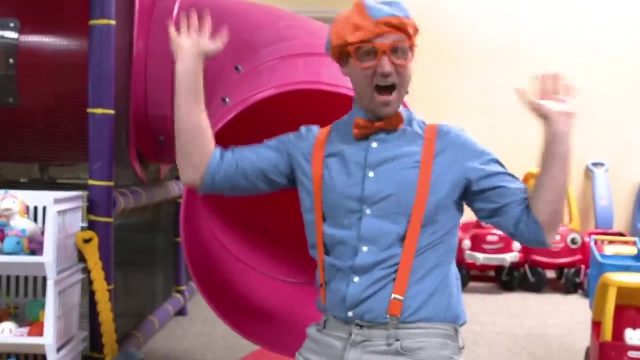 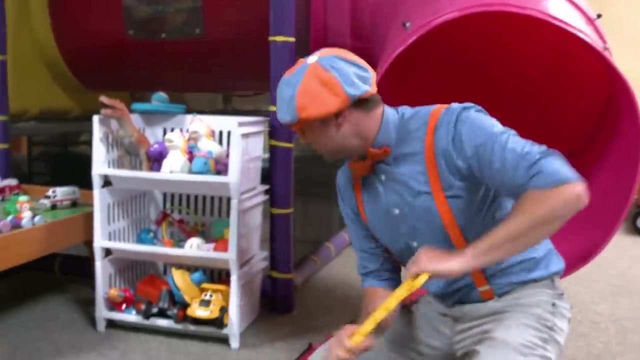 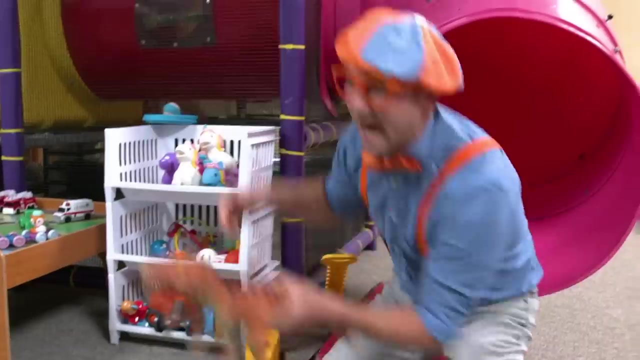 Whoa-oo-hoo, Whoa, Hello, Whoo. This slide was so much fun And it is a pink slide. Wow, What is this? Whee, Whee, Whoa, Whoa, Whoa, Rawr, Rawr, Rawr. 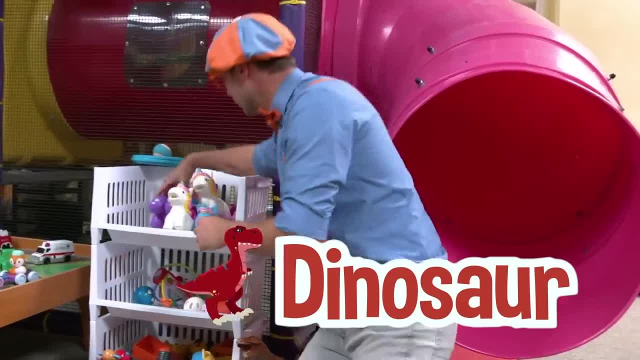 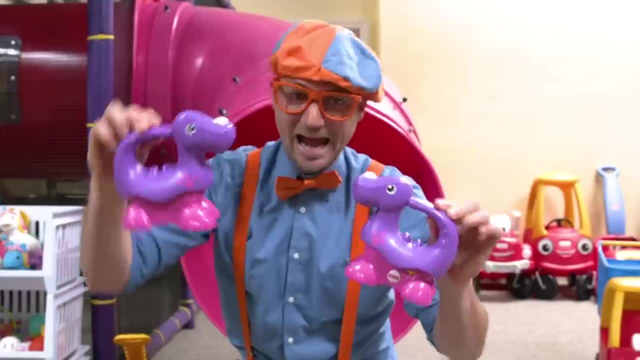 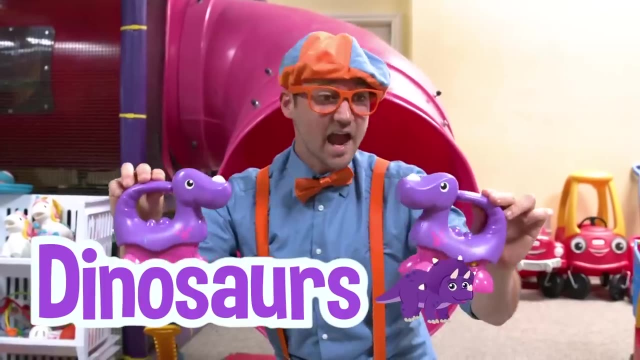 Oh, I love dinosaurs. Oh, and look at these toys. Oh, they're so cute. Hello, Hello, Hi. How are you So silly? What color are these dinosaurs? Yeah, they are the color purple and pink. Whoa. 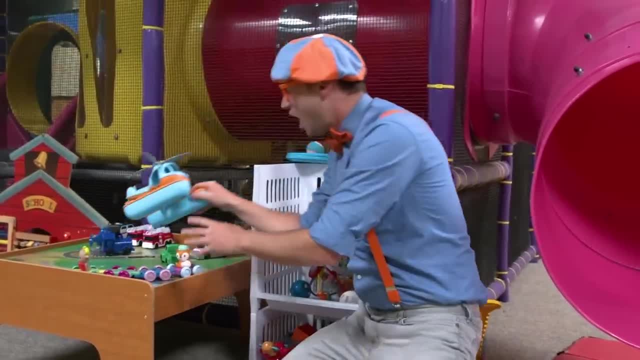 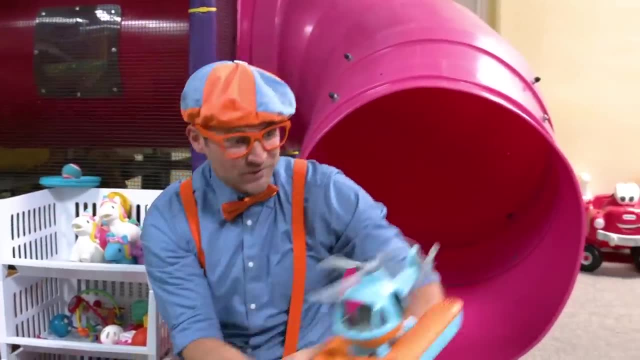 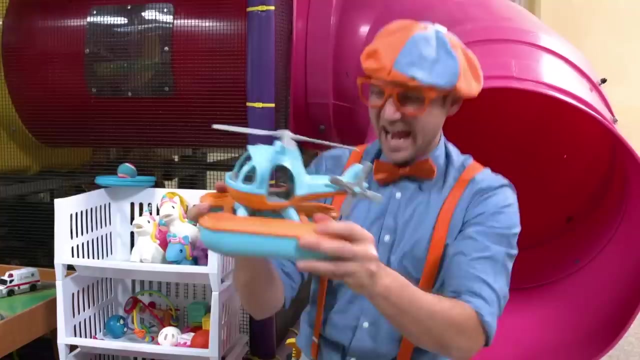 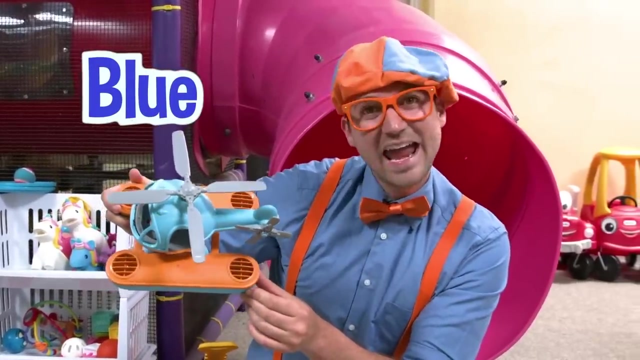 Whoa, Look at this, It's a helicopter And it is my two favorite colors. Yeah, What color is this helicopter? Yeah, there's two colors: Blue and orange. Woohoo, We'll set that back and go explore. 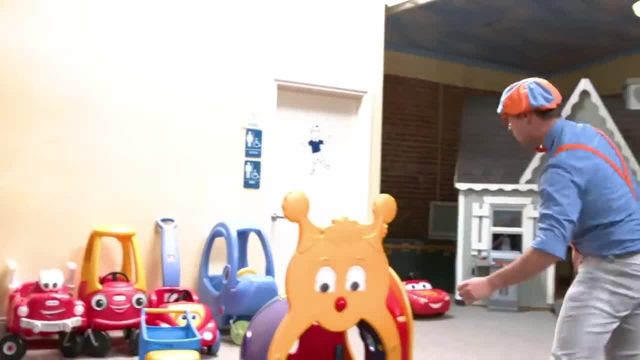 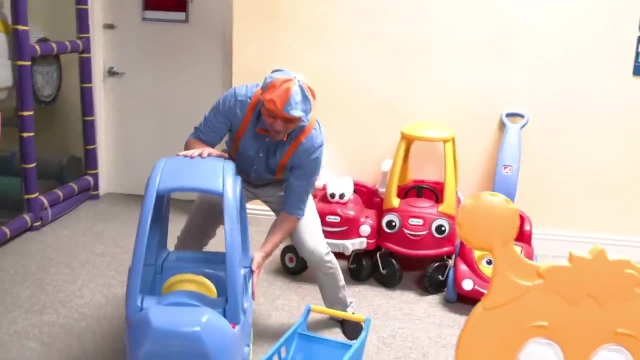 Whoop, Whoop, Whoop, Woohoo, Whoa, Whee Whee, Ha ha Whoa. Look at this light blue car: Whee Whee Whoa. And look at this car. This car looks so fast. 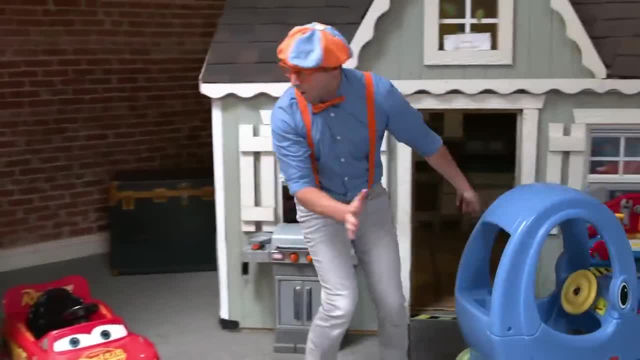 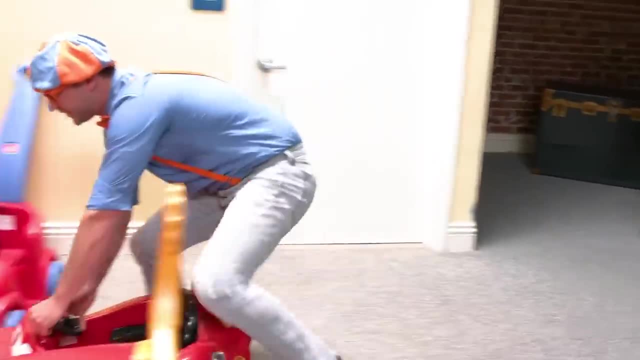 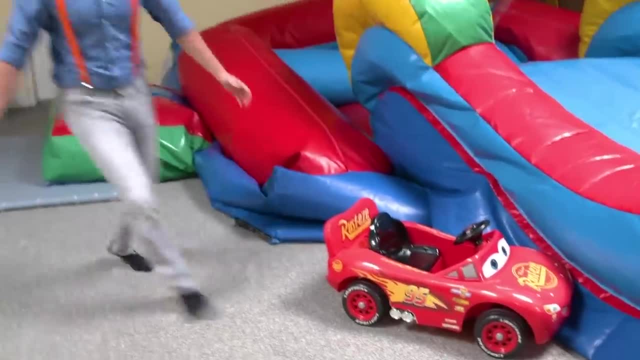 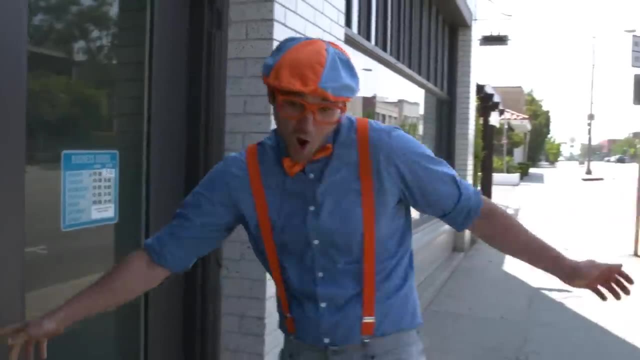 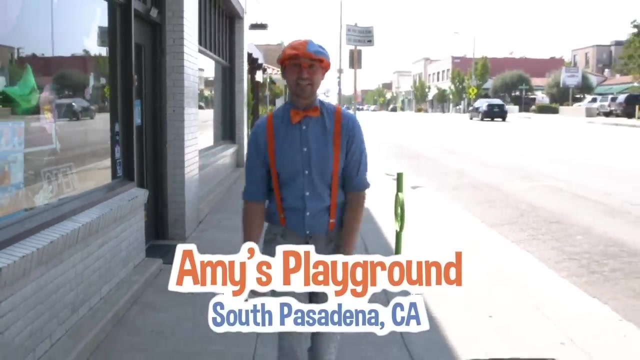 Whee, Ha ha, Whoohoo. I love learning my colors with you. Ha ha, Whoa, Whoa. That was so much fun playing at Amy's playground in South Pasadena, California. Woohoo, I really enjoyed learning about colors with you today. 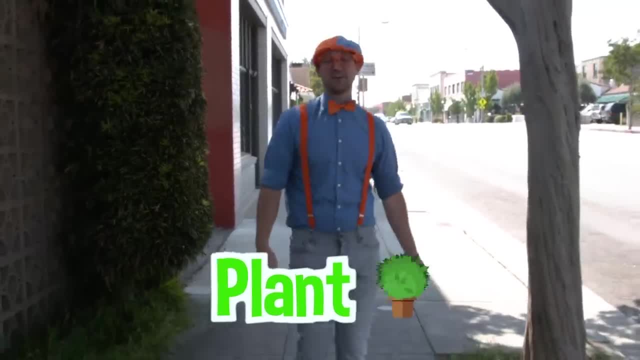 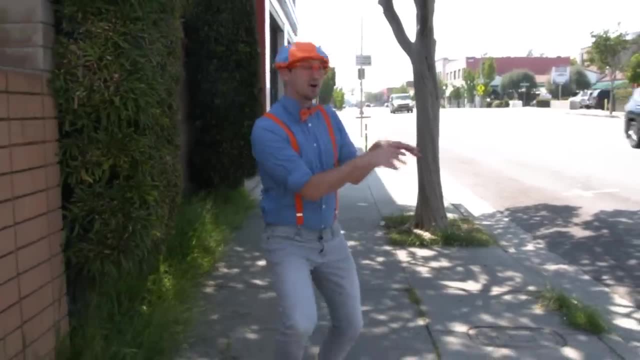 Hey, like this green plant. That was so much fun. Well, this is the end of this video, But if you want to watch more of my videos, all you have to do is search for my name. Will you spell my name with me? 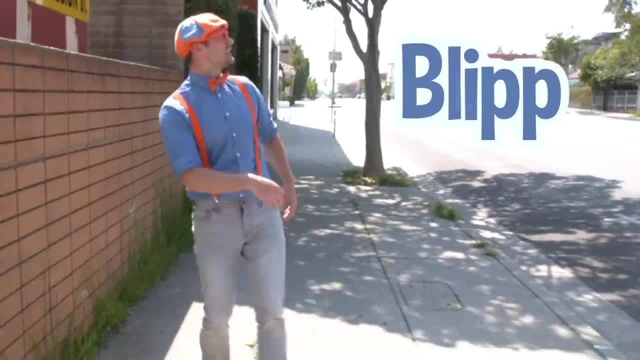 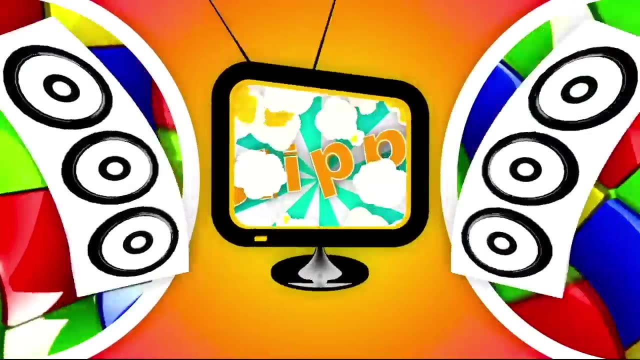 Ready B-L-I-P-P-I- Blippi, Good job, All right, see you later. There's so much to learn about. It'll make you want to shout: Blippi. Hello, Hey, it's me, Blippi. 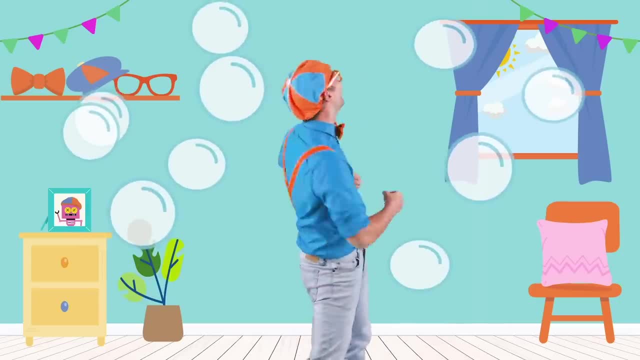 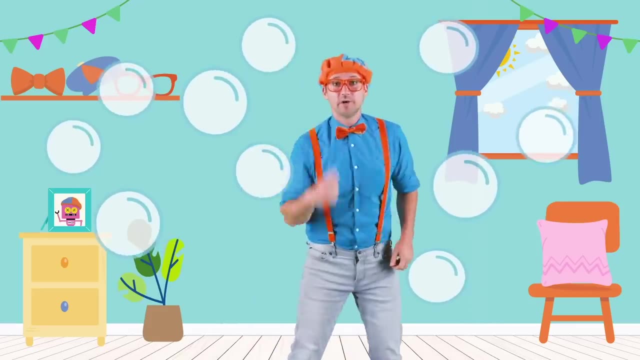 I'm just hanging out with all of these bubbles. I sure do love bubbles, Do you? Yeah? Well, in this video, you and I are going to meet someone really cool that knows a lot about bubbles. Are you ready? Let's go. 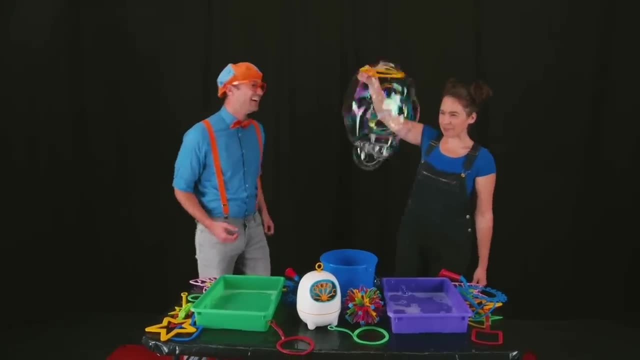 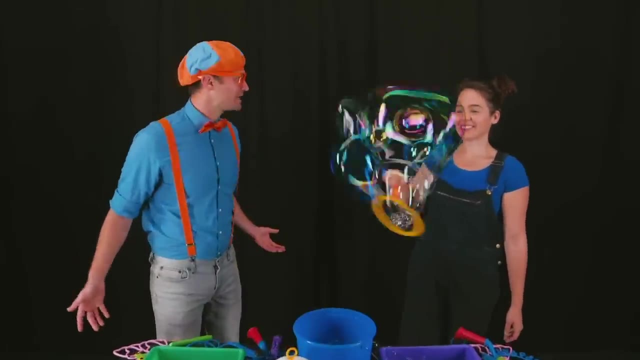 Wow, that is so cool. Thanks, Blippi. Yeah, Wait, who are you? Oh well, I'm Megan the Bubble-ologist. Bubble-ologist, What does that mean? Well, I make all types of bubbles. Oh, bubbles. 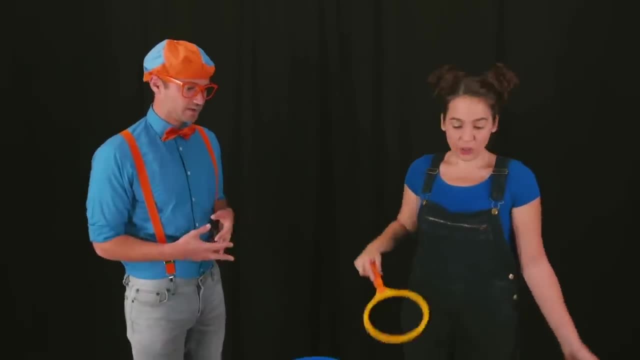 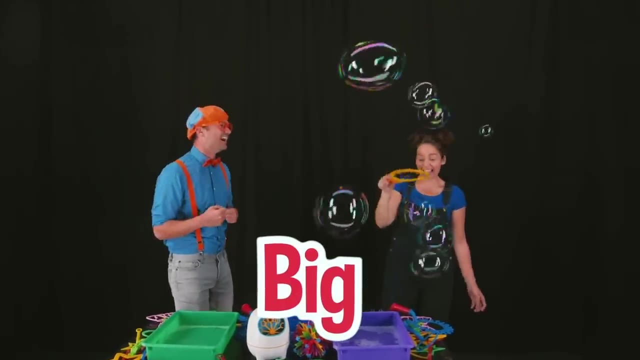 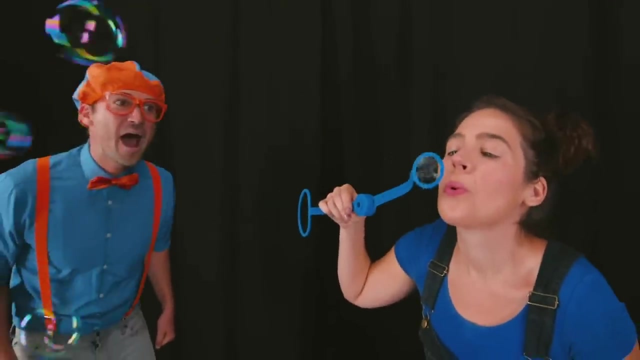 I love bubbles, Like: will you show me one? Sure, I can make big bubbles. Wow, That is a big bubble. I can also make small bubbles. Really, Mm-hmm, I'm so excited, Wow Look. 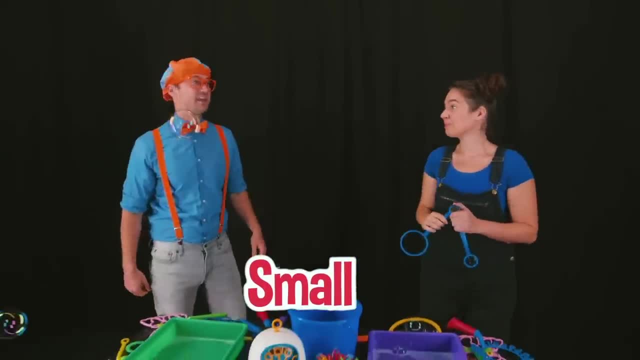 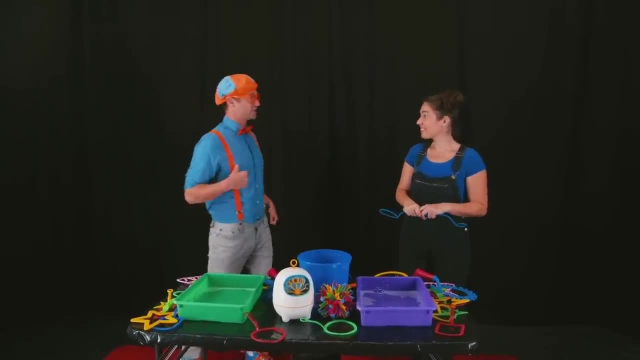 Those are small bubbles. Megan just made big bubbles and small bubbles. Wow, That is so cool. Can I try, Of course? Oh, all right, What do I do? Well, you can take any bubble wand that you want to use. 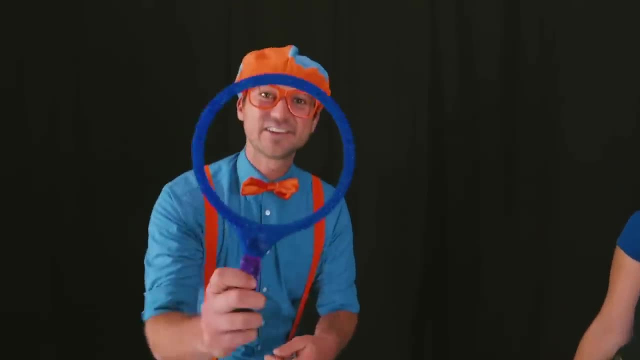 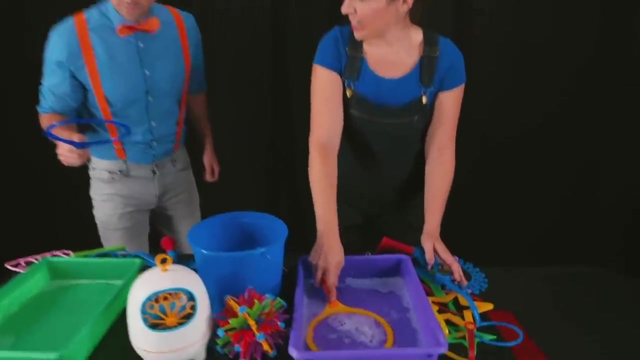 Okay, How about this one? Wow, This one is a big circle. Hello, All right. Now what? Well, you just stick it all the way into the bubble. solution, Okay, And make sure it gets really wet. Okay, Here we go. 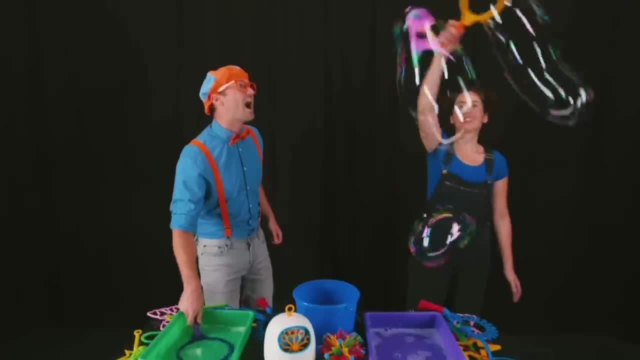 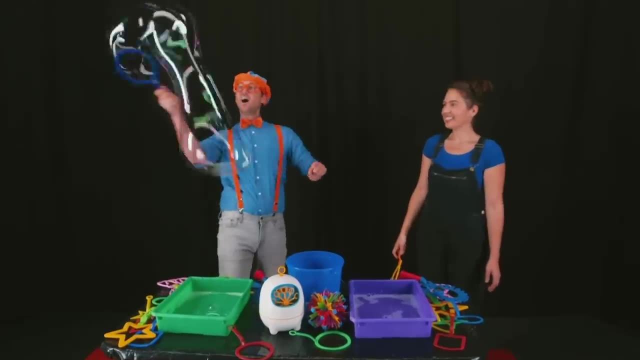 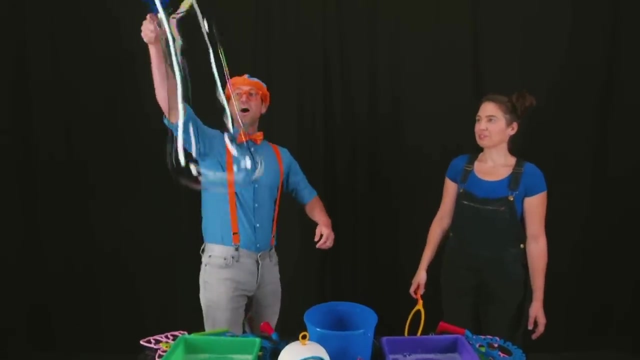 And then pull it out and wave it around. Wow, That is awesome. My turn: Three, two, one, Whoa. It just popped Here we go. Three, two, one, Whoa. I did it again. This is awesome. 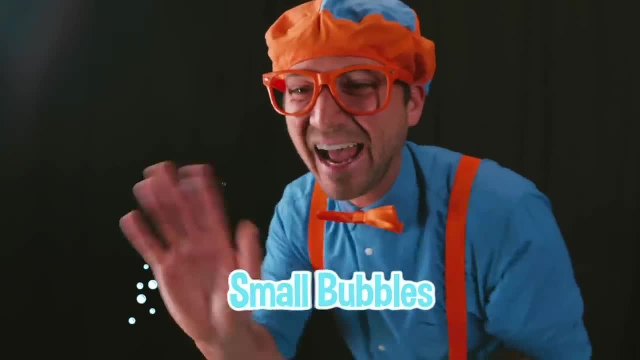 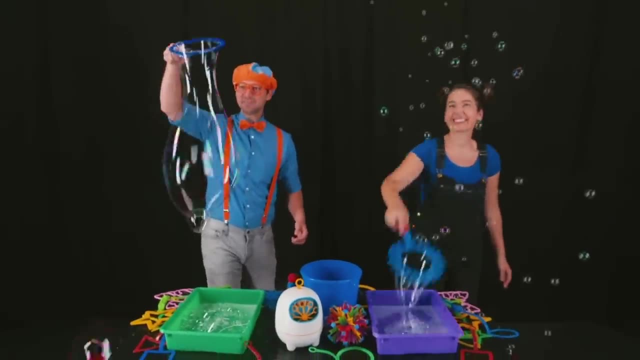 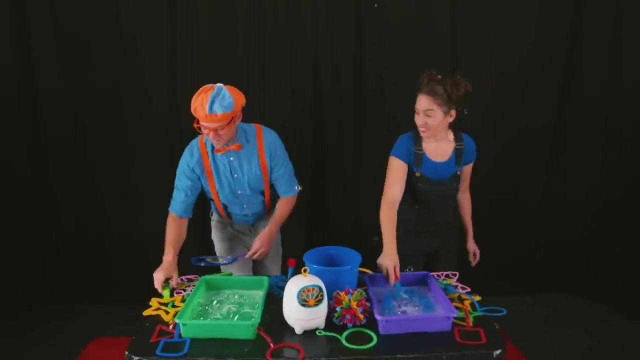 Wow, That is a small bubble. I love making bubbles. It's so cool that all this equipment is so colorful. Oh, like this one. This is the color yellow and green. This one is red and blue. Wow, That is so cool. 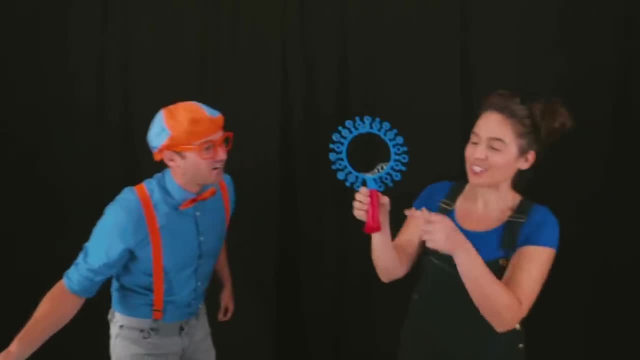 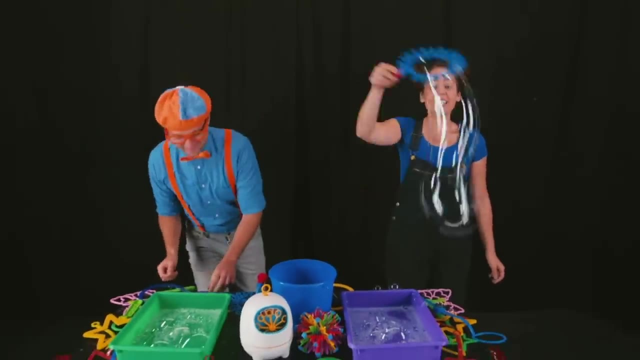 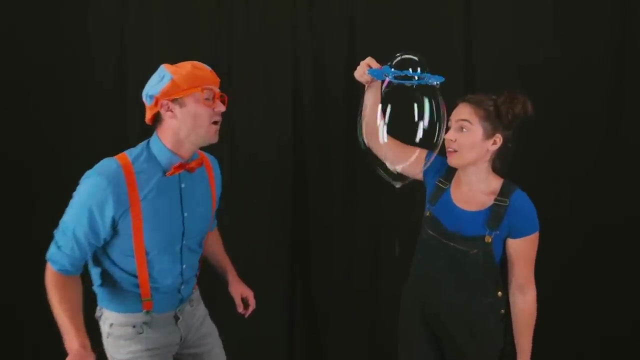 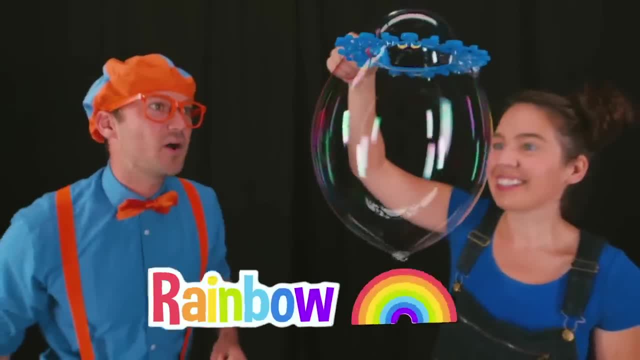 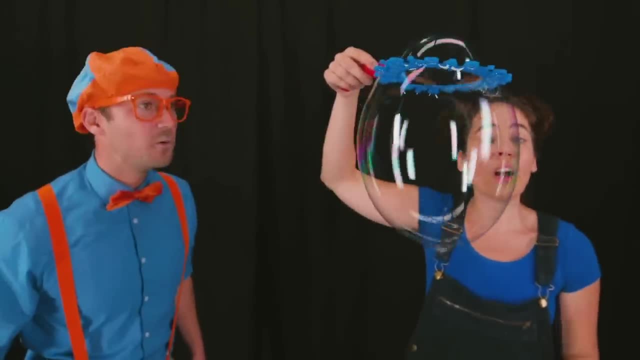 Oh yeah, I see it. It kind of looks like a rainbow. How does that work Exactly? Well, the light shines on the bubble and refracts, So then you see all the different colors of the rainbow. Wow, I love rainbows. 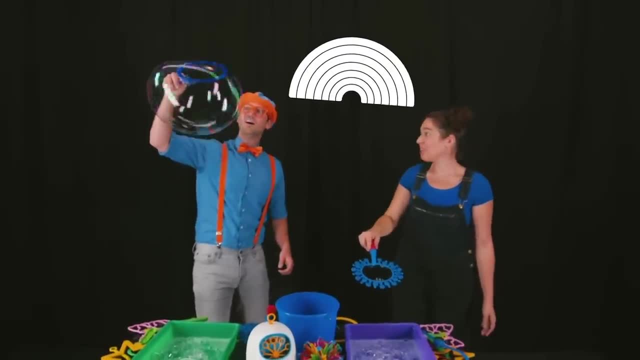 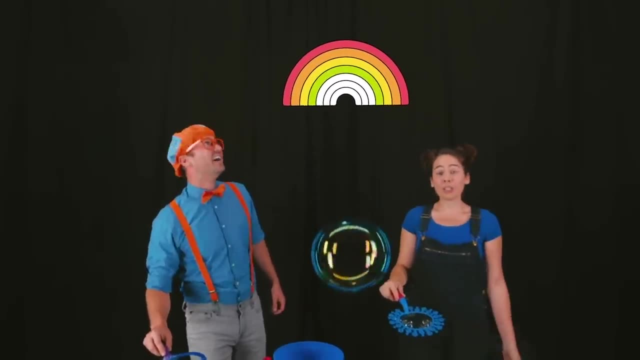 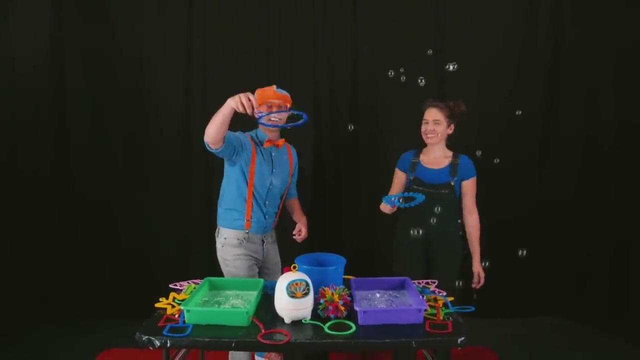 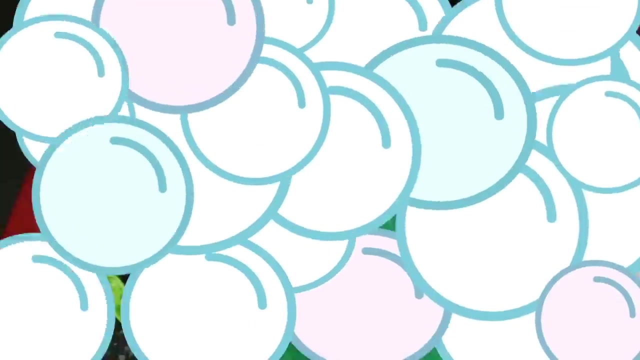 Do you know the colors of the rainbow? I sure do. They are red, orange, yellow, green, blue, indigo and violet. Woohoo Colors, Rainbows and bubbles. Whoa Wee, This wand is a triangle. 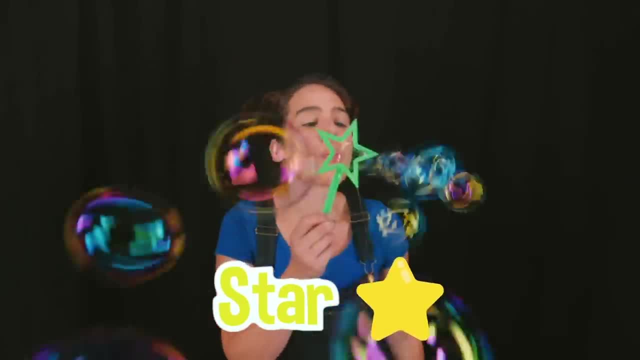 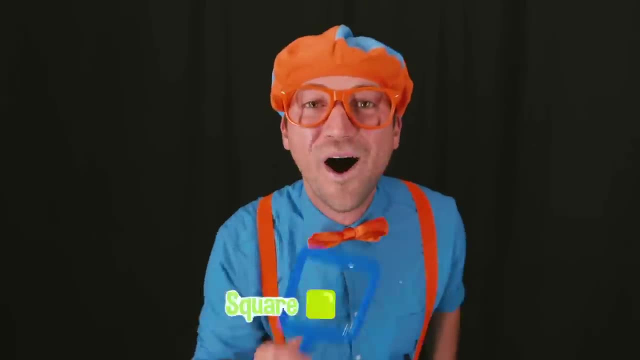 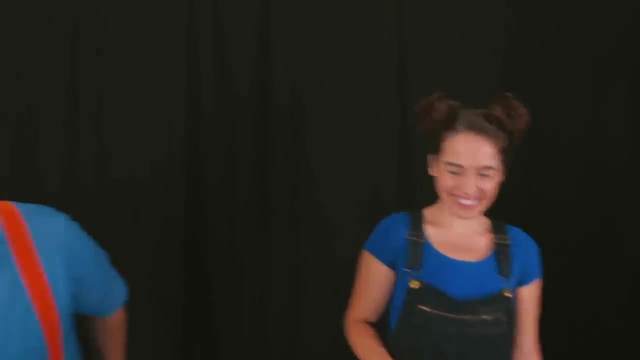 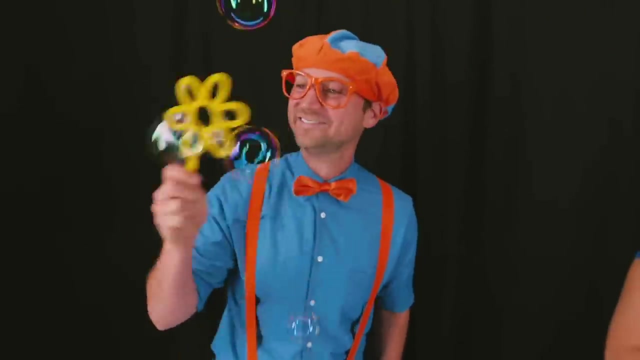 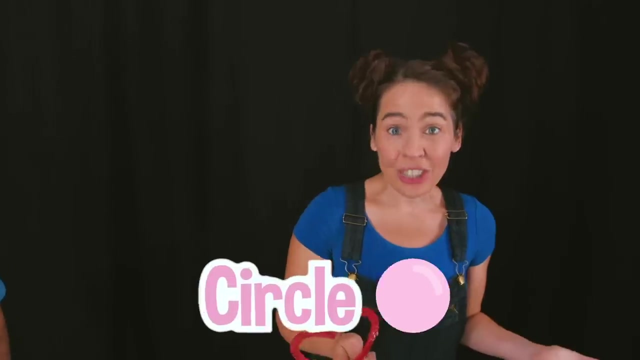 This wand is a star, This wand is a square, This wand is a heart And this wand is a flower. Did you notice that all the bubbles that we made were circle-shaped bubbles, Really? Why is that? Because no matter what shape you use, 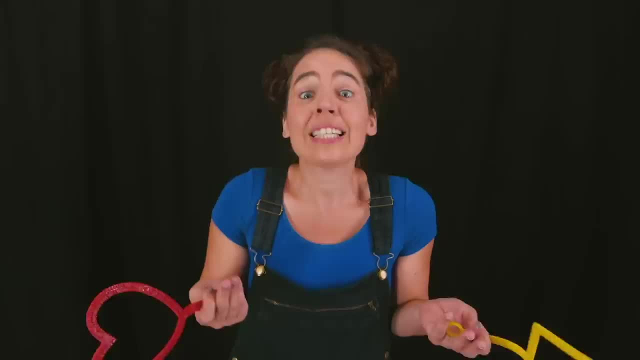 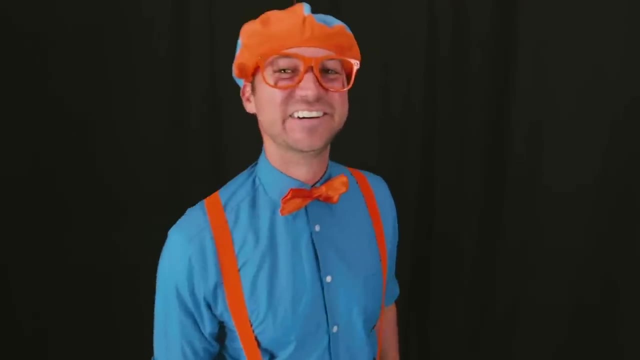 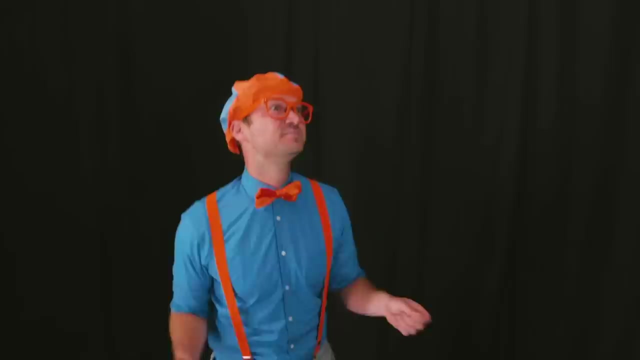 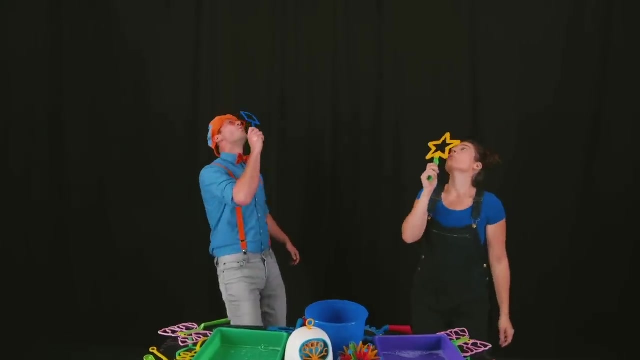 a bubble is always going to be a circle-shaped bubble, because a circle is the most efficient shape a bubble can make. Oh, that makes sense now. That is so cool, But wait a second, Unless you use bubble magic, of course. See you all later. 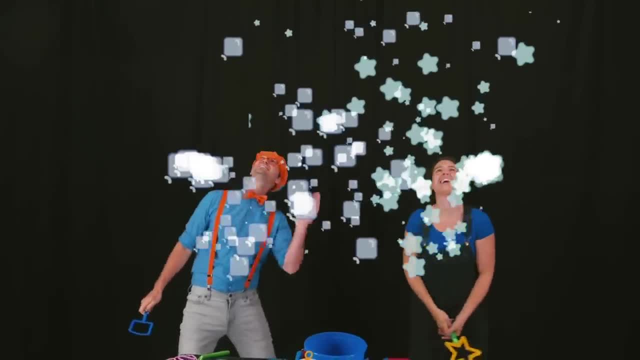 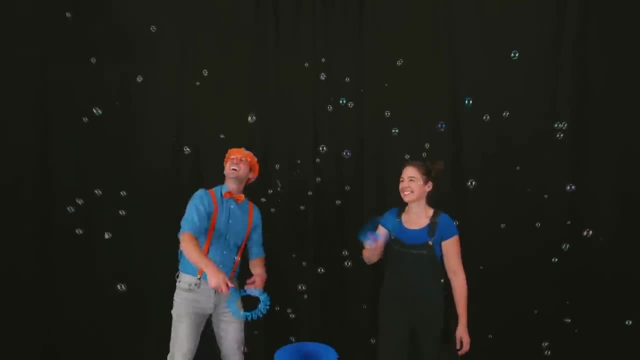 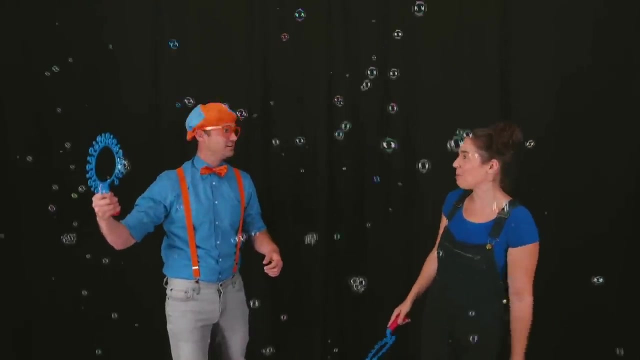 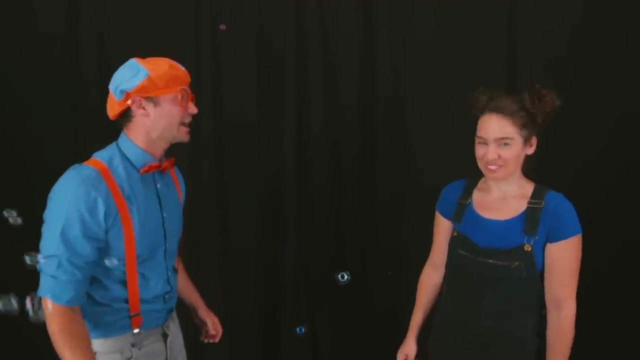 Bye, Wow, See you later. Bye, bye, Wow. Hey, I have a special bubble for you. Really, What do you mean by special? Well, I can make an insect bubble. Wow, really, What kind of insect. Okay, I'm ready. 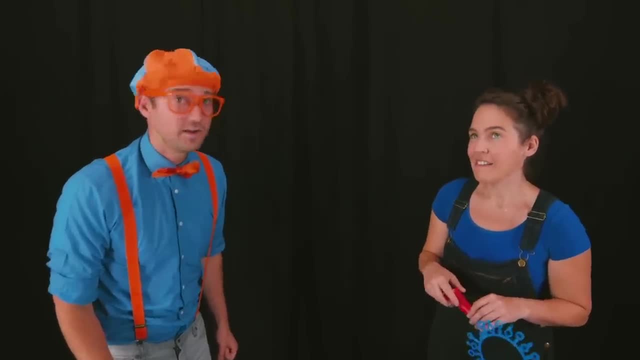 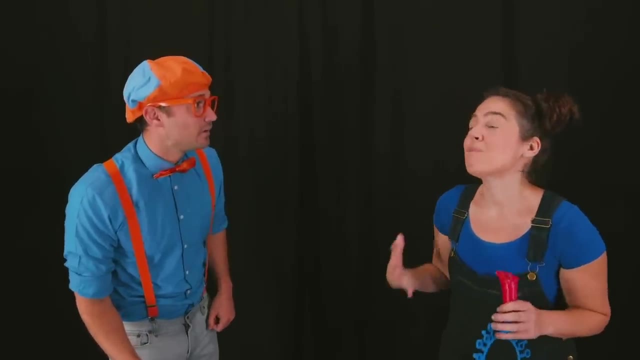 Let's see. It likes to crawl on the ground. Okay, It likes to eat vegetables. Hmm, I love vegetables. Also, it goes through a metamorphosis later in life- Metamorphosis- I know what insect that is. 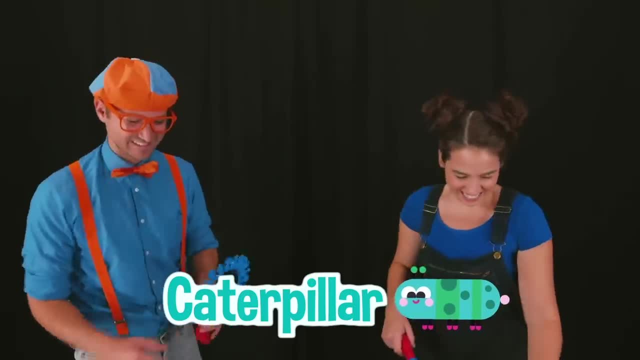 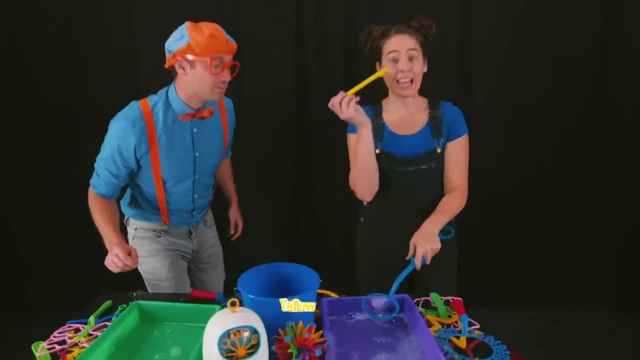 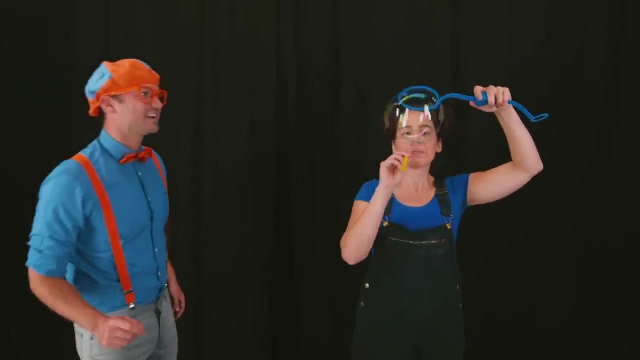 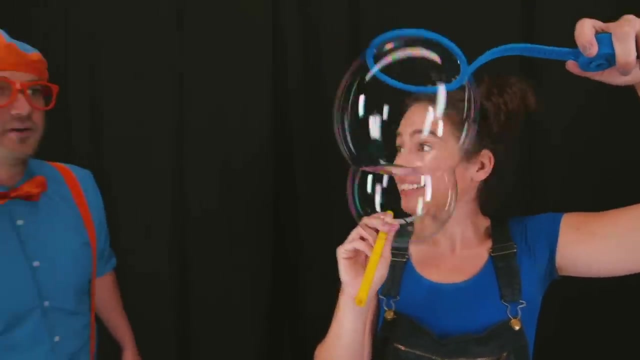 Yeah, that is a caterpillar. You got it Flippy. Okay, let's see this bubble. All right, well, first I need my blue circle wand and my yellow straw. Wow, Oop, Perfect, Wow, So it looks like you're putting one circle bubble on top of the other circle bubble. 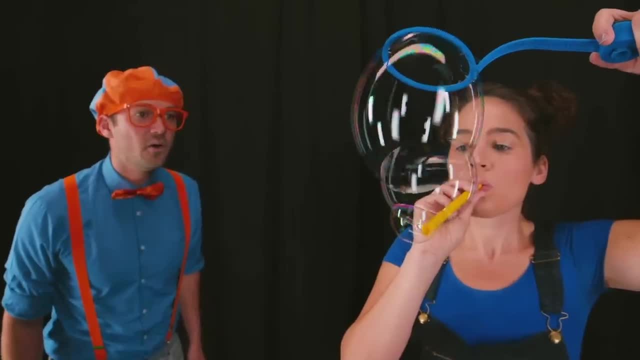 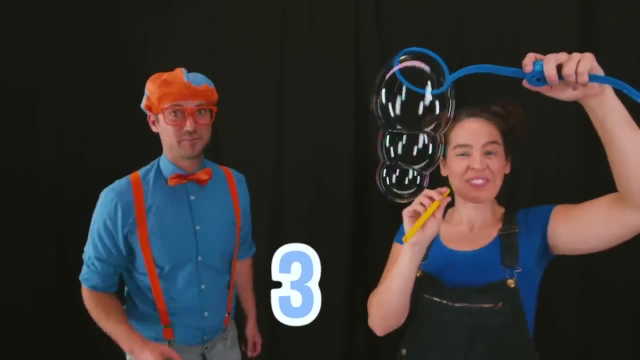 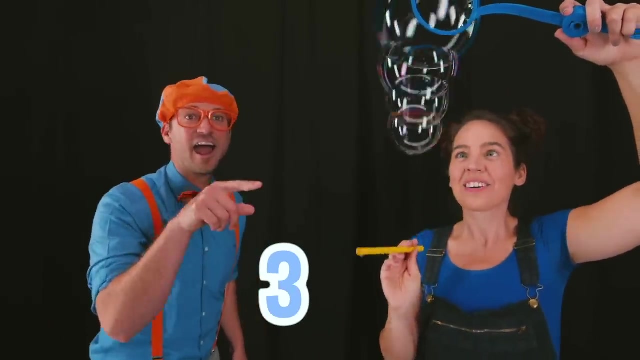 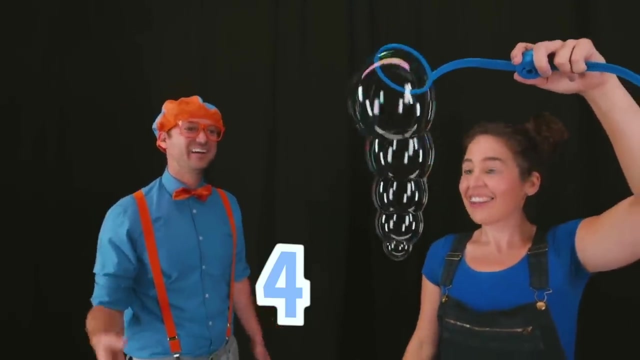 That's right, Okay, Another circle bubble. So we have three circle bubbles connected right now: One, two, three, four, Wow. And another one Five circle. well, four circle bubbles now. That's cool, Wow. 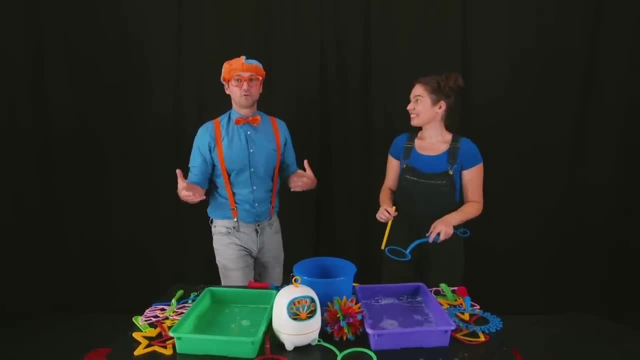 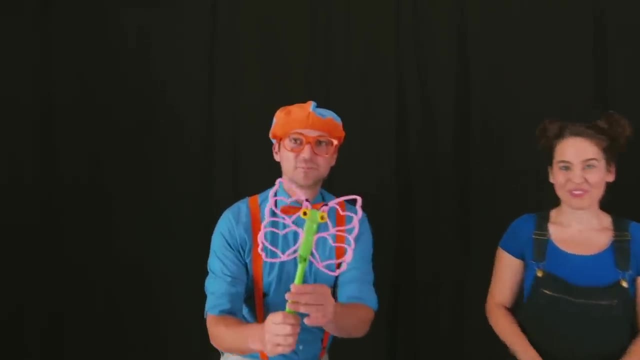 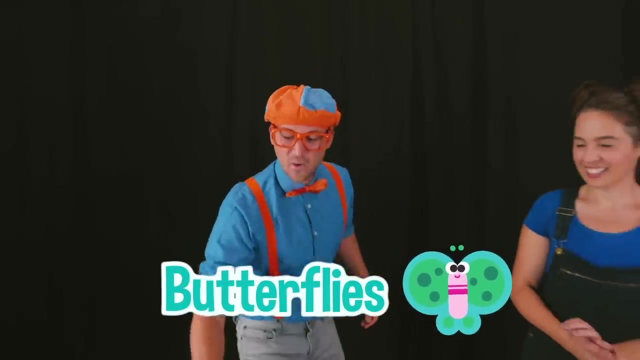 I think caterpillars are really cool because they go through metamorphosis. Hey, I saw What insect it turns into. Yeah, After metamorphosis they turn into butterflies. Here we go. Woo-hoo, Butterfly bubbles, Caterpillar bubbles. 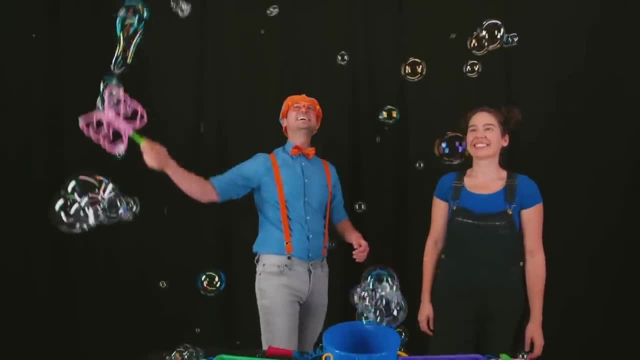 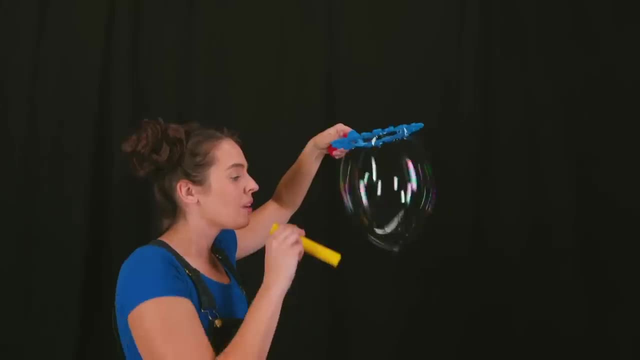 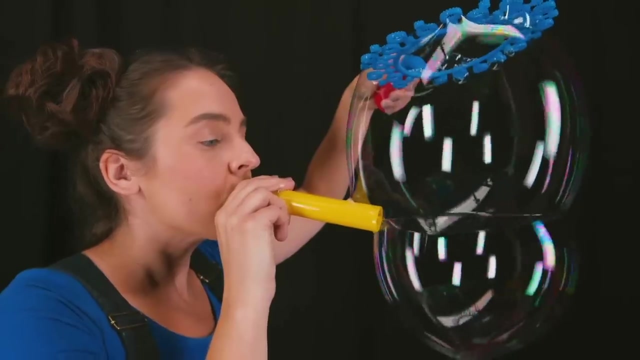 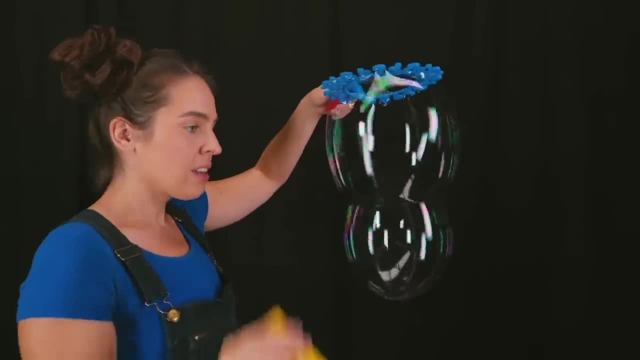 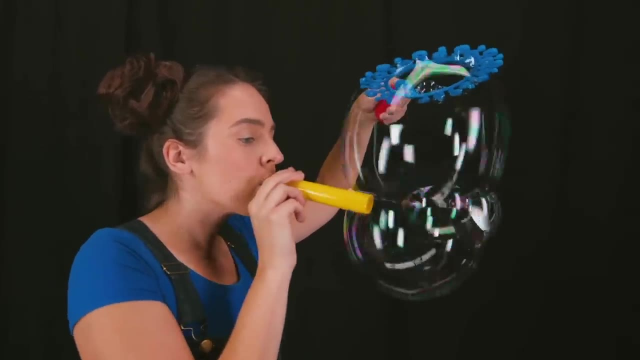 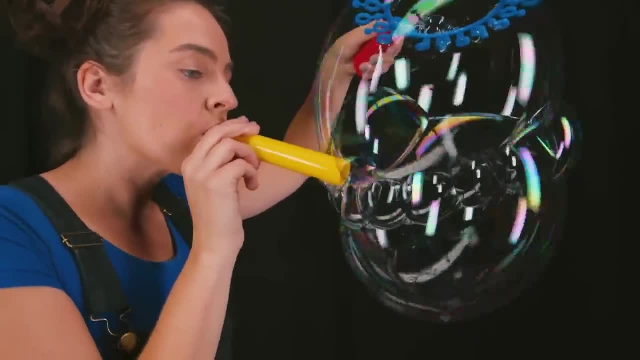 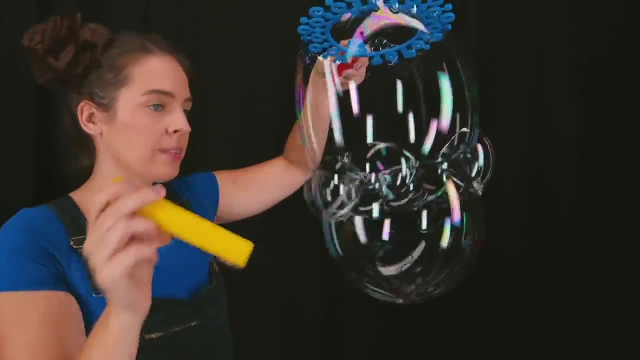 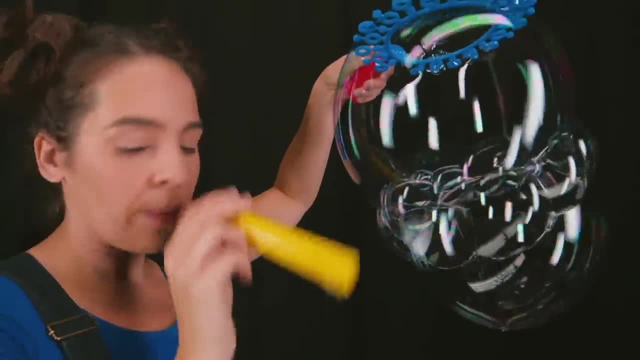 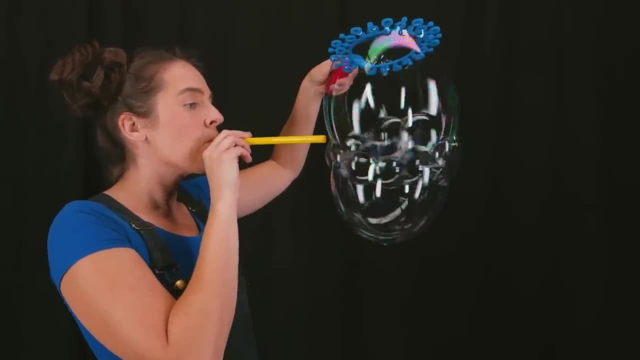 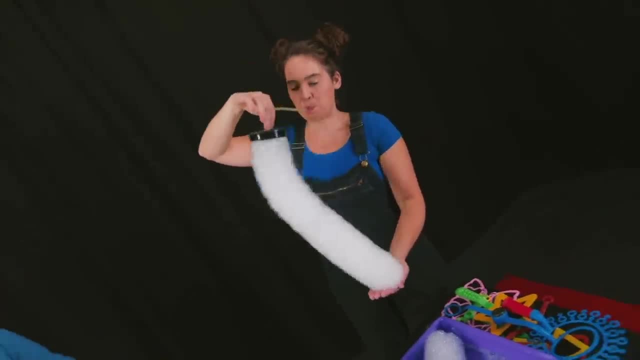 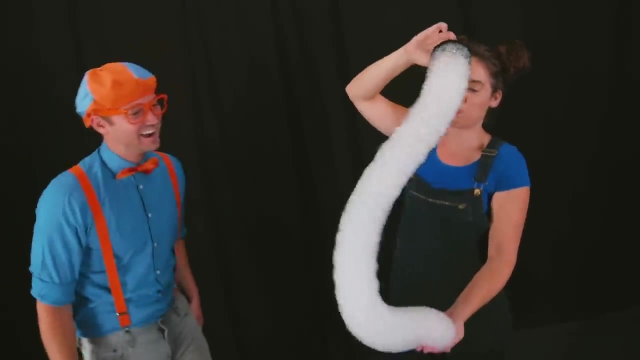 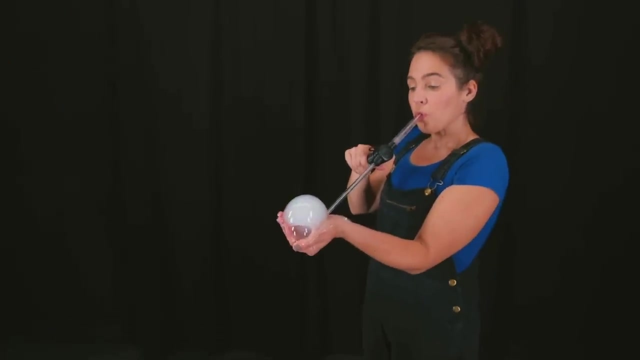 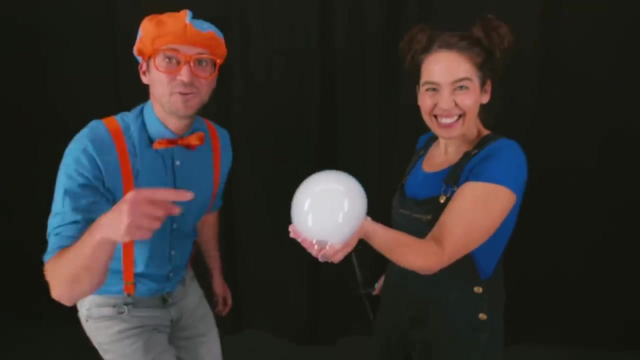 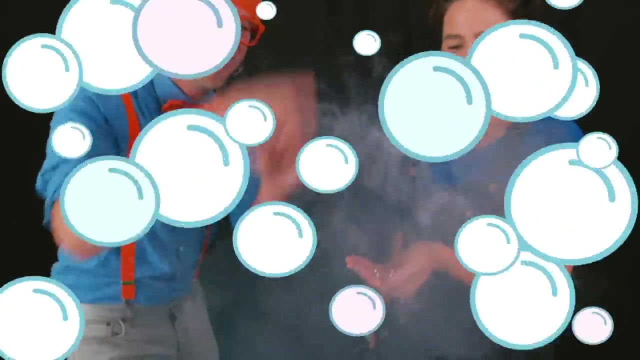 Wee, Wee, Wee, Wee, Wee, Wee, Wee, Whoa. check it out, It's a cloud bubble. Can I pop it? Of course, Here we go, Whoa, Haha, I love popping bubbles. 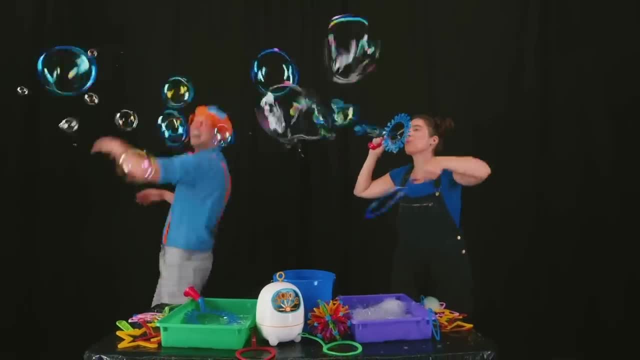 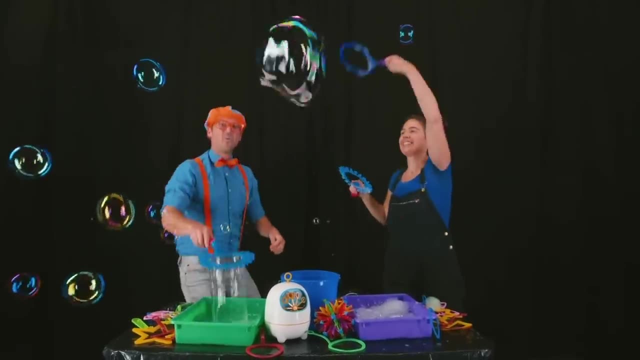 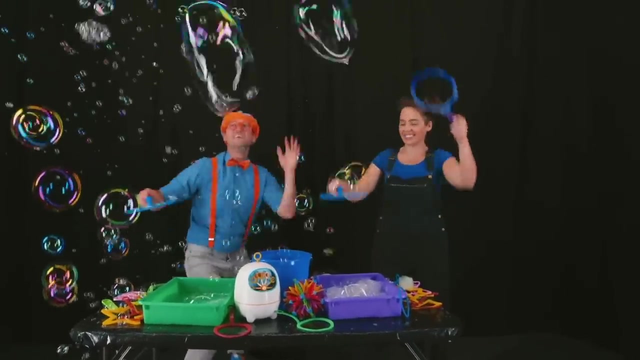 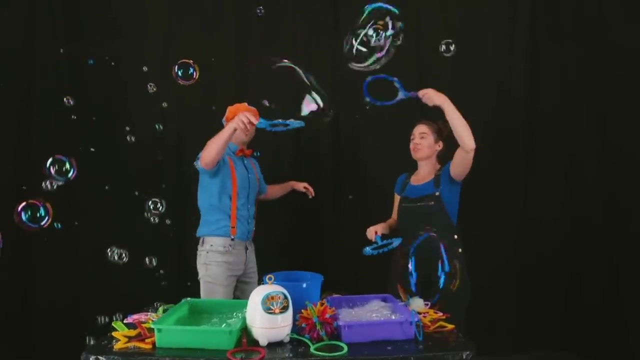 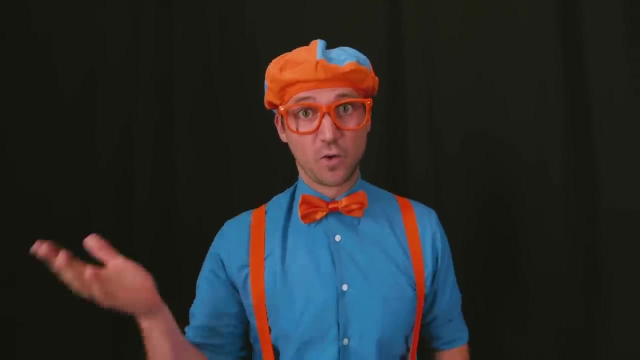 Wee, Wow, Woohoo, Yeah, Whoa, that's a big bubble, Whoa, Whoa. So we have learned a lot about bubbles today. We learned about the colors of the wand, the colors of the bubbles themselves, shapes of the. 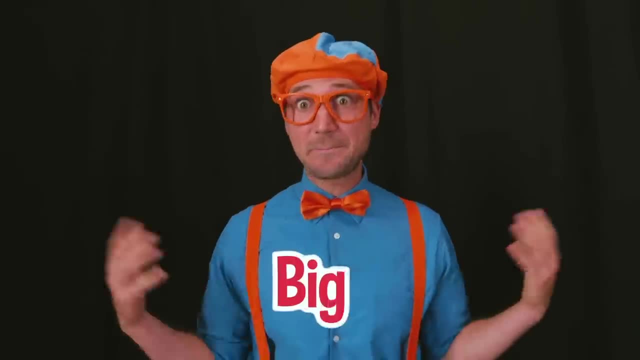 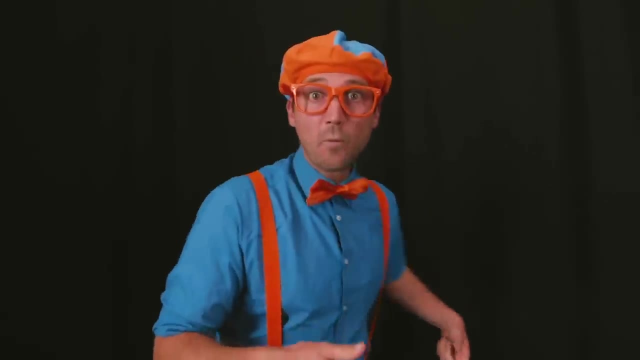 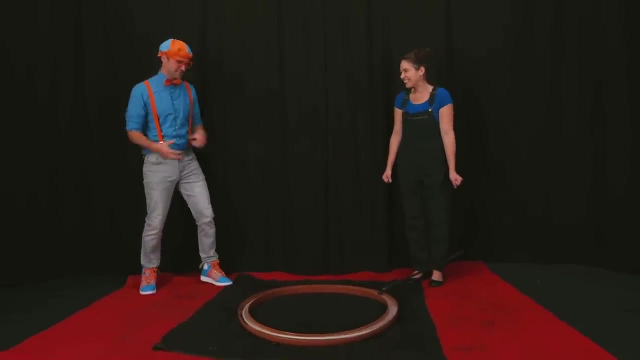 wand. We even learned about how some can be big and some can be really small, But you can't forget about those cute little insects. But what's this? Well, I have a really big bubble wand for you. I love big bubbles. What do you do? Well, it's. 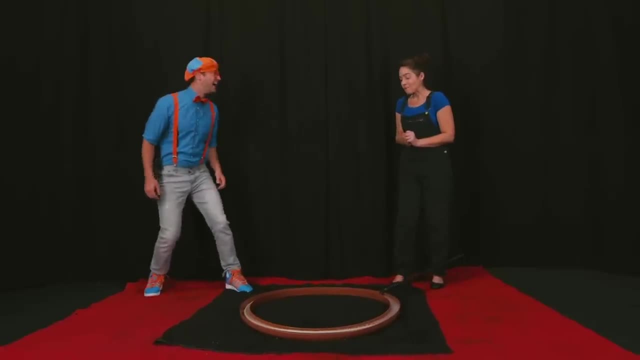 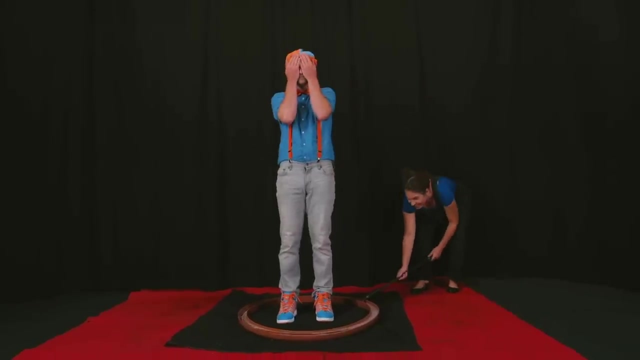 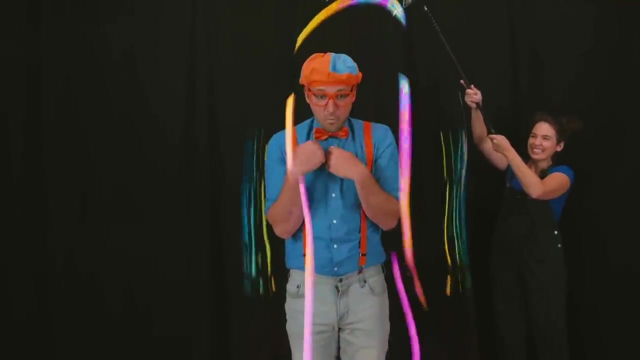 a surprise. Okay, I love surprises, But first I need you to step right in the middle of it. Okay, Now close your eyes. Alright, Now open them. Whoa, Look at it, I'm inside a bubble. Whoa, This is awesome. 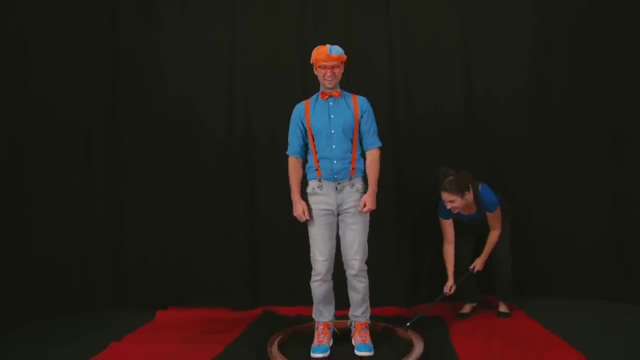 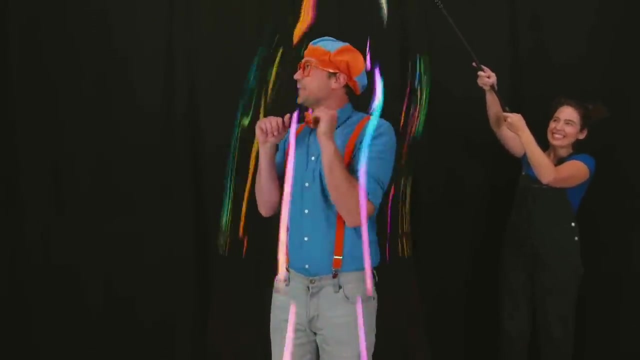 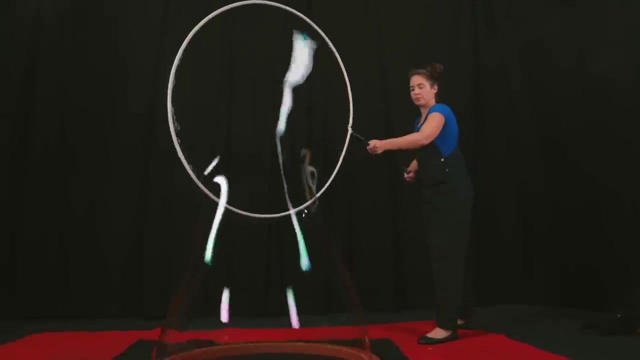 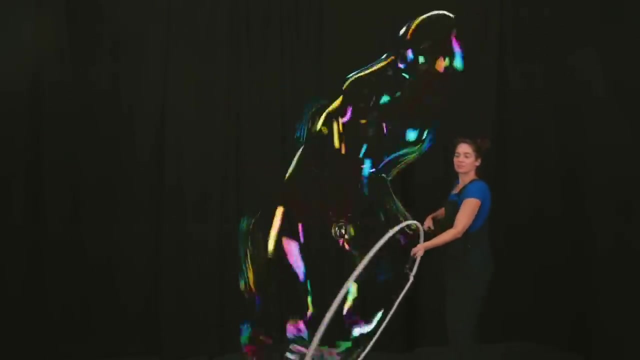 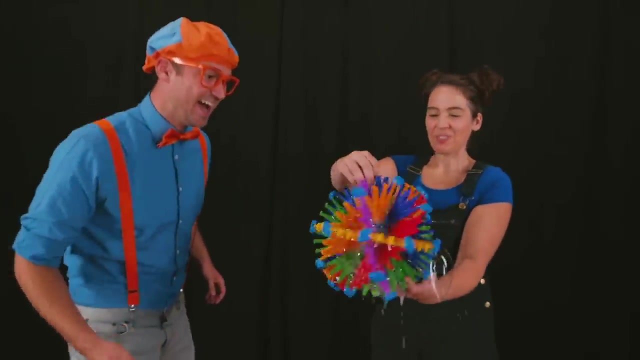 Can we do that again, please, Of course. Alright, Here we go. Whoa, I'm swimming in a bubble. Whee, Yeah, Wow, What is that? Well, this is the rainbow ball. Wow, A rainbow ball. Let's see.